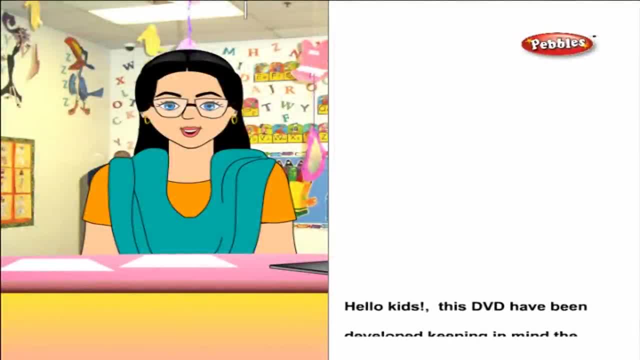 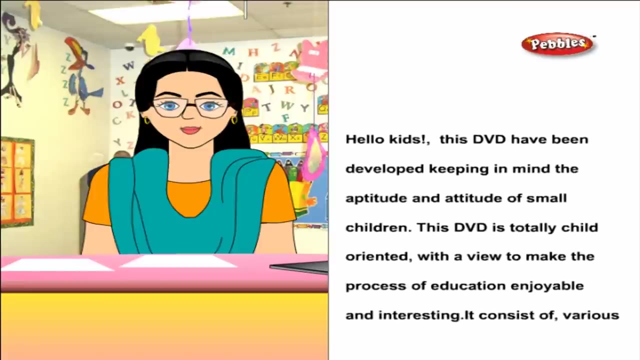 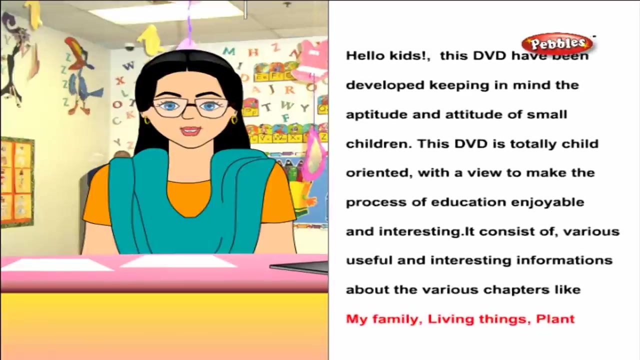 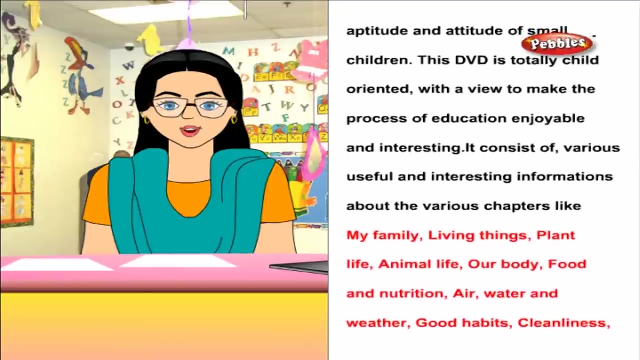 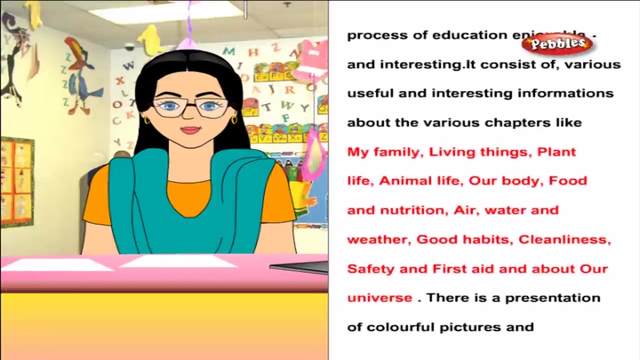 Hello kids. This DVD has been developed keeping in mind the aptitude and attitude of small children. This DVD is totally child-oriented with a view to make the process of education enjoyable and interesting. It consists of various useful and interesting informations about various chapters like My Family, Living Things, Plant Life, Animal Life, Our Body. 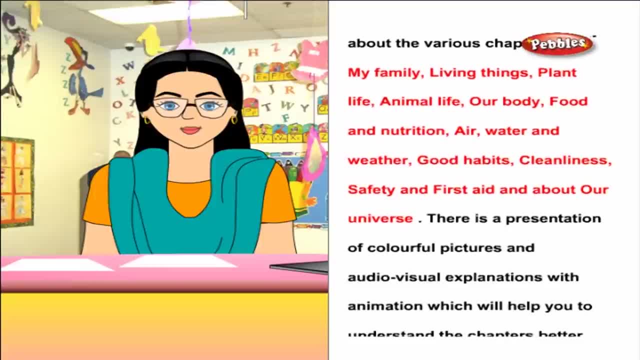 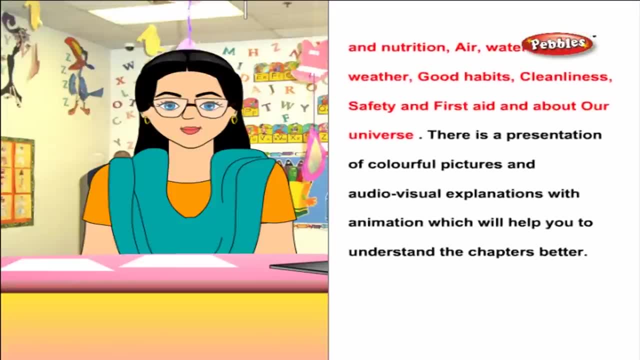 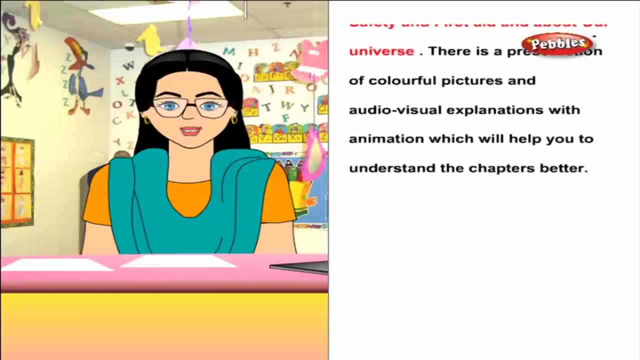 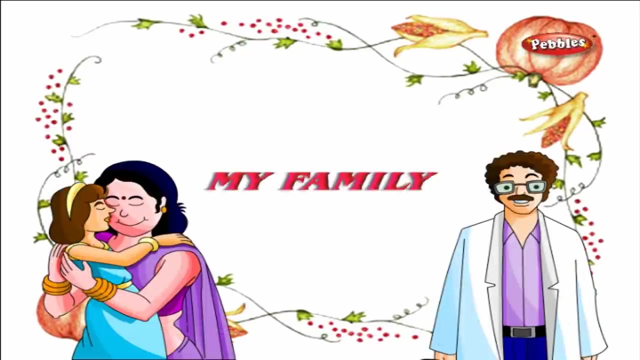 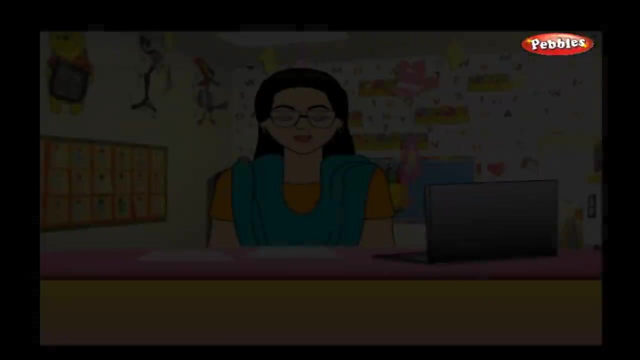 Food and Nutrition, Air, Water and Weather, Good Habits, Cleanliness, Safety and First Aid, and About Our Life. There is a presentation of colourful pictures and audio visual explanations with animation, which will help you to understand the chapters better. Hello kids, This DVD has been developed keeping in mind the aptitude and attitude of small 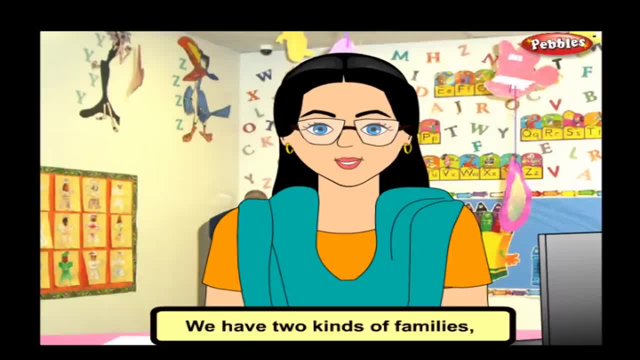 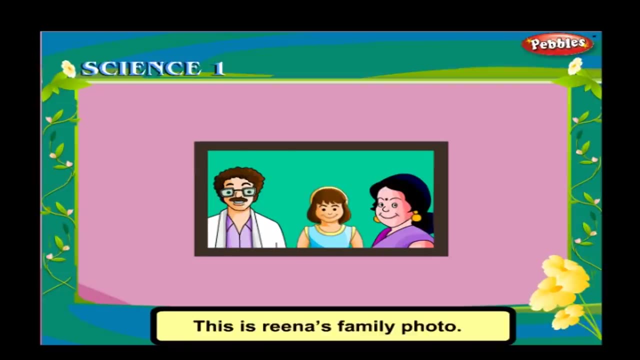 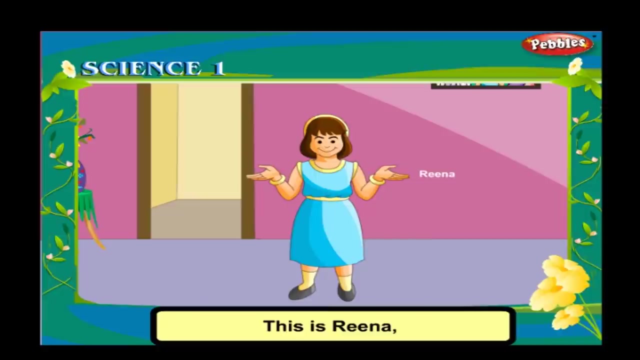 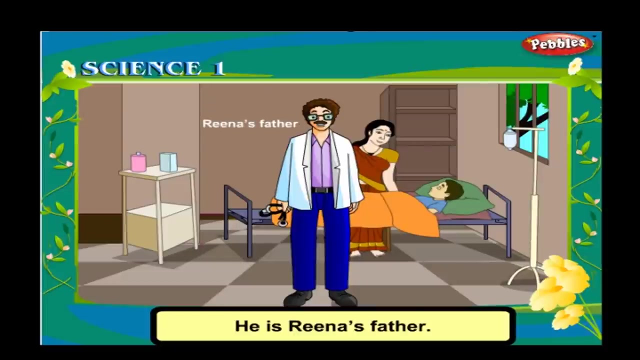 children. This DVD is totally child-oriented with a view to make the process of education family. we have two kinds of families: small family and a big family. let us first see what a small family is. this is Reena's family photo. let me introduce them one by one. this is Reena. she is eight years old. he is Reena's father, his. 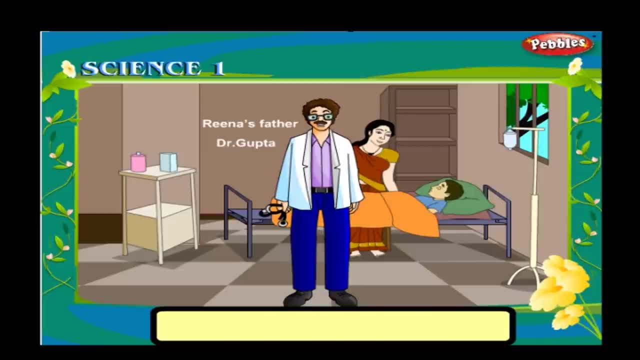 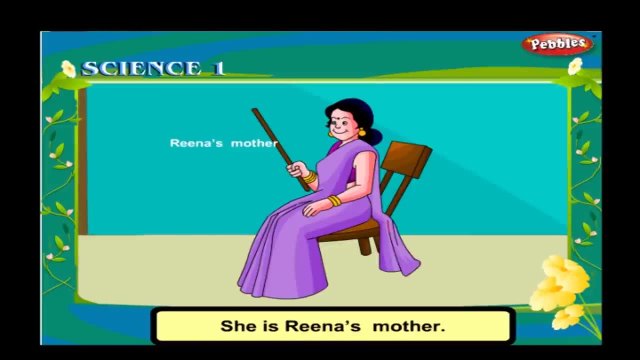 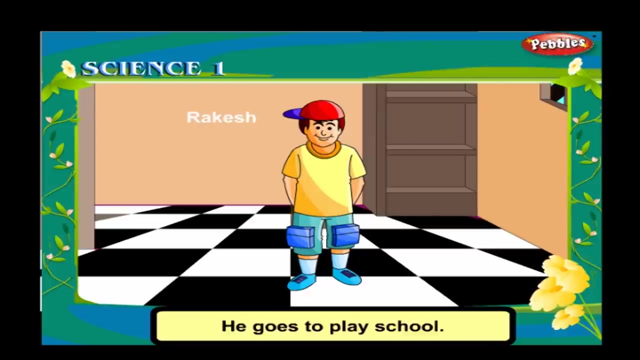 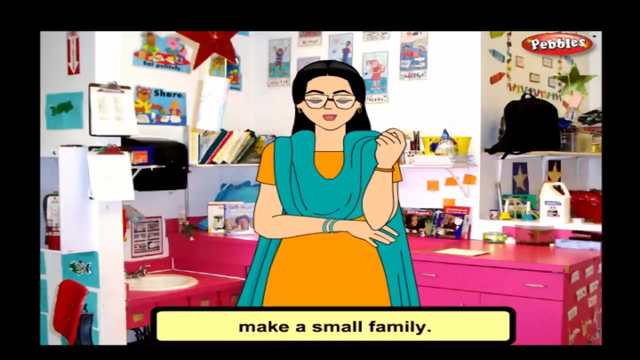 name is dr Gupta. he is working as a doctor in a hospital. she is Reena's mother. her name is Meera. she is working as a teacher in a school. meet her little brother, Rakesh. he goes to play school. father, mother, one or two children make a small family. see this photograph. this is a big 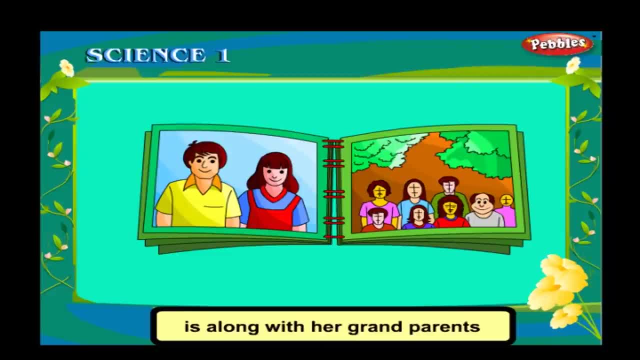 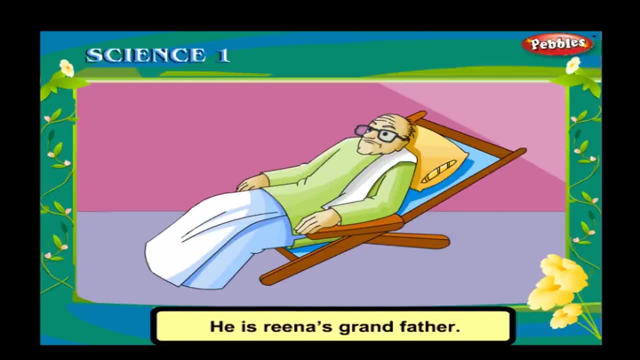 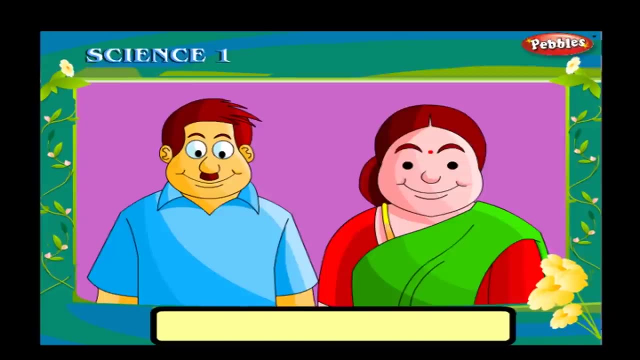 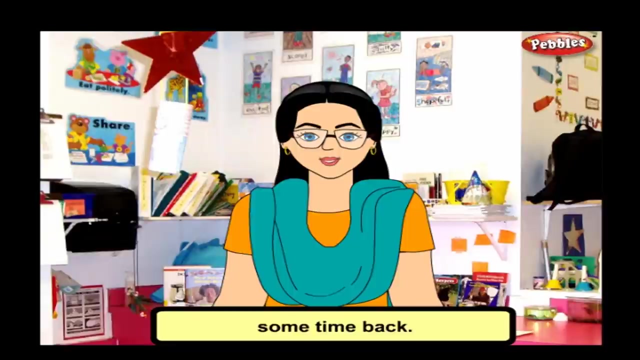 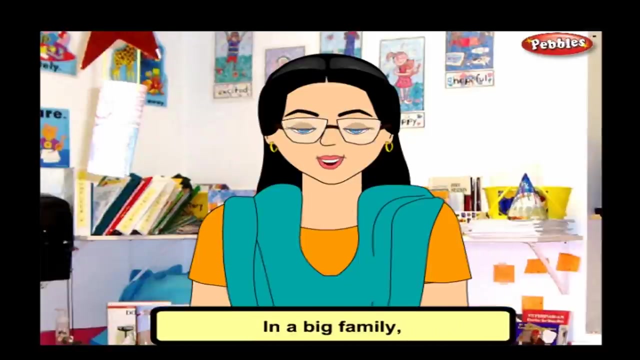 family. Reena is along with her grandparents and cousins. he is Reena's grandfather, she is her grandmother, he is her uncle and she is her auntie. they all were living together sometime back. when you live with your grandparents and cousins, it is called a big family. in a big family, we love each other, we help each. 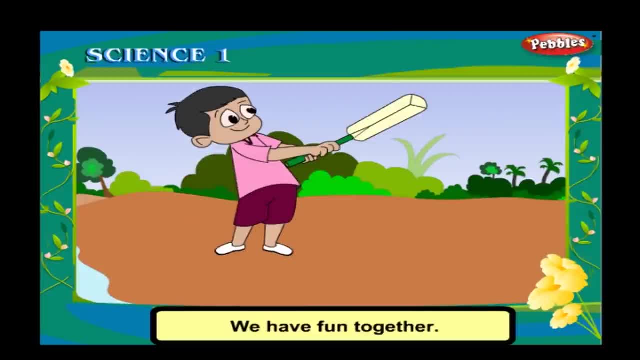 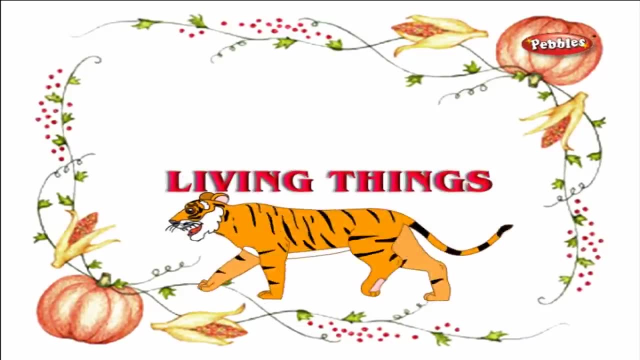 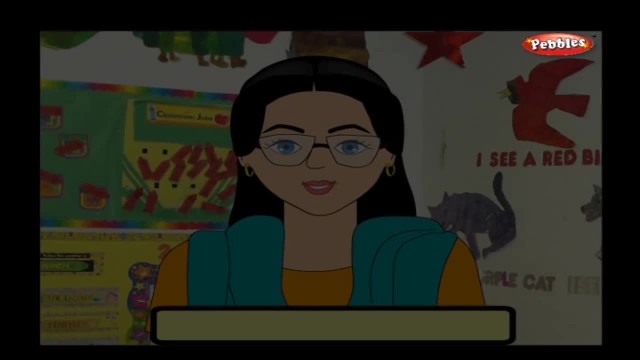 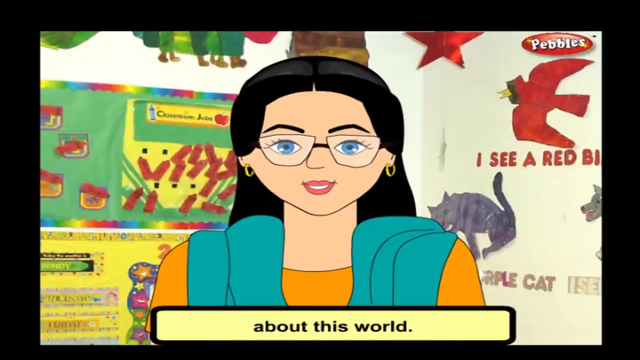 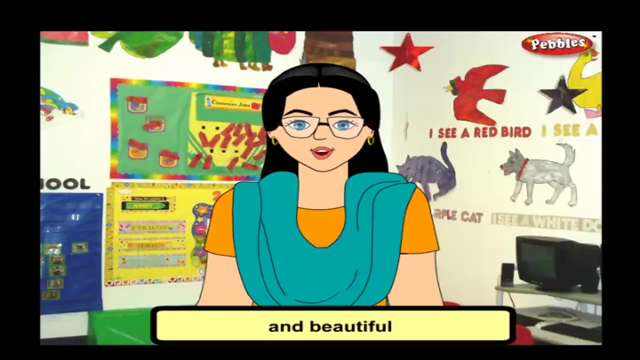 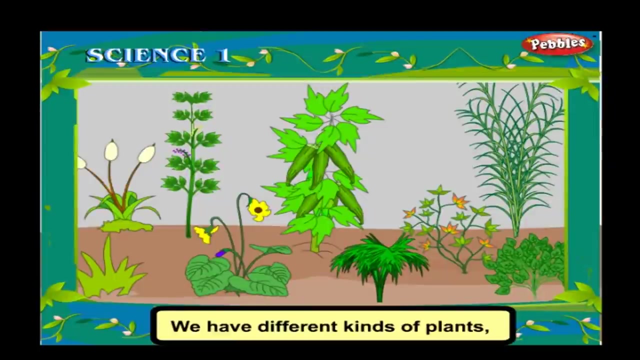 other. We have fun together. We all live very happy. Apart from our family, there are many more things that we should know about this world. This world where we live is wonderful and beautiful with various kinds of things, isn't it? We have different kinds of plants, different kinds of animals and birds around us. 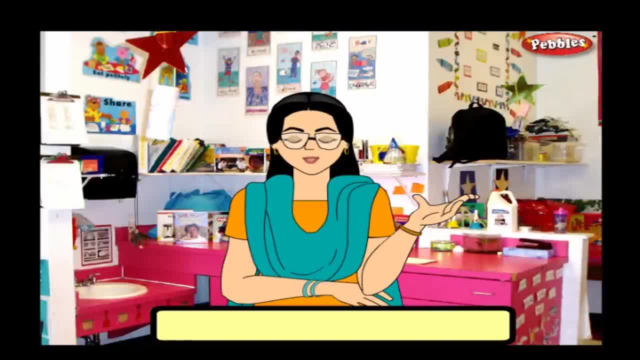 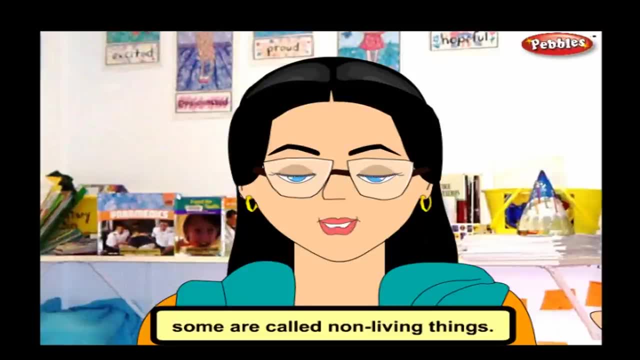 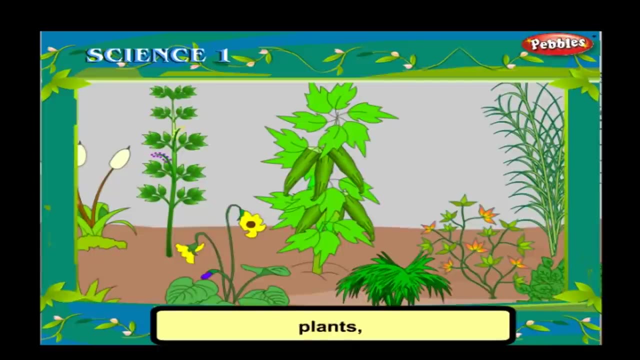 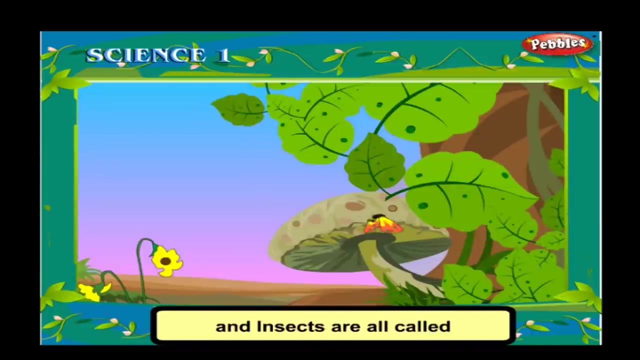 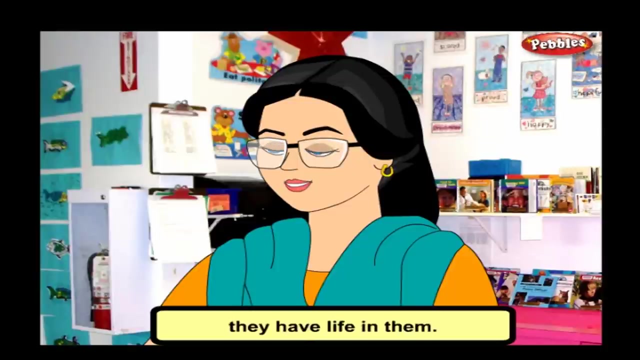 This makes the world wonderful. Some of the things around us are called living things and some are called animals, Non-living things. human beings, trees, plants, birds, animals and insects are all called living things. They are called living things because they have life in them. 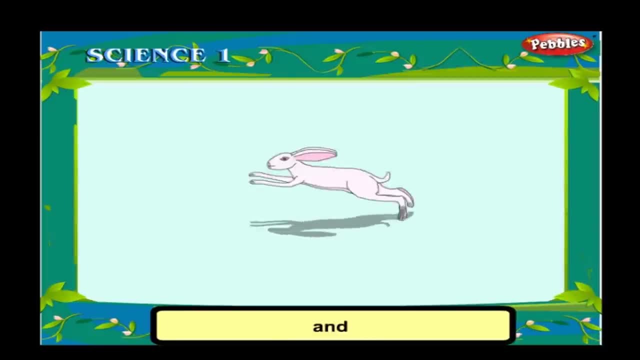 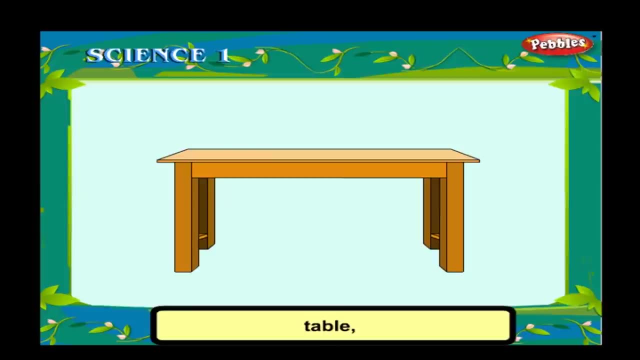 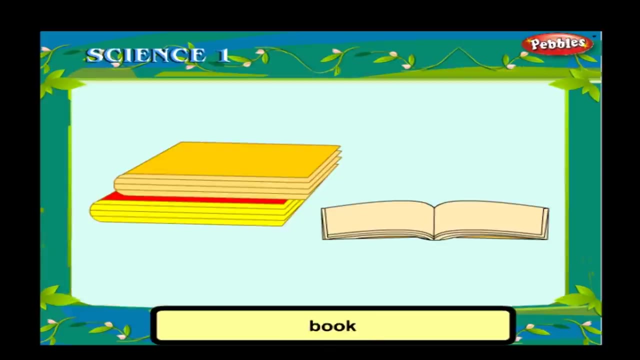 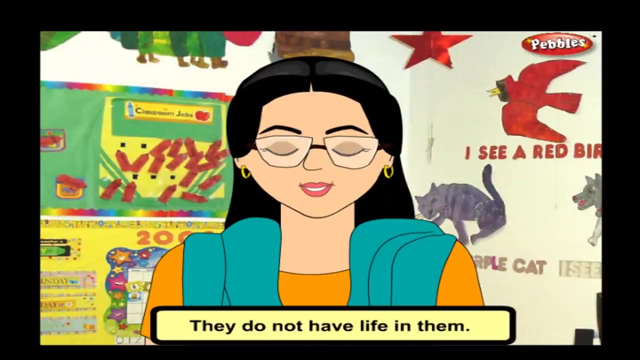 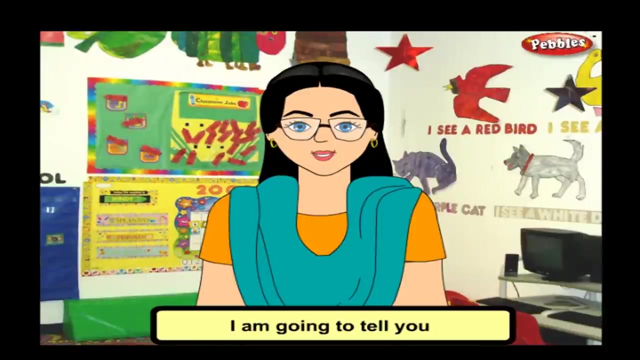 They grow, they move and they also die. Some other things like the chair, table, car, buildings, book and ball are called non-living things. They do not have life in them, They cannot grow or move. Now I am going to tell you about the special features of living things. 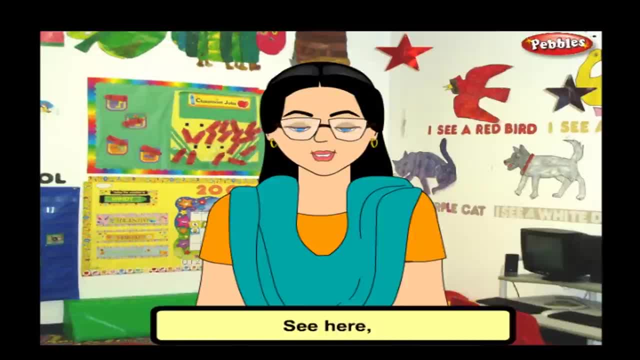 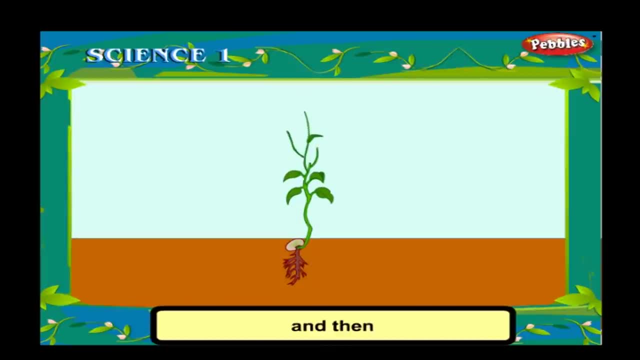 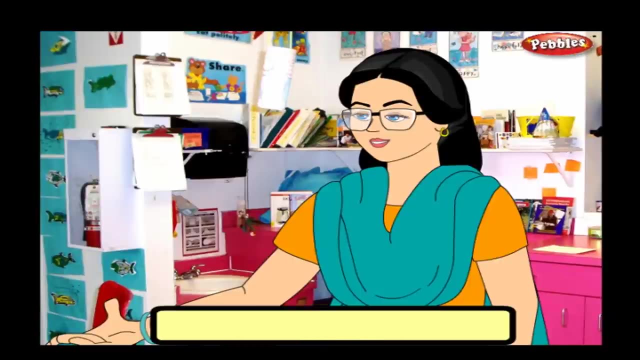 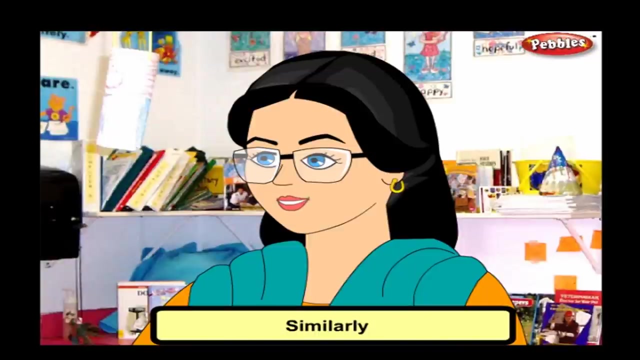 Living things can grow. See here: A seed grows into a small plant and then into a big plant. You can watch the plants in your garden. A small plant in your garden grows into a big plant. Similarly, an egg hatches into a chick. 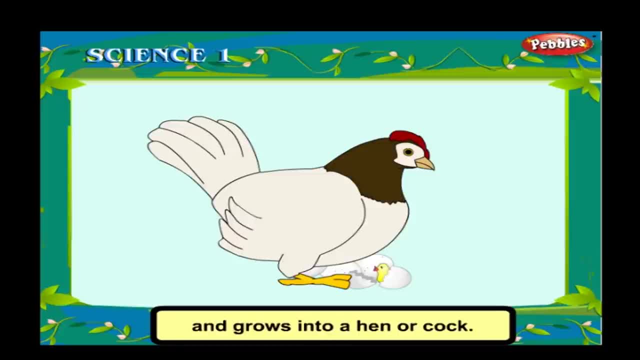 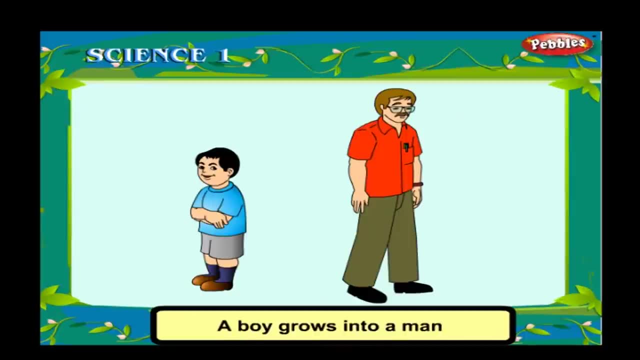 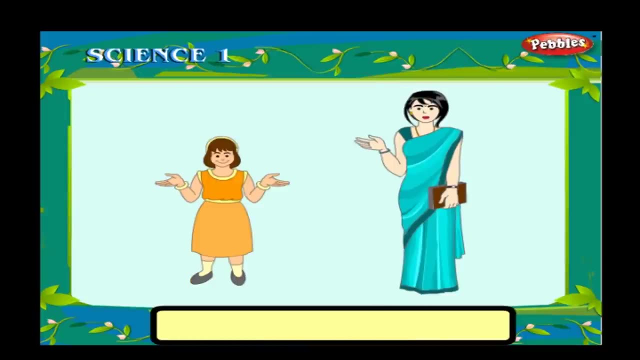 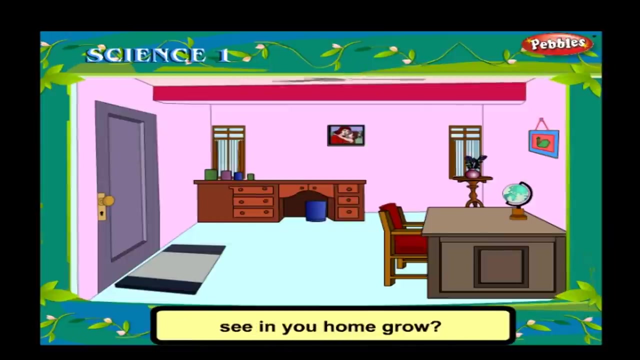 A chick comes out of an egg and grows into a hen or a cock. A baby grows into a boy or a girl. A boy grows into a man and a girl grows into a woman. All living things grow. Does a non-living thing, like the chair or a table which you see in your home, grow? 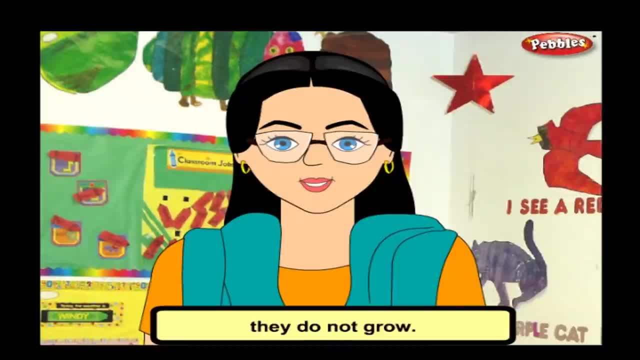 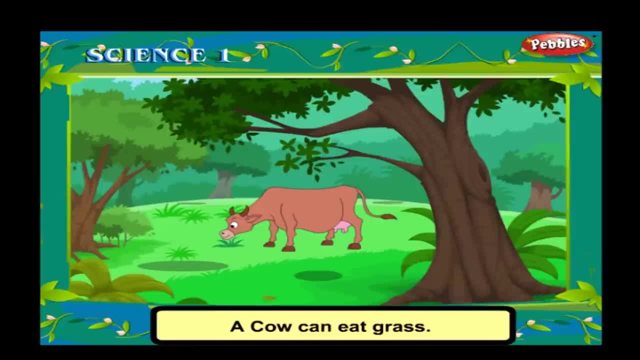 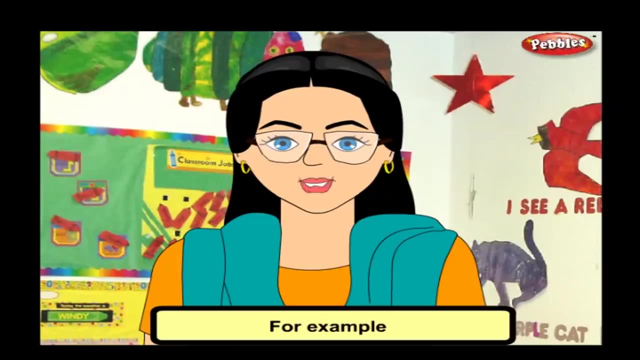 No, they do not grow. They do not grow. They do not grow. Living things can eat. A hen can eat grains, A cow can eat grass, Man can eat food. For example, take a bird and a stone and keep them both on the floor. 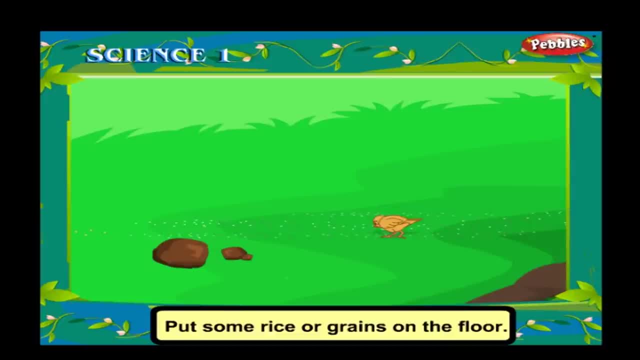 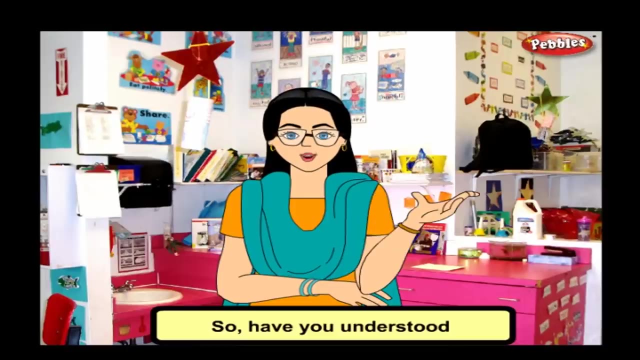 Put some rice or grains on the floor. Watch them. Now tell me who is eating the rice. Yes, a bird can eat rice. A cow can only eat The stone will not eat the rice. So have you understood that only a living thing can eat food? 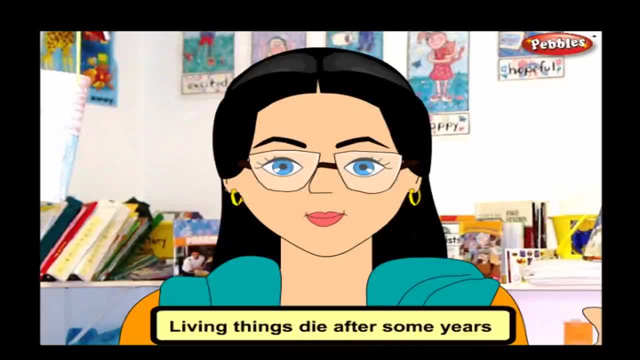 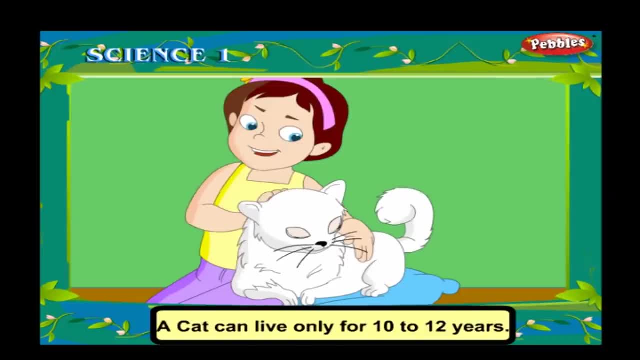 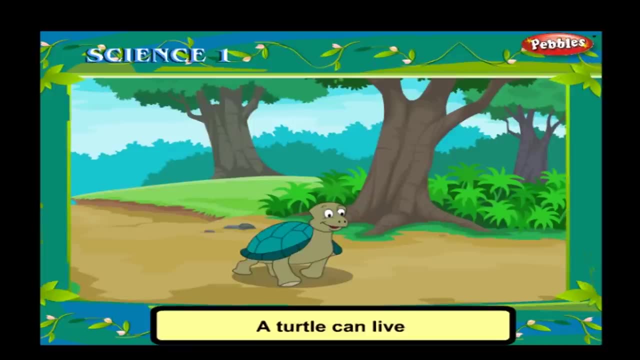 The food helps the living things to grow. Living things die after some years, after they grow old. A cat can live only for 10 to 12 years. A dog can live only for 20 years. A turtle can live for more than 50 years. 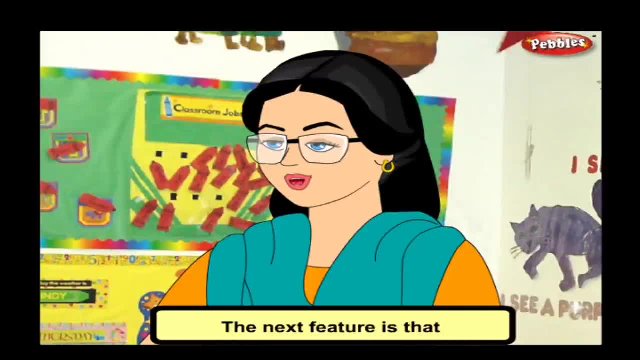 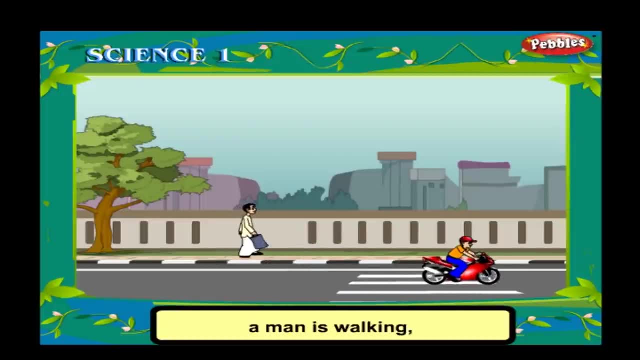 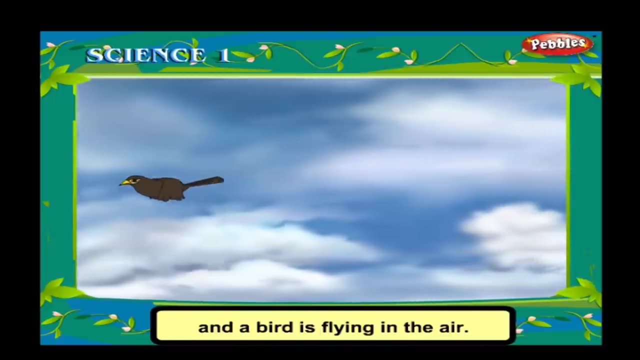 Non-living things do not die. The next feature is that living things can move. See, here a man is walking, a fish is swimming in the water and a bird is flying in the air. Does a chair or a book or a stone move from one place to another? 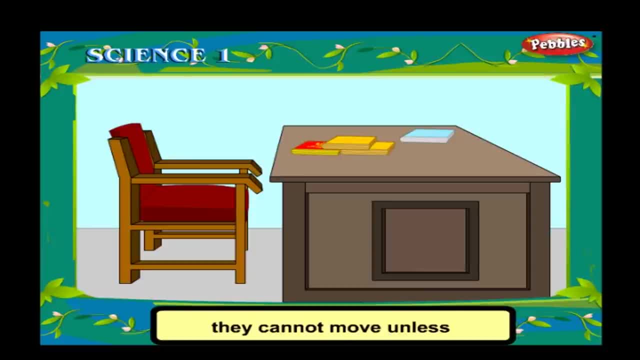 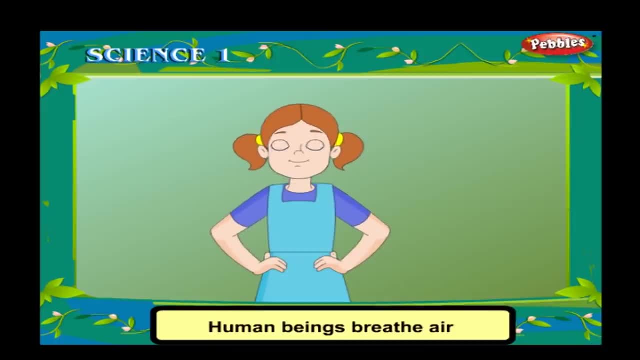 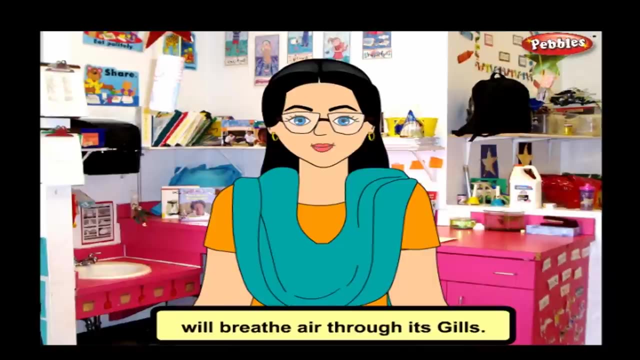 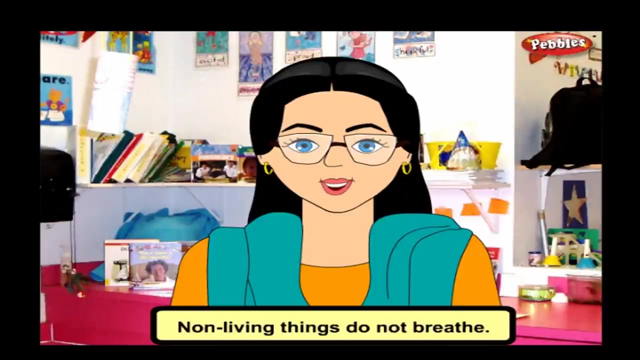 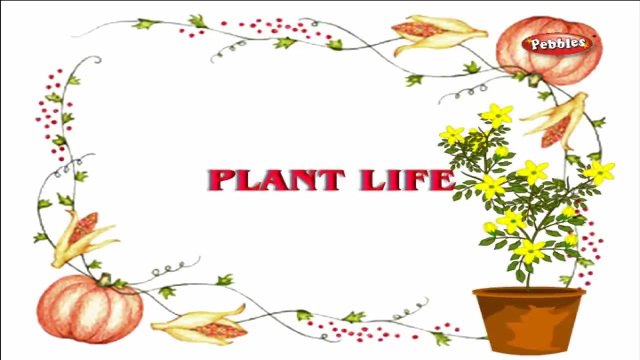 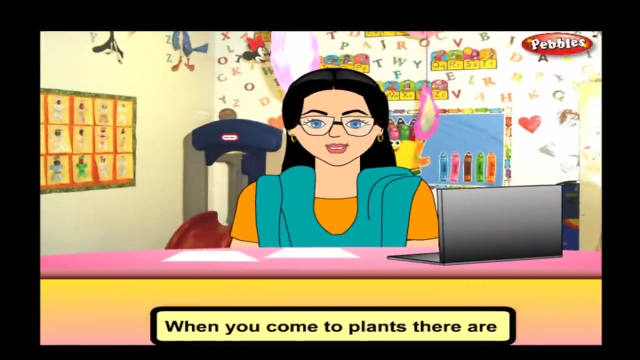 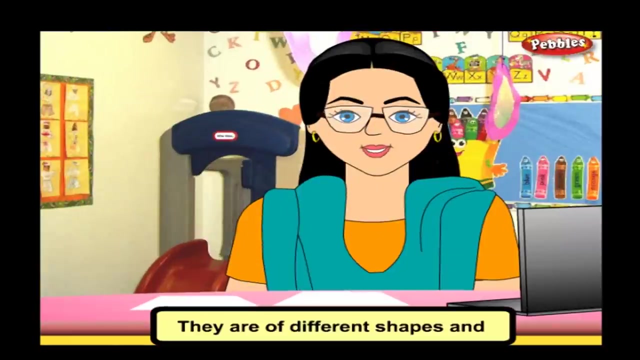 No, They cannot move unless you move them. Living things can breathe. Human beings breathe air through their nose. A fish will breathe air through its gills. Living things cannot live without air. Non-living things do not breathe. when you come to plants, there are variety of plants in this world. they are of different shapes. 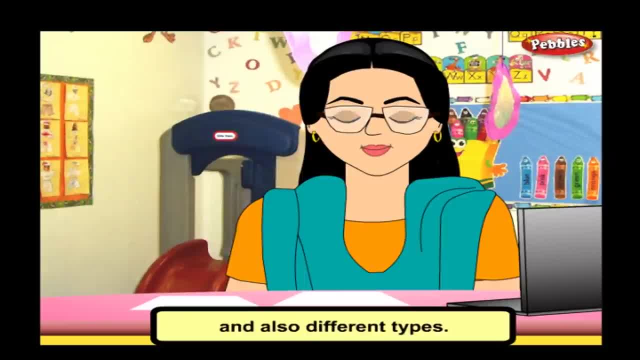 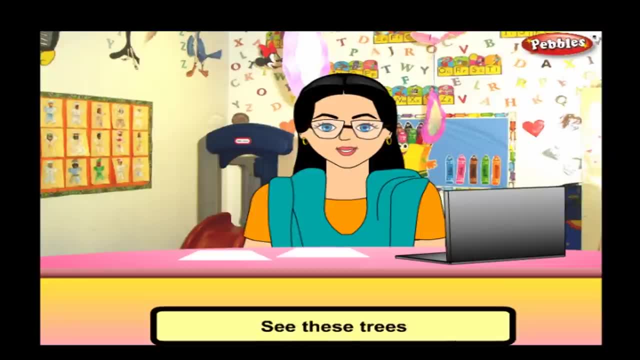 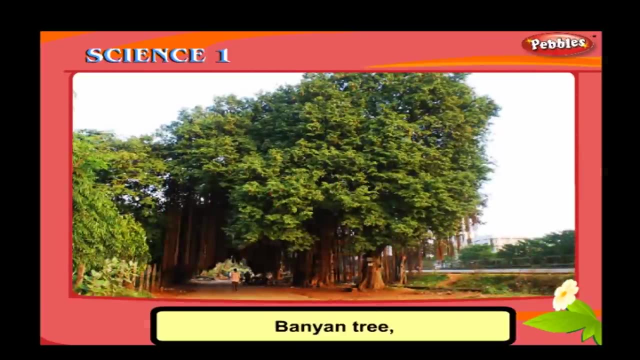 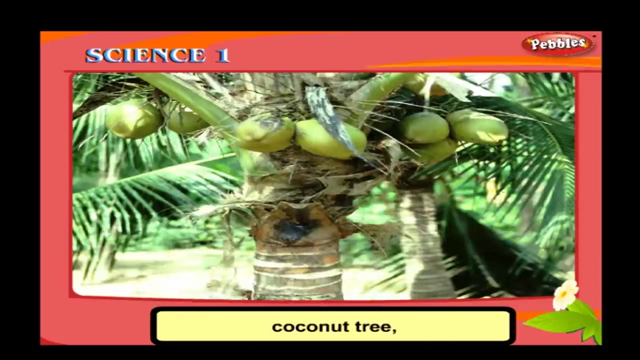 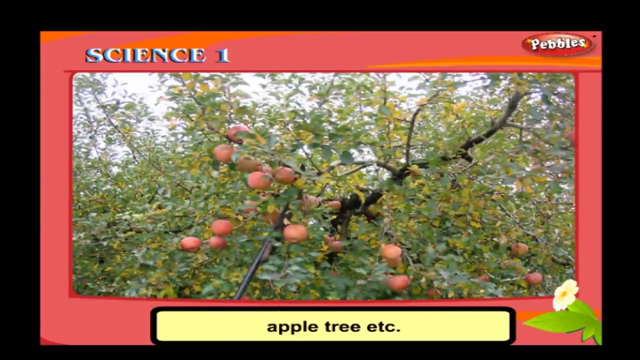 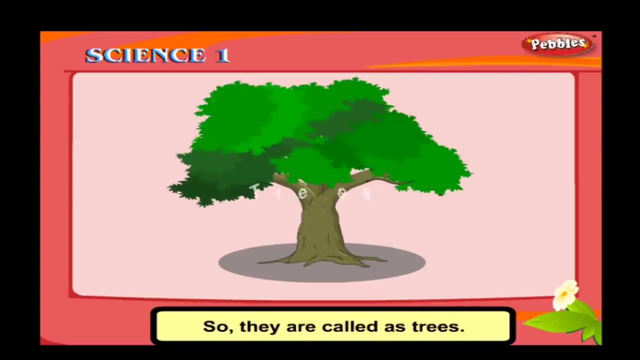 and sizes and also different types. some plants are big and some plants are small. see these trees: Ashoka tree, banyan tree, mango tree, neem tree, coconut tree, gulmoha tree, apple tree, etc. these plants grow big and strong, so they are called as trees now. we will see about plants which are small. see these plants: rose plant, sunflower plant, hibiscus plant and cotton plant. these plants are small plants. they grow to a small height and their stems are not very strong. these are called shrubs. some plants, like the mint and basil, are very small and weak. these are called 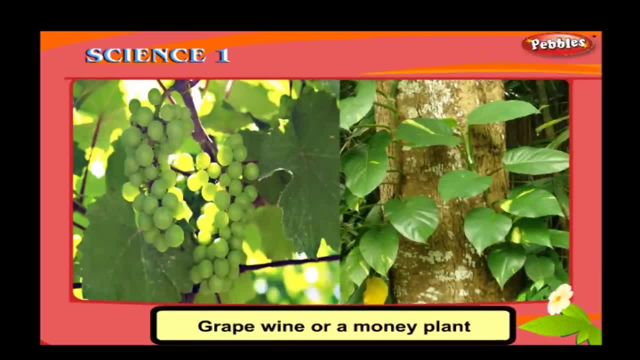 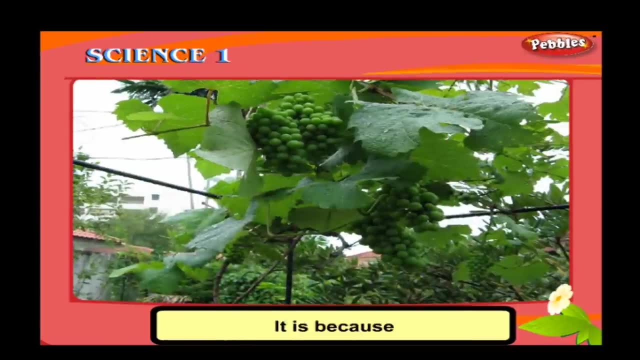 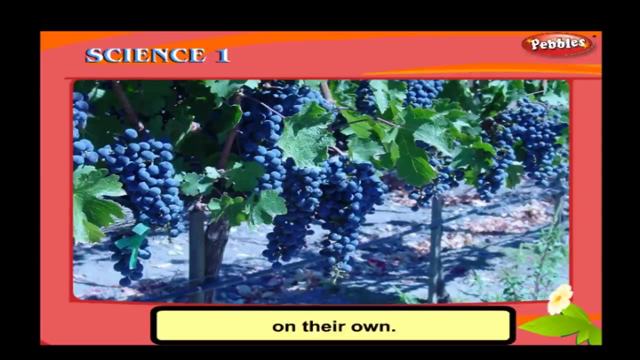 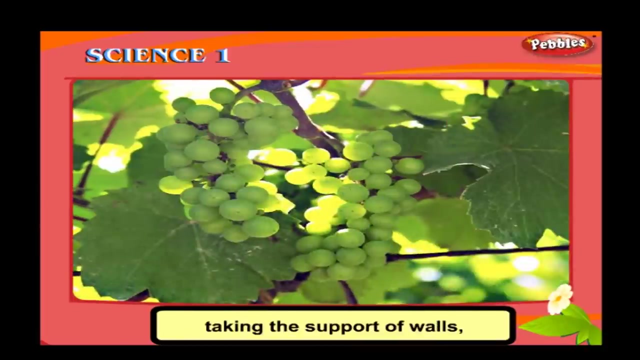 herbs, grapevine or a money plant do not grow as the other plants. do you know why? it is because these plants are weak and cannot grow straight on their own, so they need a love to grow. these plants climbed up, taking the support of bullets or other plants or sticks. these are called climbers. a pumpkin plant grows along the 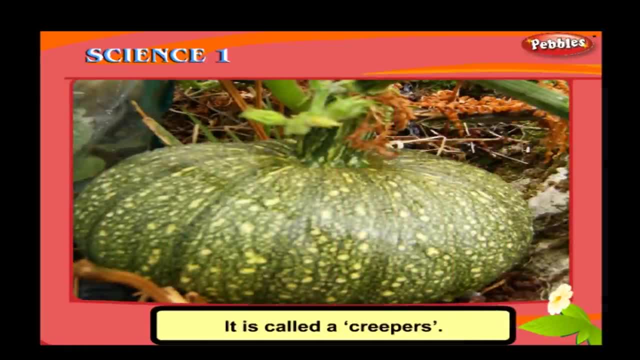 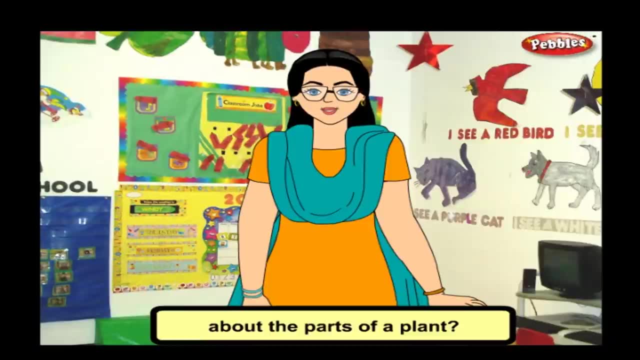 ground. it is called a creepy. now let us learn about the paths of a plant. flowers is just like Whelan plant or platypus plant: very small� as a plant flower is. the most powerful flower can have nine leaves. all its roots would be more than 20 or 30. toddlies are more th than 10 και as a gram seeds than and a kill a fast flower man'. 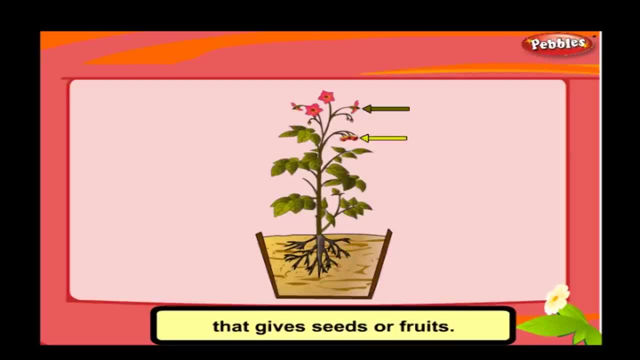 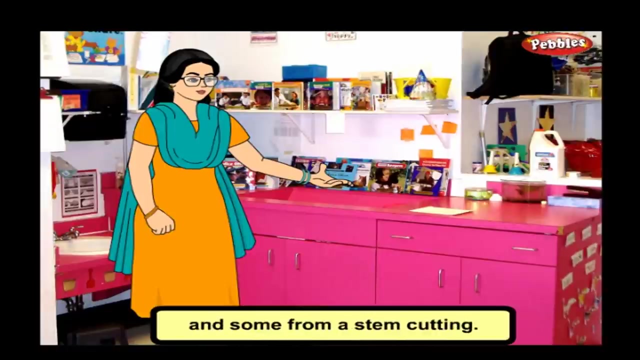 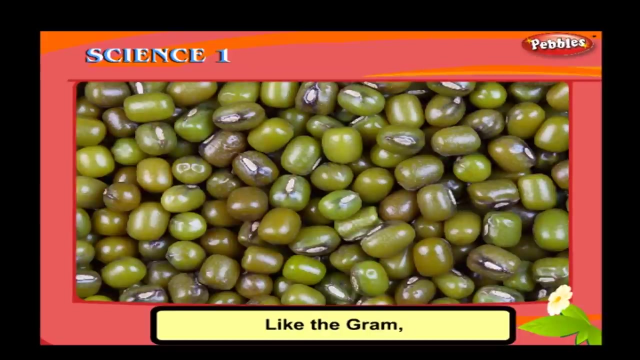 the beautiful part that gives seeds or fruits leaf, makes food for the plant stem, carries food and water to all parts of the plant root, gives support and takes water and nutrients from the soil. most plants grow from seeds and some from a stem cutting. there are different kinds of seeds, like the gram bean pea. 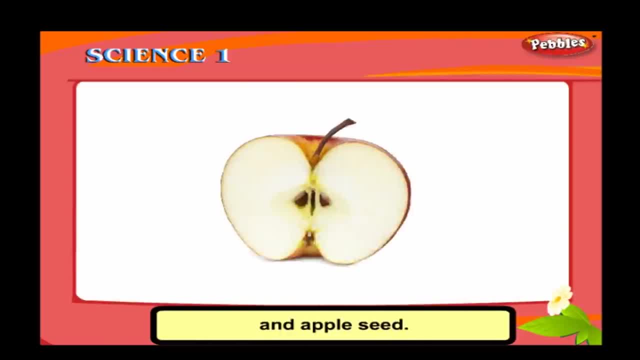 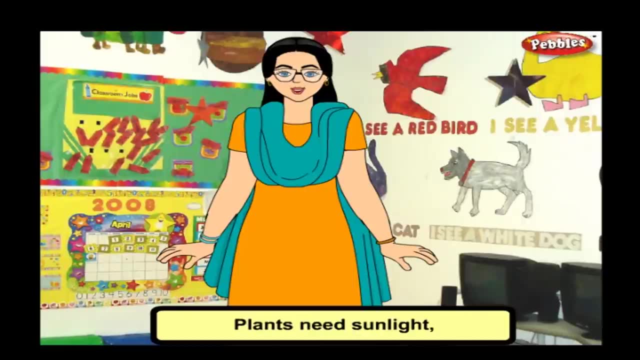 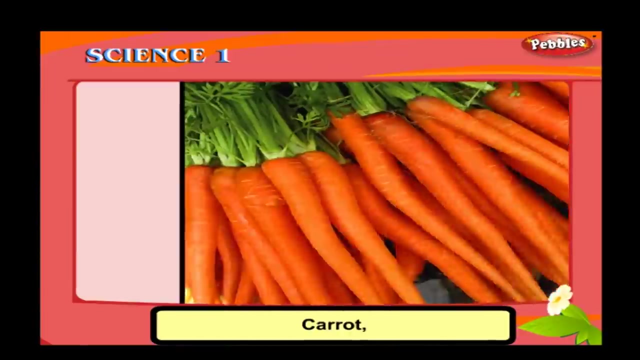 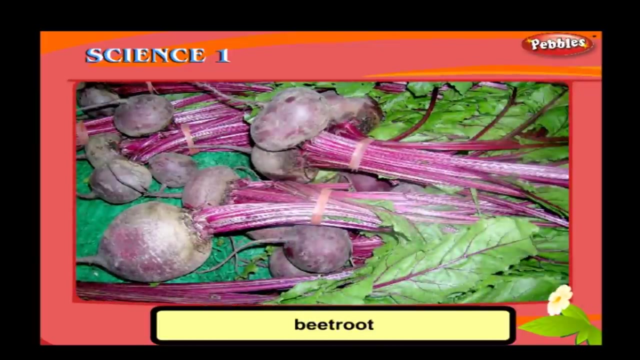 corn and apple seed. a seed has a baby plant inside it. plants need sunlight, air and water to grow. it also needs soil from which the roots take nutrients. most of our food comes from plants. we eat almost all the parts of a plant: carrot, radish, beetroot and 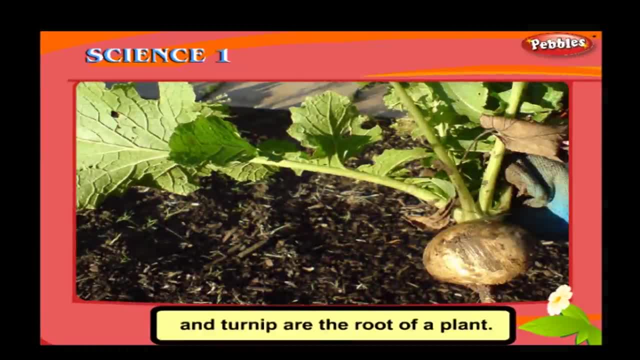 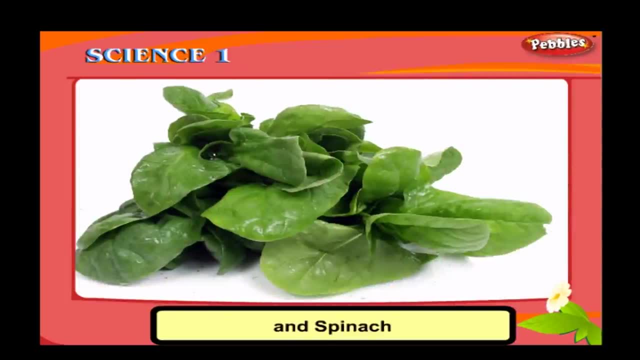 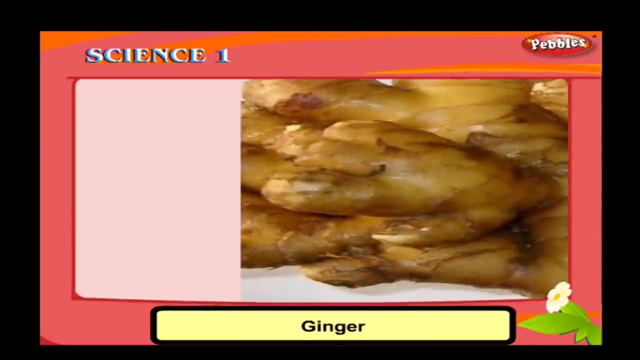 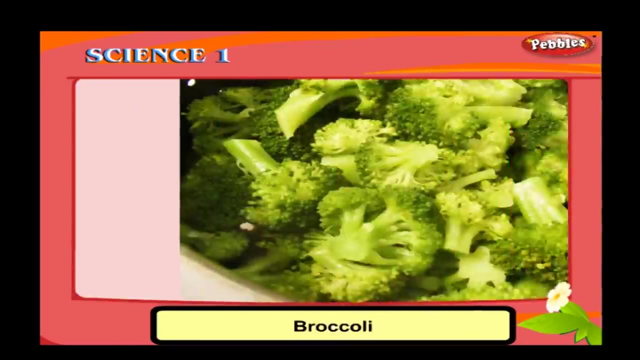 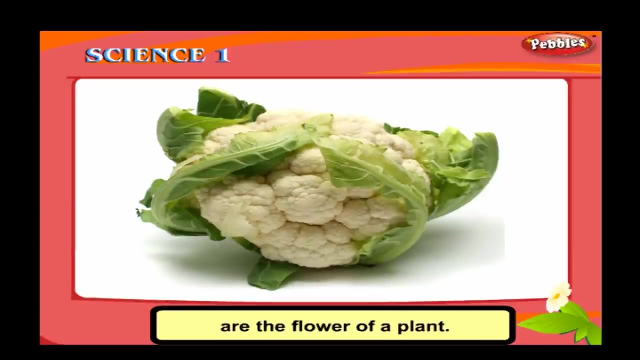 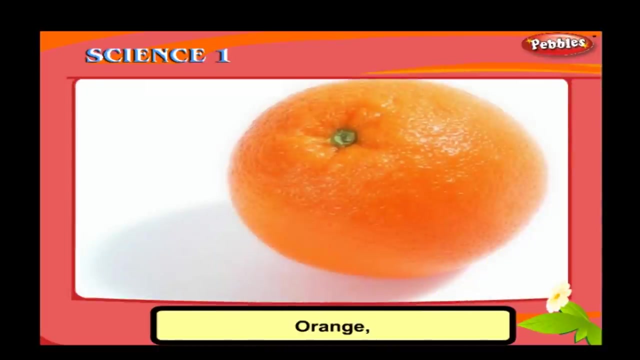 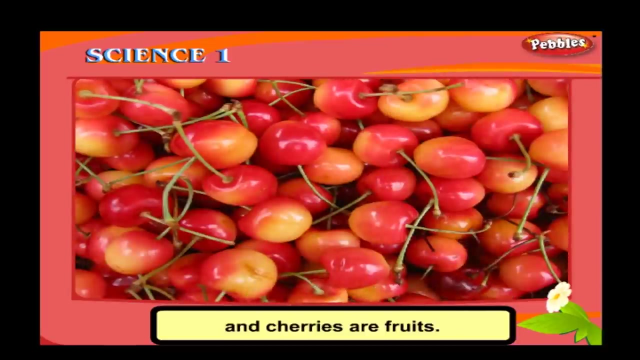 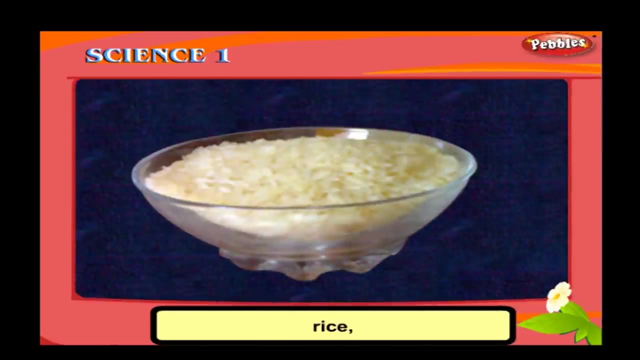 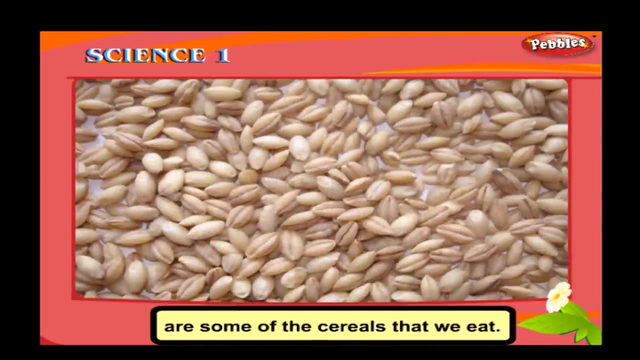 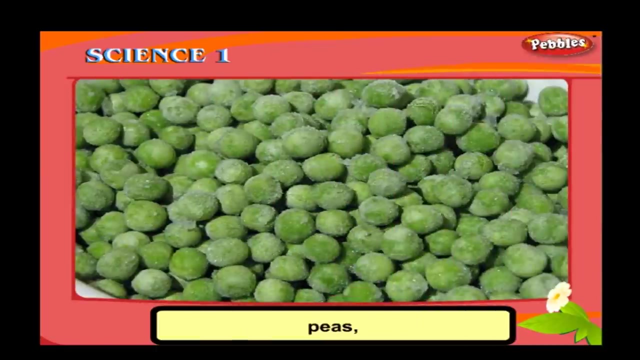 turnip are the roots of a plant. cabbage, lettuce and spinach are leaves of a plant. potato, ginger and sugarcane are the stem. broccoli and cauliflower are the flower of a plant. apple, grapes, orange, mango, banana and cherries are fruits. wheat, rice, maize and barley are some of the cereals that we eat: gram peas, beans and kidney. 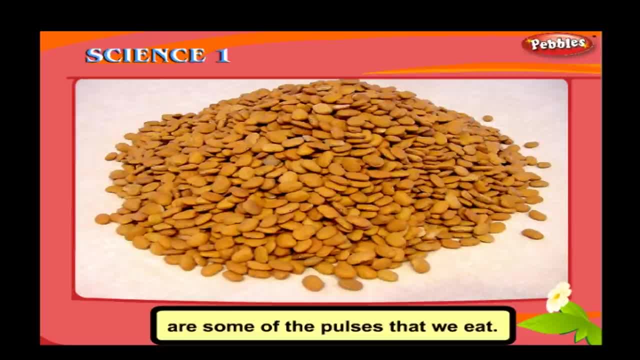 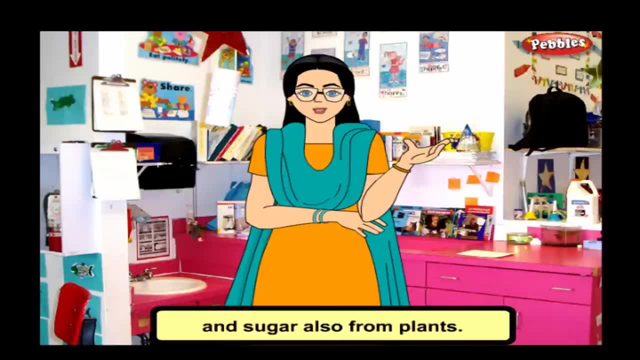 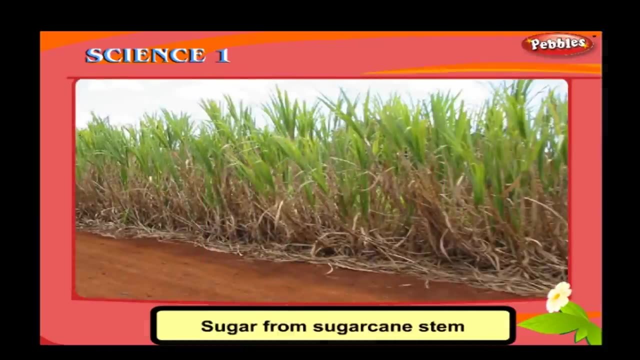 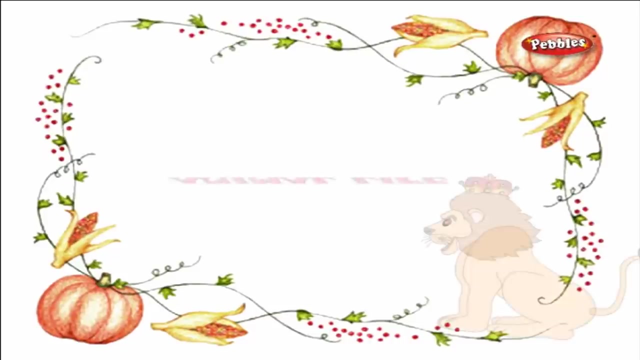 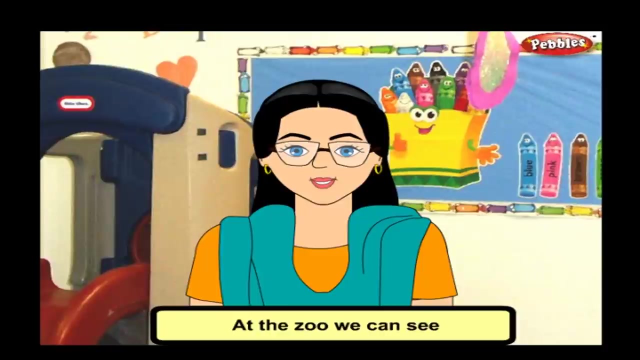 beans are some of the pulses that we eat. we get coffee, tea and sugar also from plants: coffee from coffee seeds, sugar from sugarcane stem and tea from tea leaves. have you all been to a zoo? at the zoo, we can see lots of animals. at the zoo, we can see lots of animals. 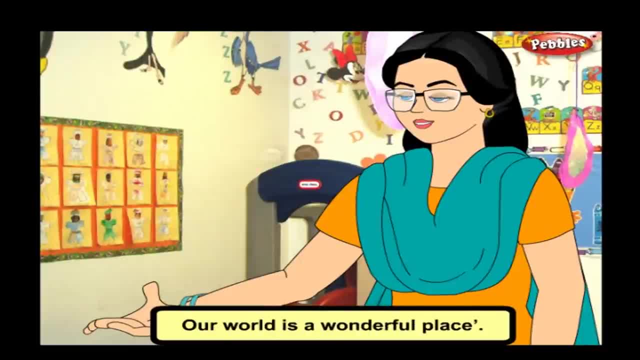 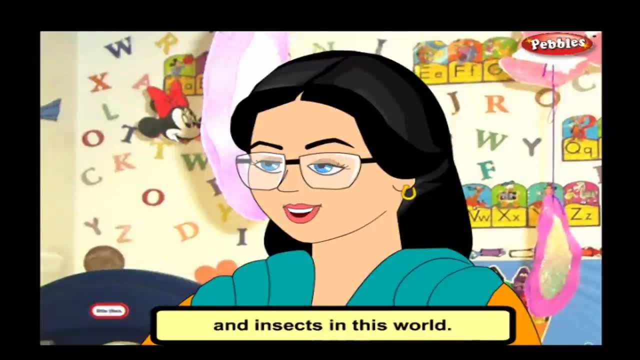 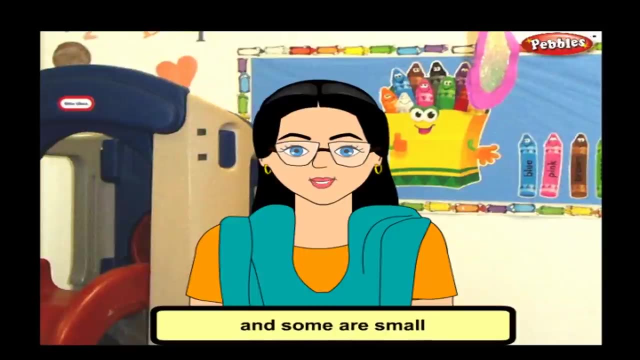 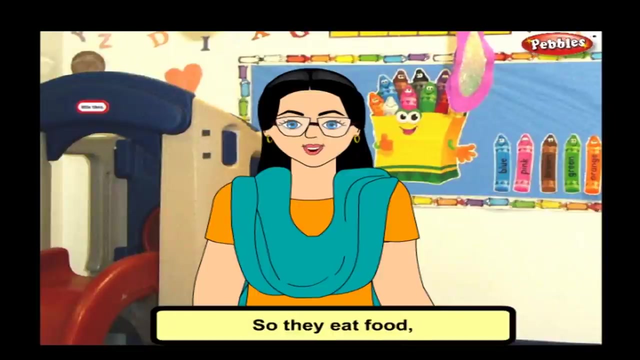 at the zoo we can see lots of animals and birds. our world is a wonderful place. there are different kinds of animals, birds and insects in this world. some animals are big and some are small. animals and birds are living things, so they eat food, grow in size, move from. 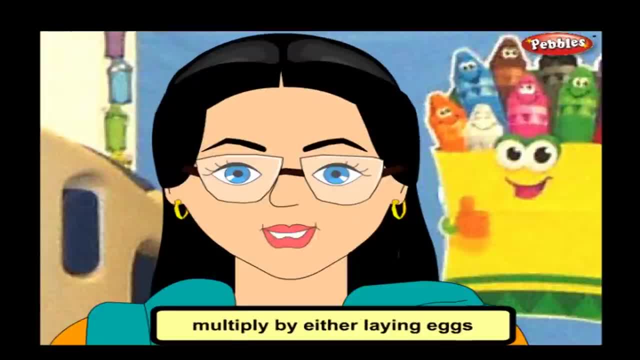 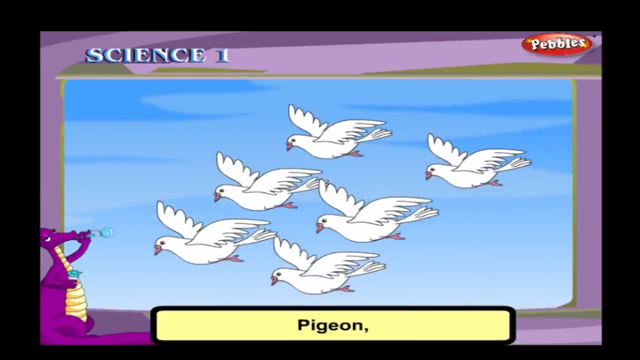 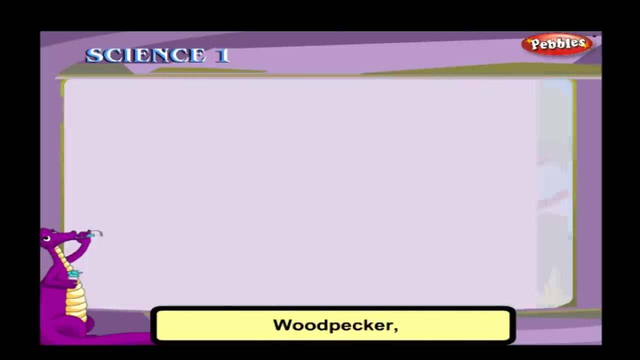 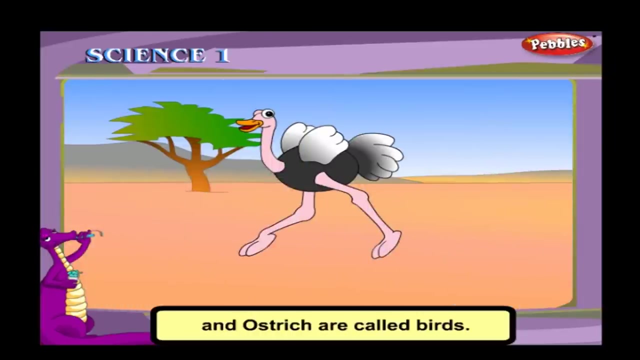 animals move from one place to another for food. x by either playing, hey multiply, by either laying or by giving birth to young once. parrot, crow, pigeon, oh wood becomes penguin kewy, oh wood becomes penguin kewy, ostrich are all called birds. these birds have two legs, which help them to walk. 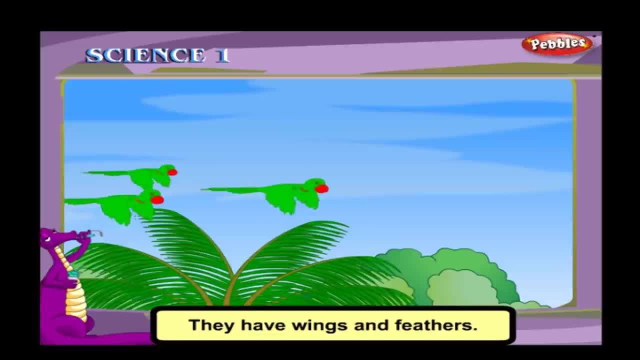 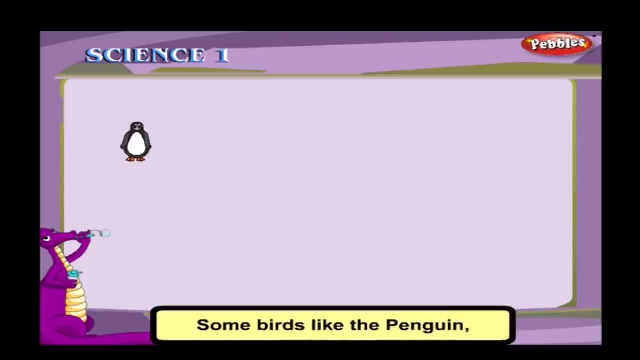 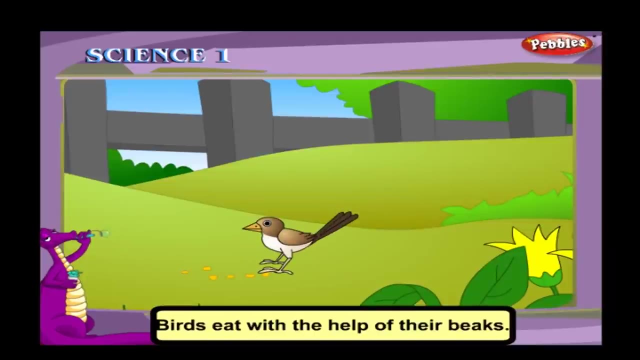 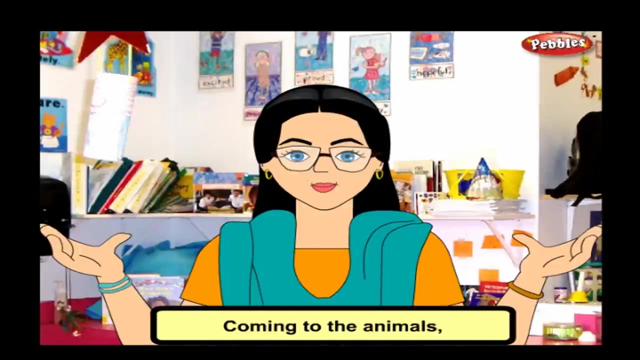 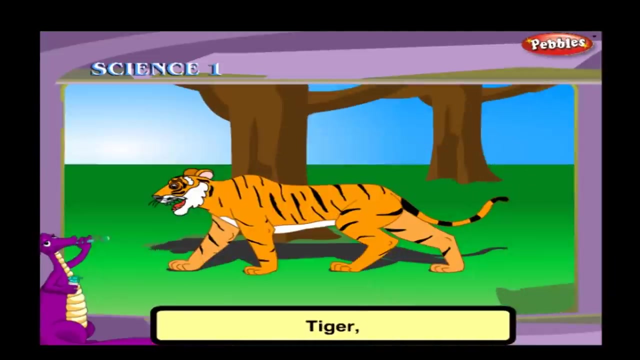 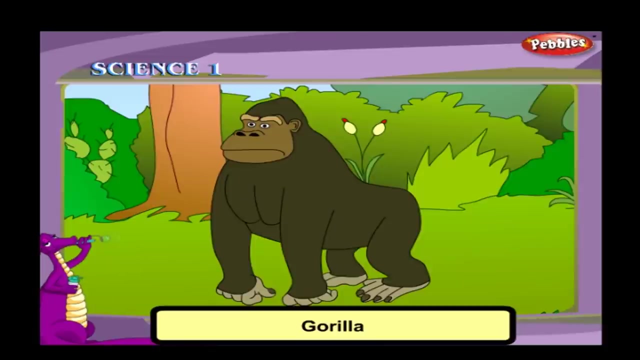 they have wings and feathers. wings help them to fly. most birds can fly. some birds, like the penguin, kiwi and ostrich, cannot fly. birds eat with the help of their beaks. they do not have teeth coming to the animals. some animals are very big, like the lion, tiger, bear, gorilla and Fox. these animals are called. 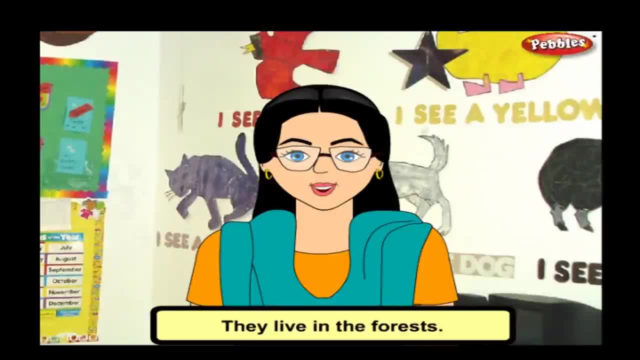 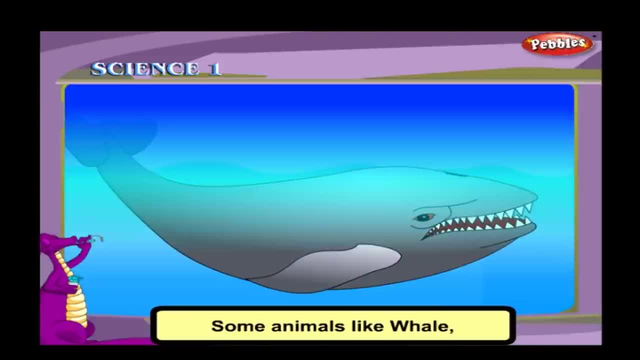 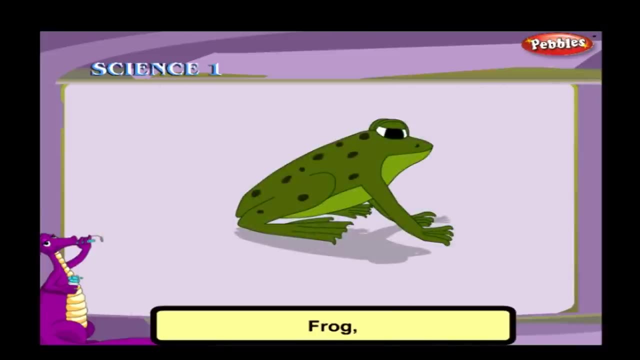 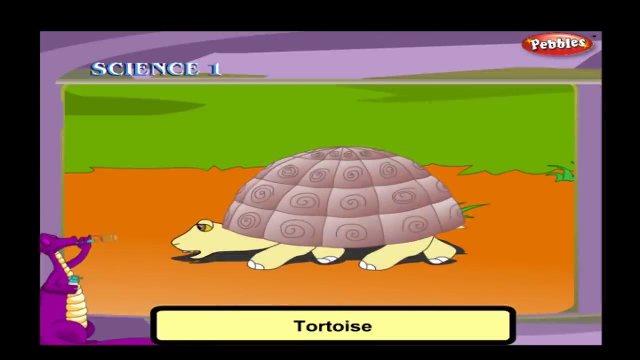 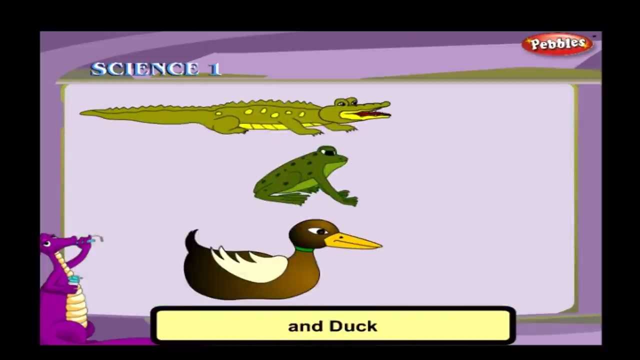 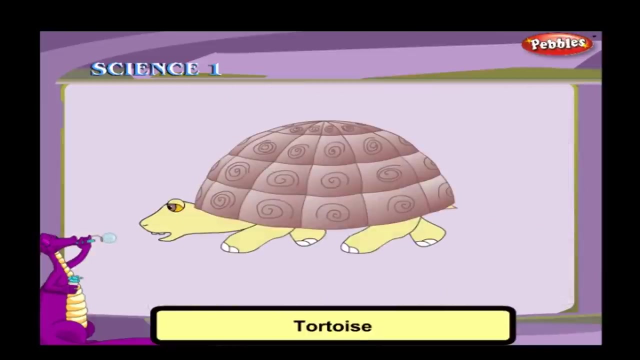 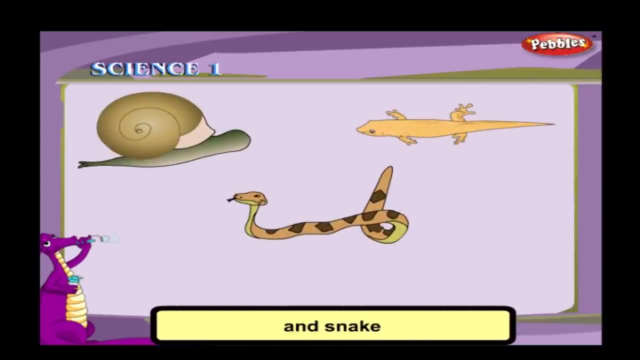 wild animals. they live in the forest. some are tamed. these animals live on land. some animals like whale, crocodile, frog, duck, tortoise and snakes live in water. crocodile frog and duck live both on land as in water. tortoise can also live both on land and water, snail, lizard and snake. 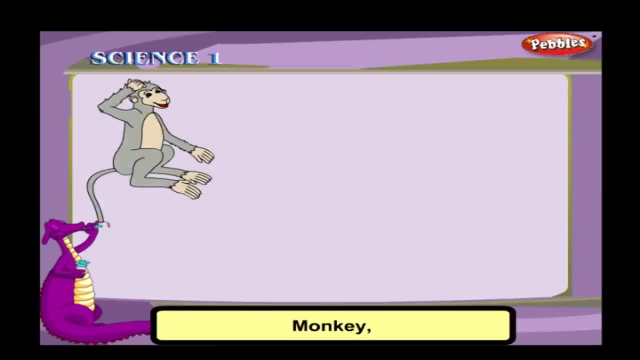 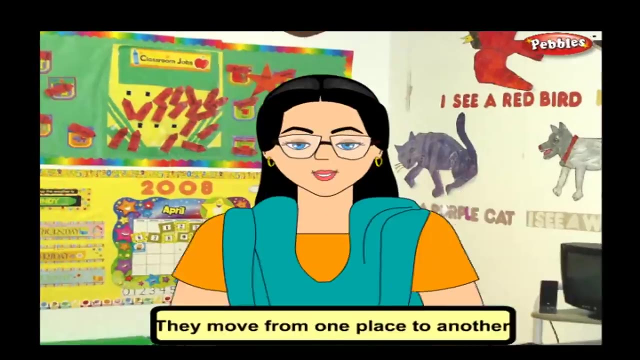 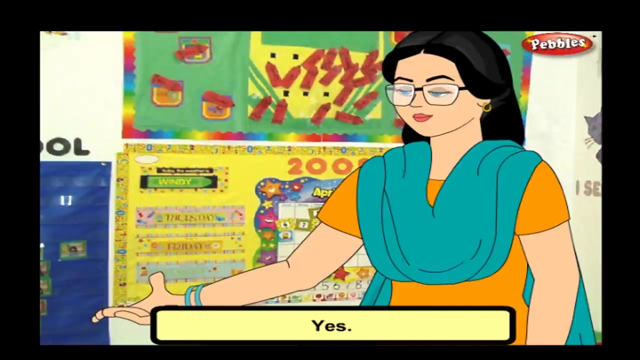 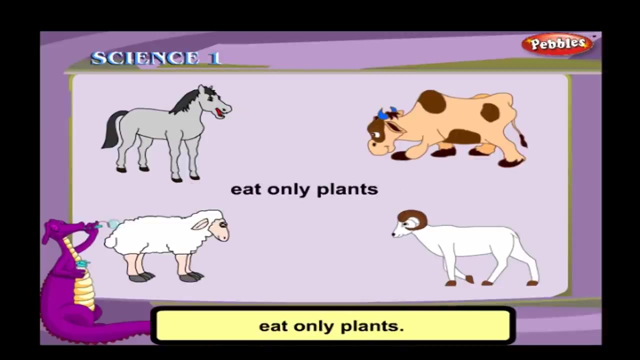 live on the ground. monkey, woodpecker and snakes live in trees and plants. do animals need food to live and grow? yes, they move from one place to another in search of food and shelter. do animals take different kinds of food? yes, horse, cow, goat and sheep eat only plants. pigeon, 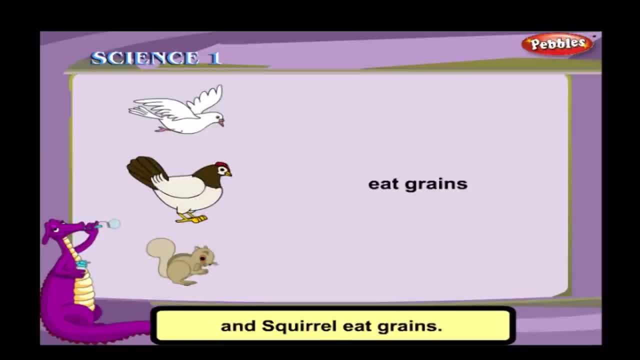 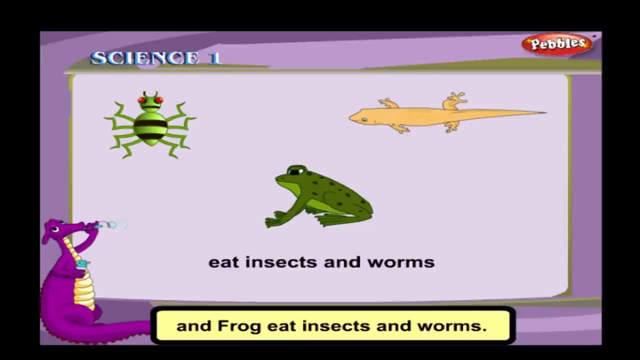 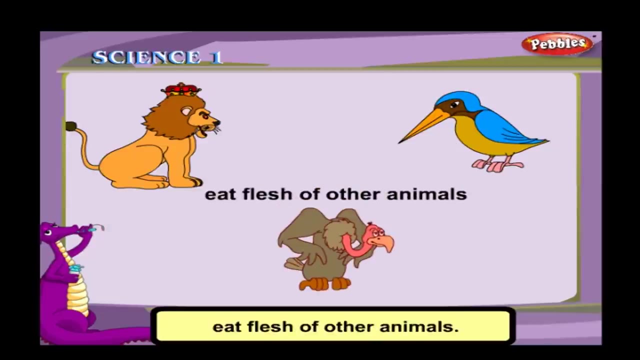 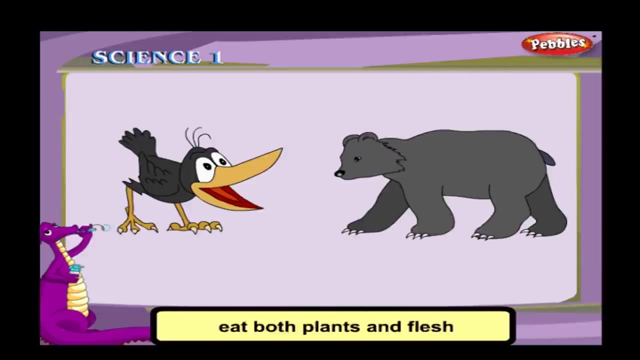 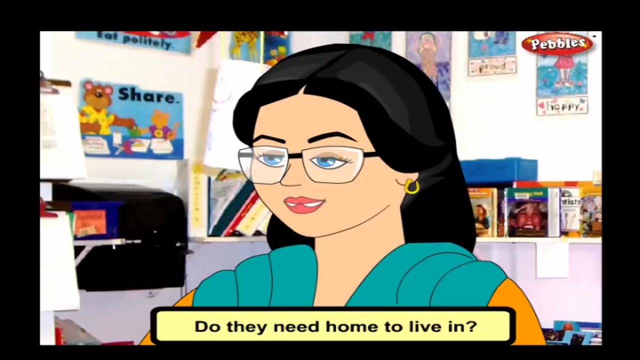 hen and squirrel eat grains. spider, lizard and frog eat insects and worms. lion, kingfisher and vulture eat flesh of other animals. bear and crow eat both plants and flesh of other animals. do they need home to live in? yes, like human beings, animals also need home to. 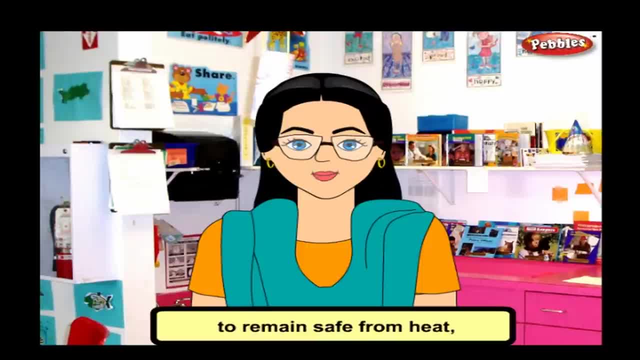 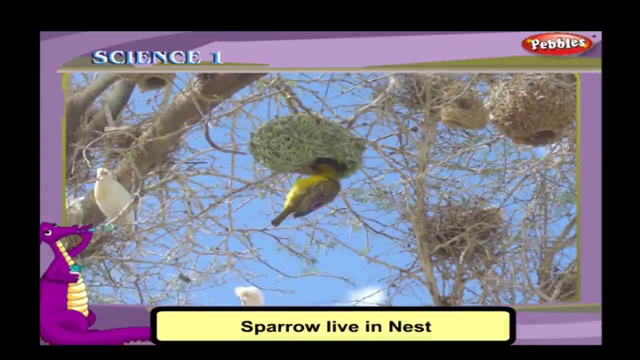 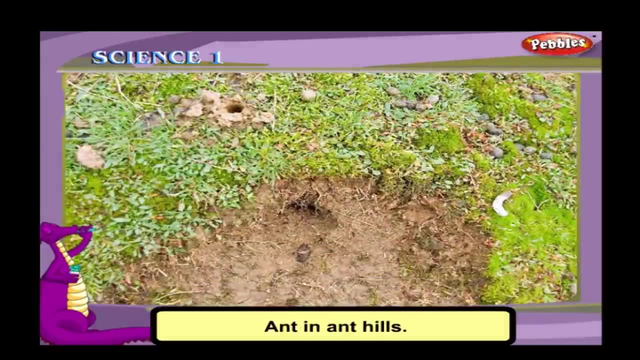 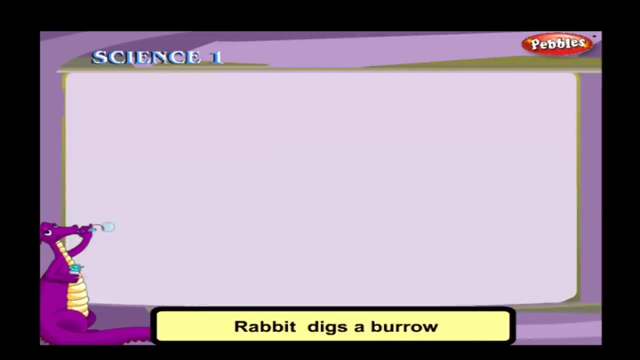 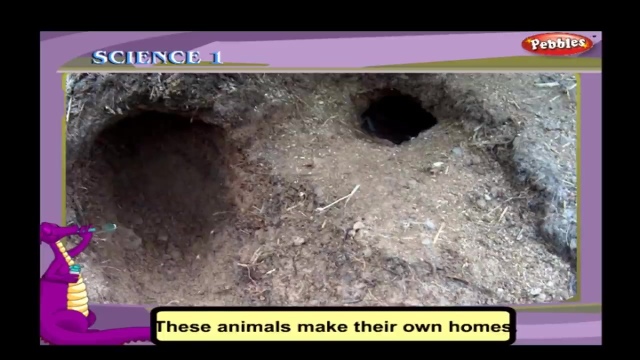 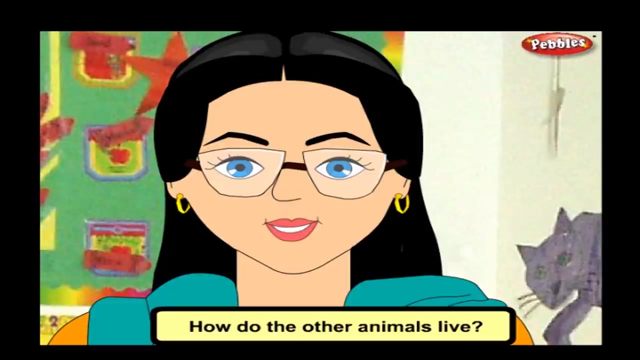 live in to remain safe from heat, cold, rain and enemies. sparrows live in a nest. spiders live in web and in and hills. rabbit in hives. rabbit digs a borrow. these animals make your own homes. lion lives in a den. how do the other animals live? we make homes for some Pet. 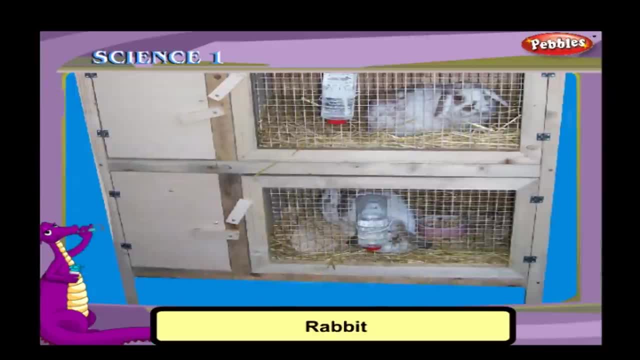 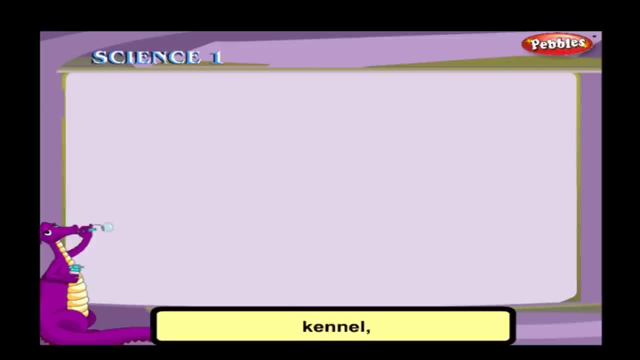 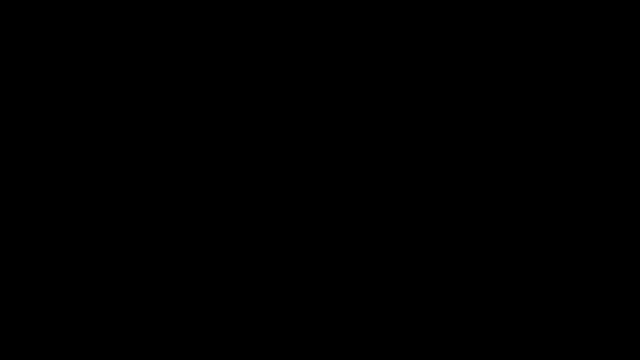 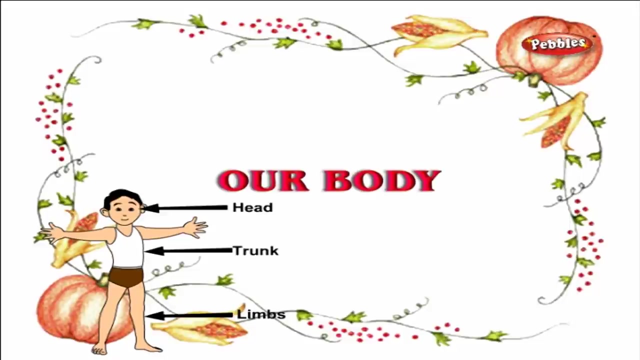 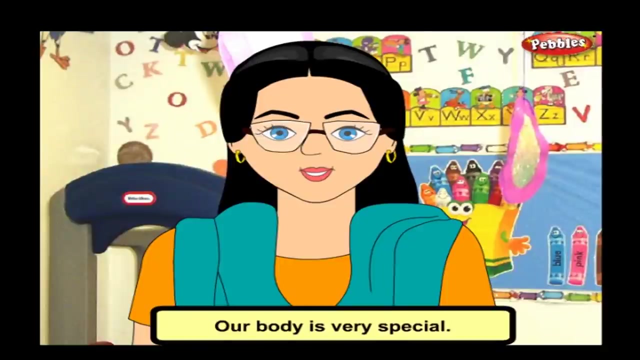 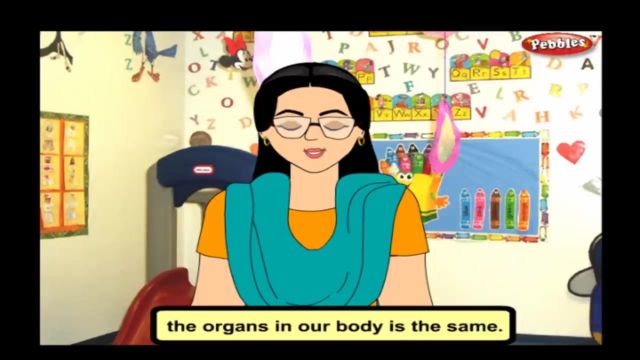 and taint animals: rabbit huts, Cork, Kennel Horse, Stable Fish Bough or an Aquarium Cows Shed. Our body is very special. we may all look different, but the organs in our body is the same. Our body consists of three main parts. They are head. 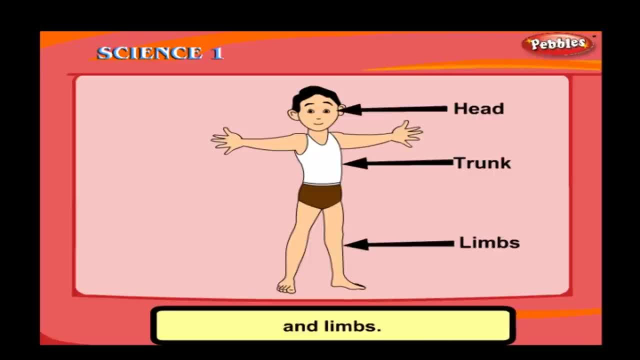 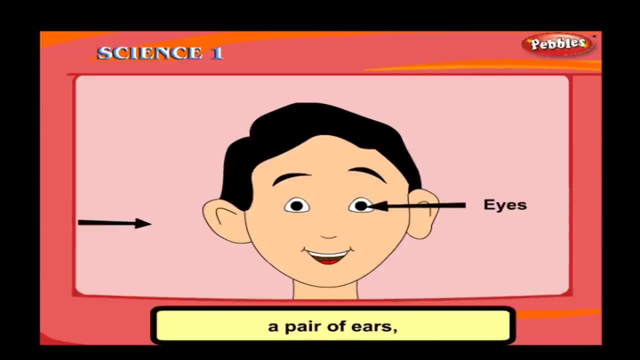 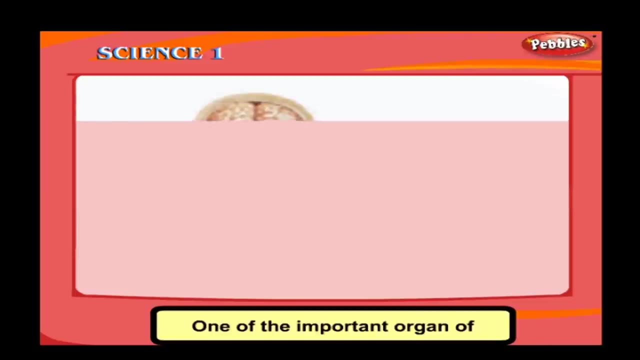 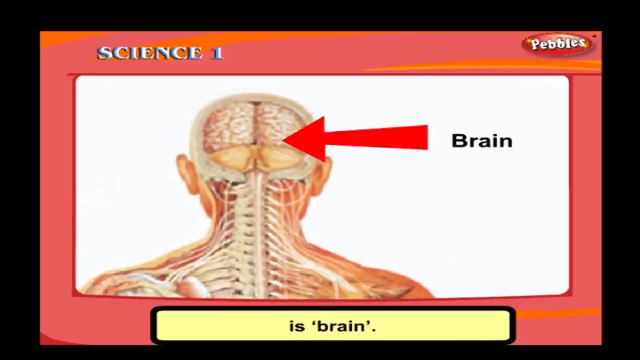 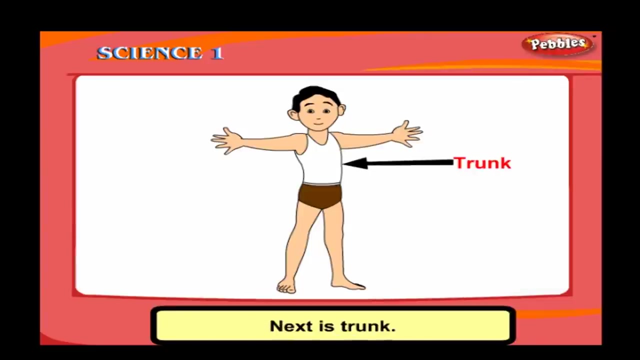 trunk and limbs Head. The head has a pair of eyes, a pair of ears, a nose and a mouth. One of the important organ of human body is the brain. The brain is situated in the head. Next is a trunk. The trunk is the main part of our body. The chest and abdomen form the trunk. The 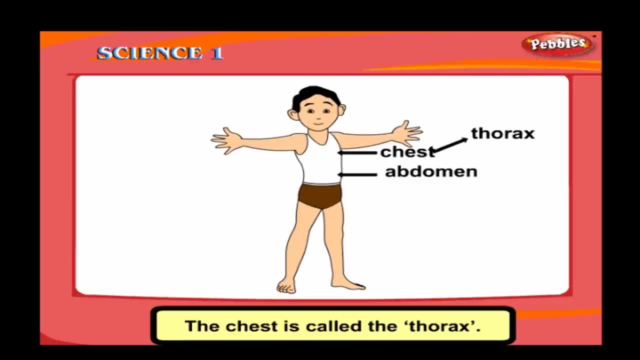 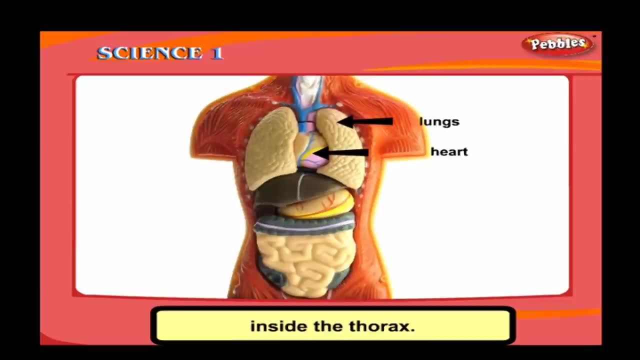 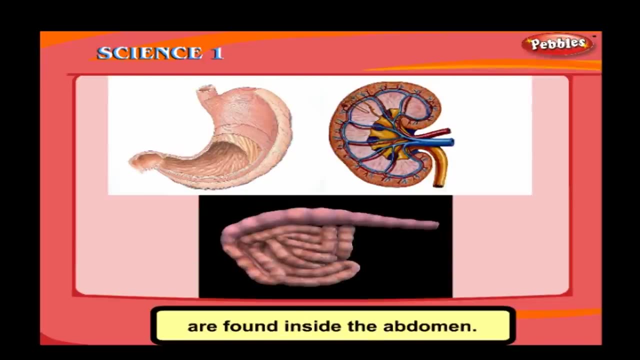 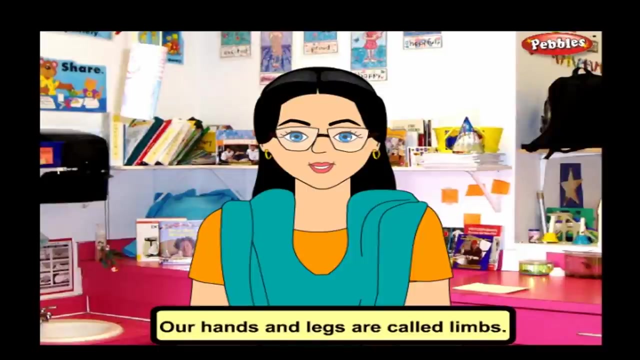 chest is called the thorax. The neck connects the head to the trunk. The heart and lungs are found inside the thorax. The stomach, kidneys and intestines are found inside the abdomen. Our hands and legs are called limbs. The legs are lower limbs and the hands are 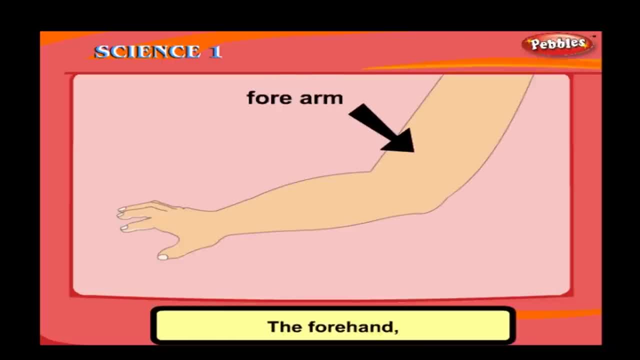 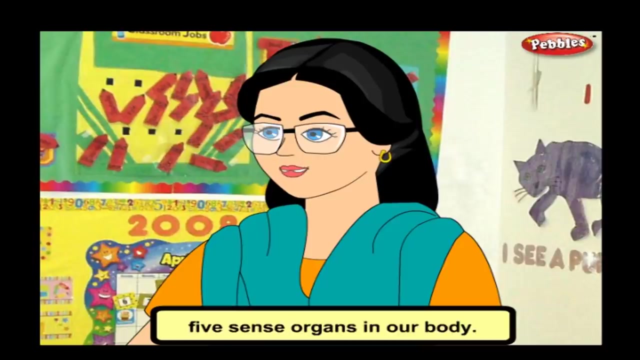 upper limbs. The forehand, elbow, wrist, palm and finger form the parts of the hand. The thigh, knee, ankle, foot and toe form the parts of the leg. We have five sense organs in our body: Eyes, ears, nose, tongue and skin are called 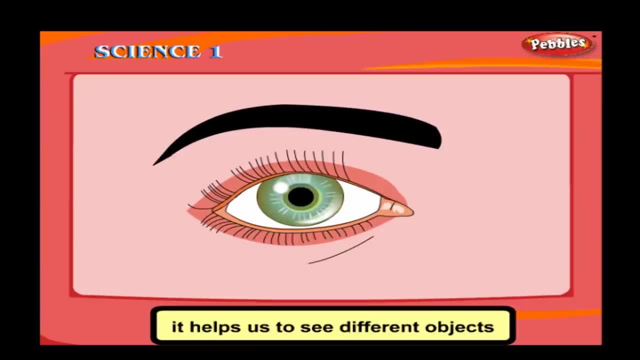 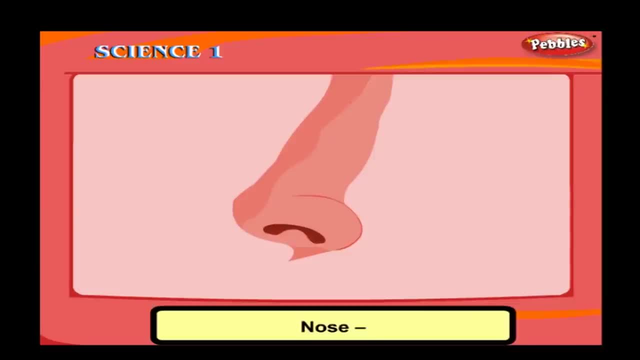 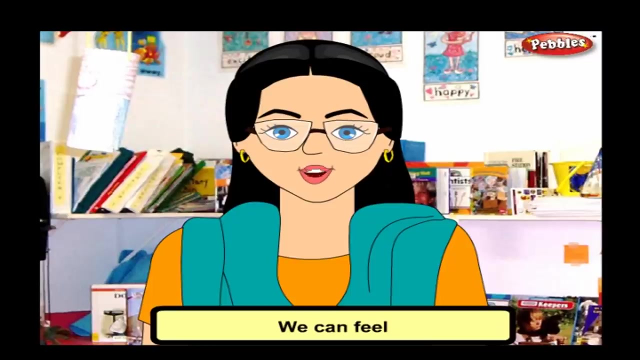 sense organs. Eyes it helps us to see different objects and their colours. Nose it helps us to smell different fragrance. Ears it helps us to hear different sounds. Tongue it helps us to know different tastes. Skin it helps us to feel. We can feel roughness. 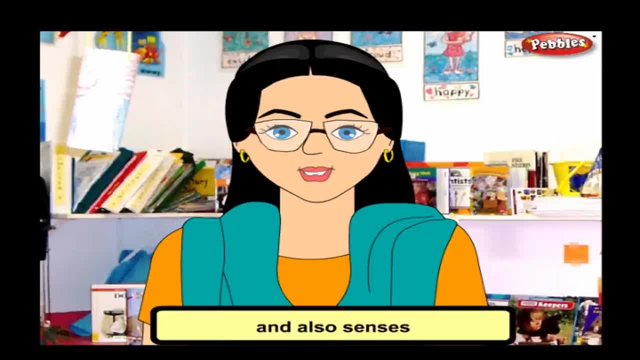 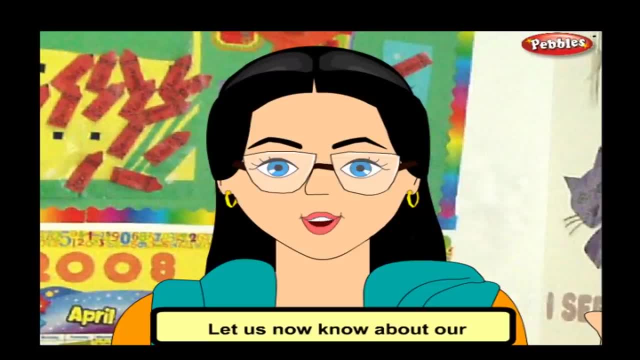 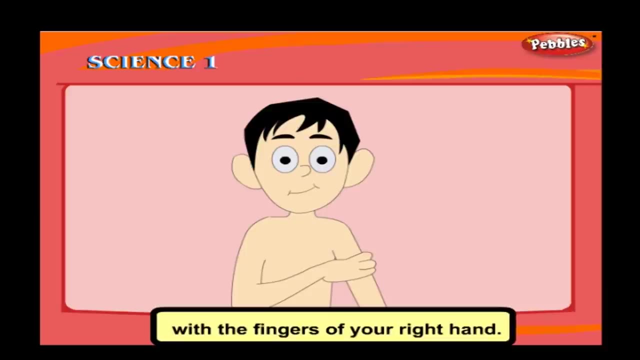 in our body. We can feel smoothness and smoothness with our skin and also sense whether the object is hot or cold with the skin. Let us now know about our bones and muscles. Press your left arm with the fingers of your right hand. What do you feel? Can you feel? 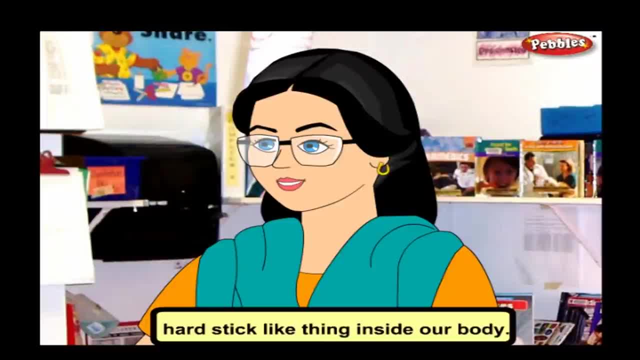 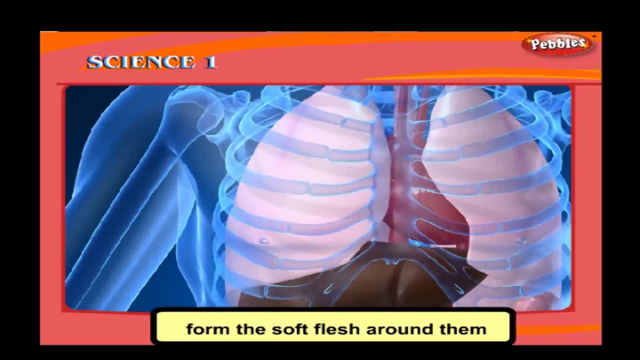 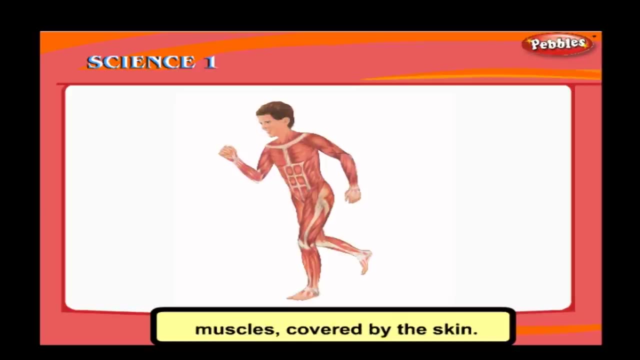 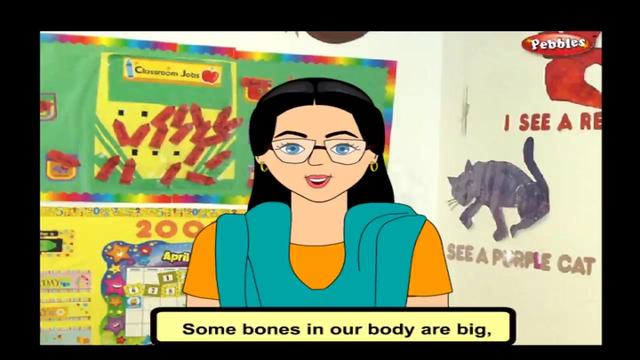 a hard, stick-like thing inside our body. The hard things in the middle are called the bones and muscles. The muscles form the soft flesh around them. Our body is made up of bones and muscles covered by the skin. It gives shape and support to our body. Some bones: 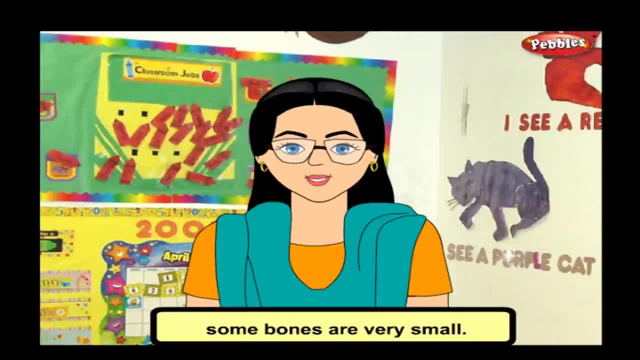 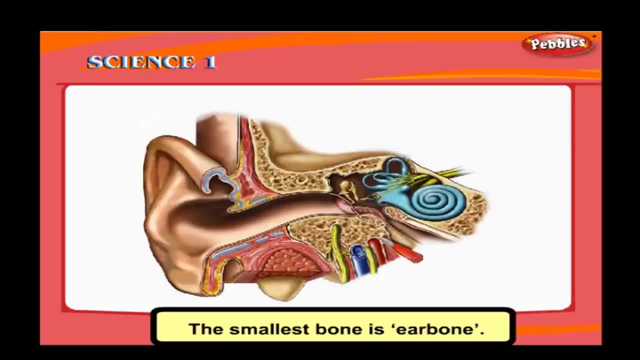 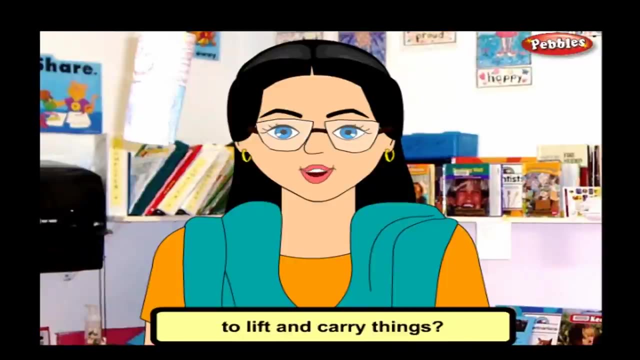 in our body are big. Some bones are very small. The thigh bone is the biggest bone in our body. The smallest bone is the ear bone. The thigh bone is the biggest bone in our body, The smallest. from where do we get strength to lift and carry things? it is from our muscles. some muscles are 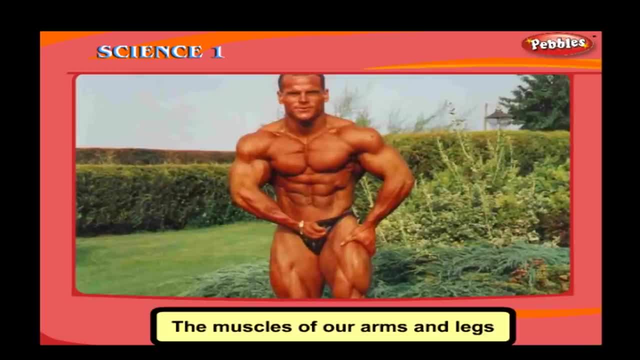 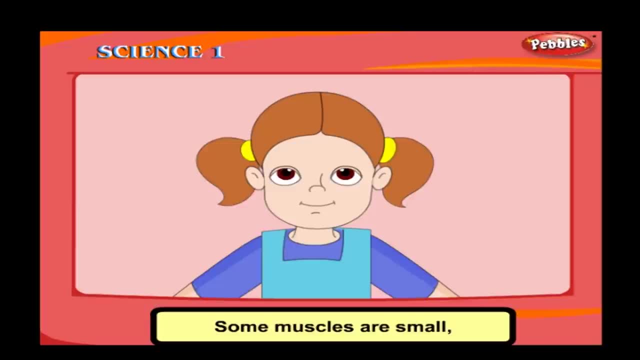 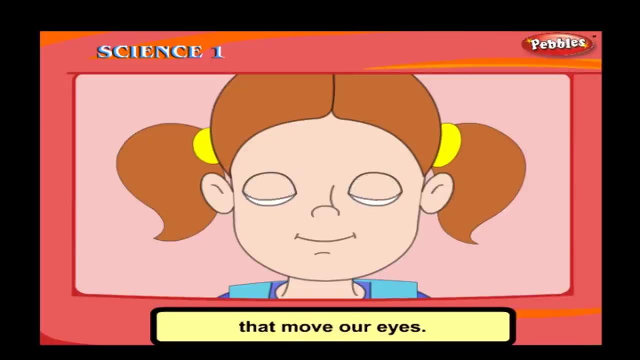 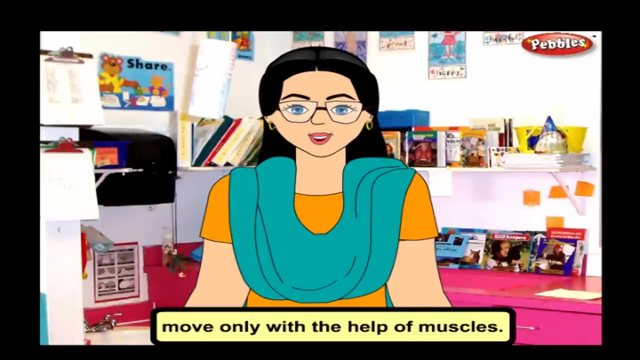 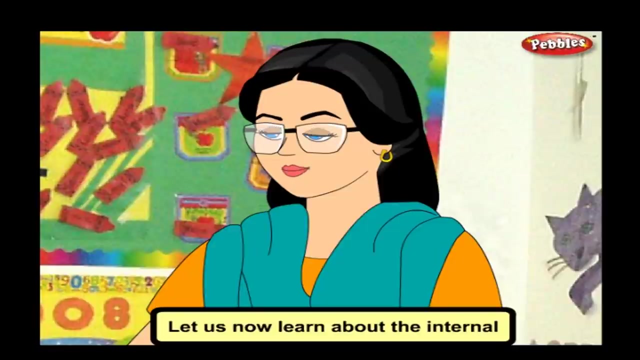 big and strong. the muscles of our arms and legs are big and strong. some muscles are small, like the muscles of the eyes. they move our eyes. all parts of the body move only with the help of muscles. there are some muscles that do not move. let us now learn about the internal organs of our 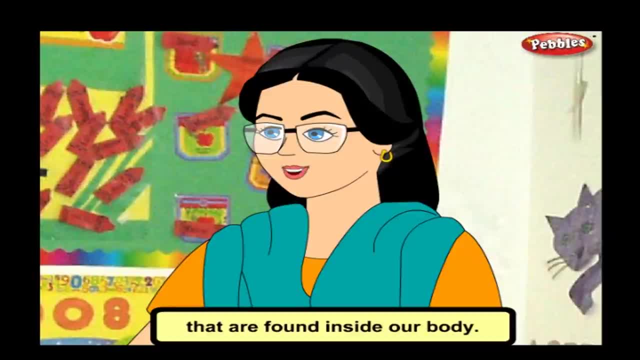 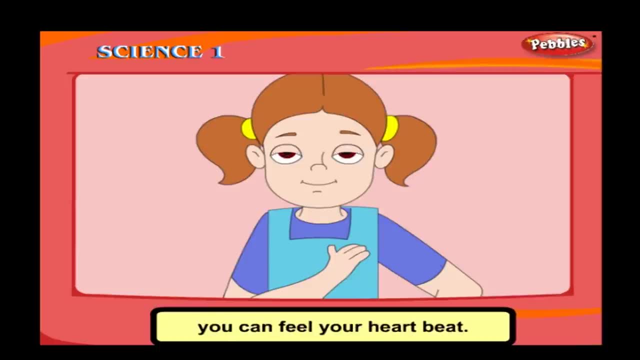 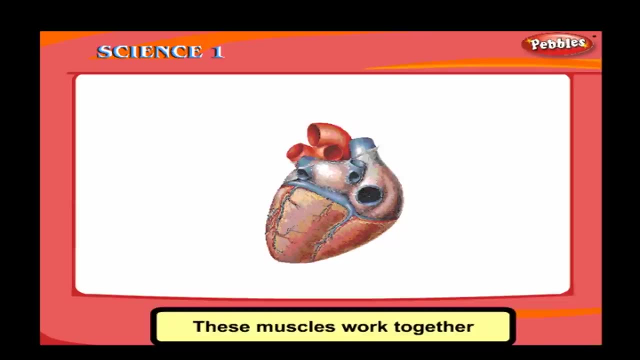 body that are found inside our body. if you keep your palm on the left side of your chest, you can see the muscles of the eyes. they move our eyes. all parts of the body move only with the help of your heart beat. heart is the organ made up of muscles. these muscles work together and pump. 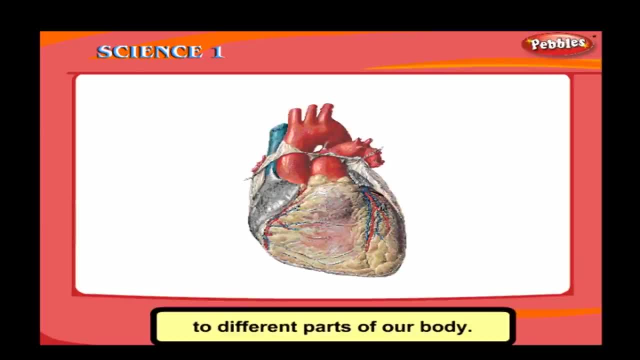 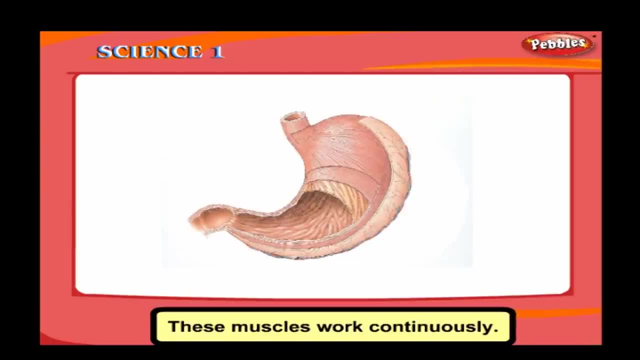 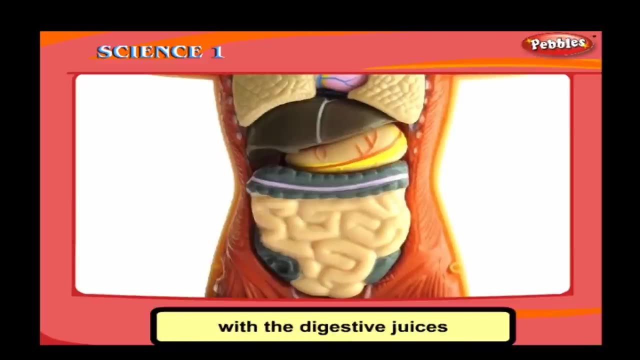 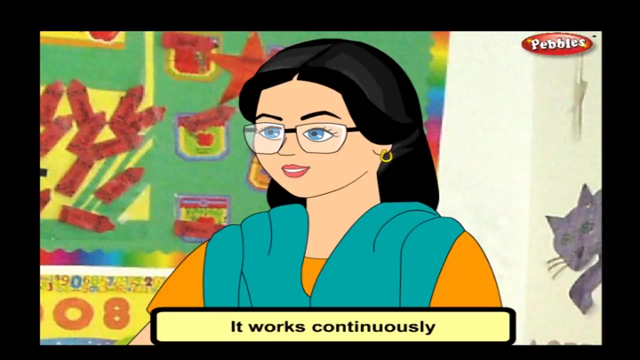 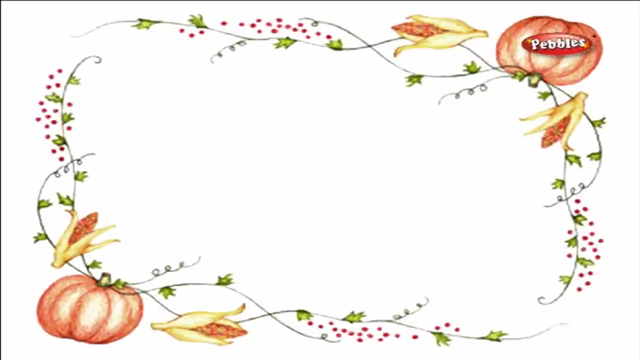 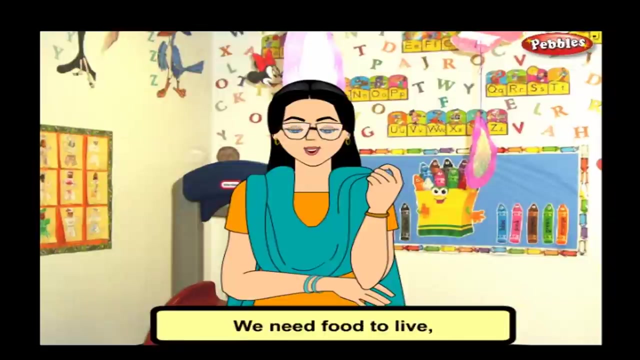 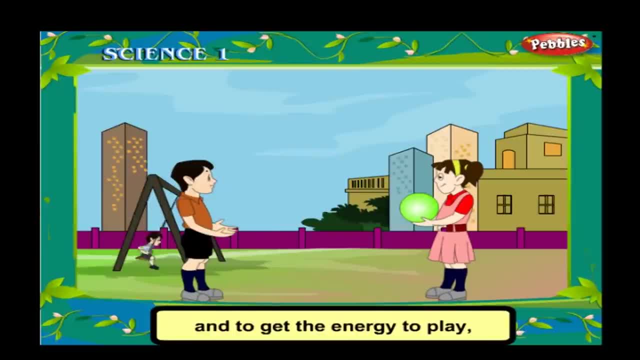 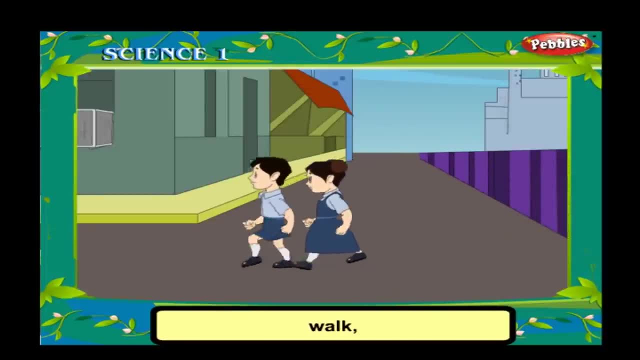 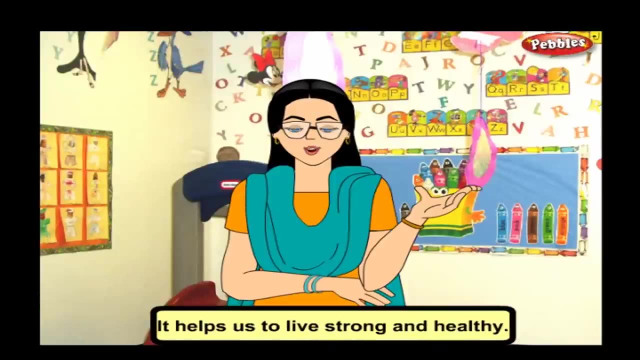 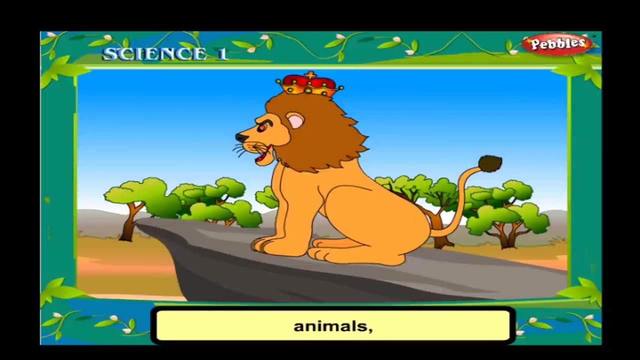 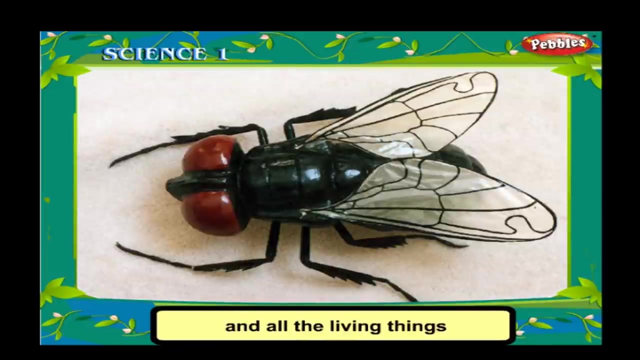 and to get the energy to play, run, walk, work and to do many more activities. it helps us to live strong and healthy. do you know that all living things need food? plants and in Animals, birds, insects and all the living things need food to live. 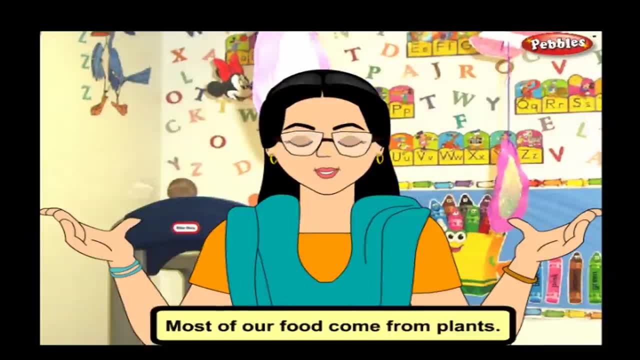 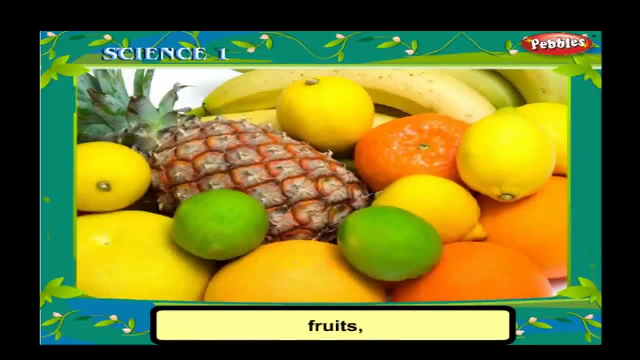 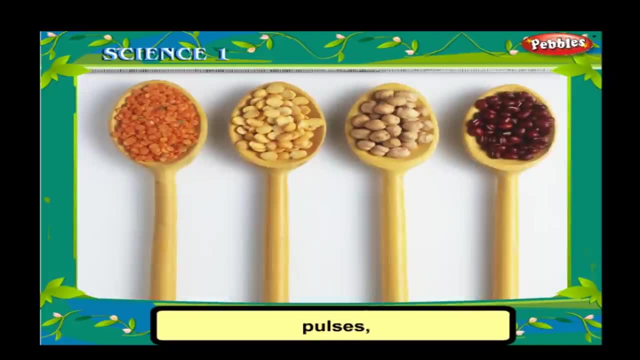 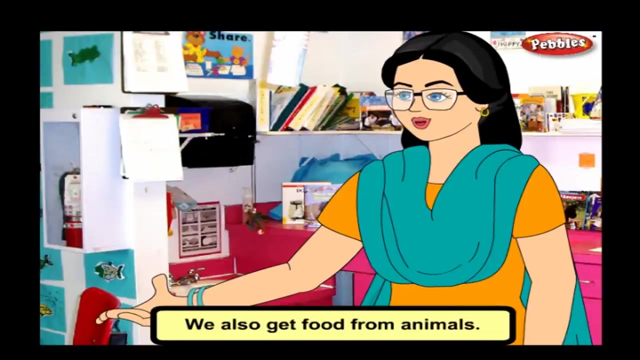 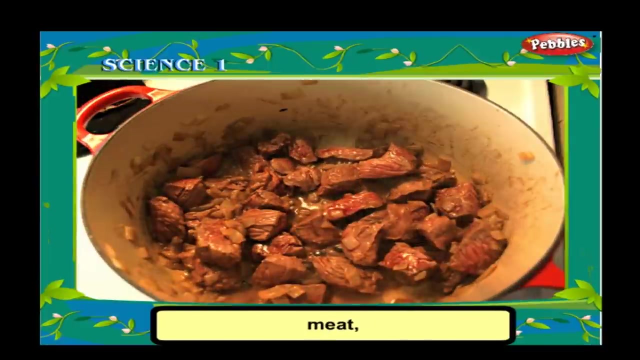 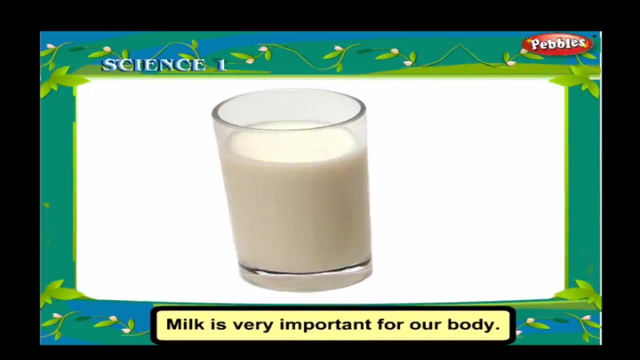 Where do we get our food from? Most of our food comes from plants: vegetables, fruits, nuts, grains, pulses, cereals, etc. We also get food from animals. Examples are meat, milk, eggs, etc. Milk is very important for our body. 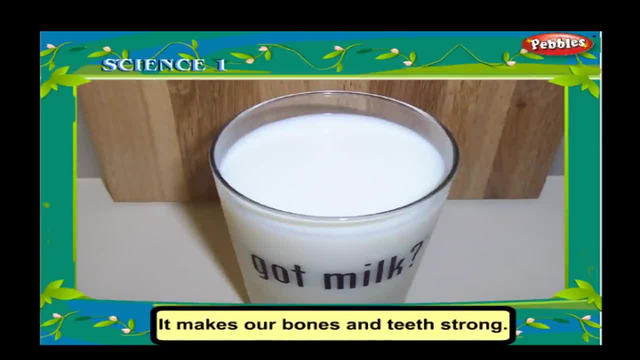 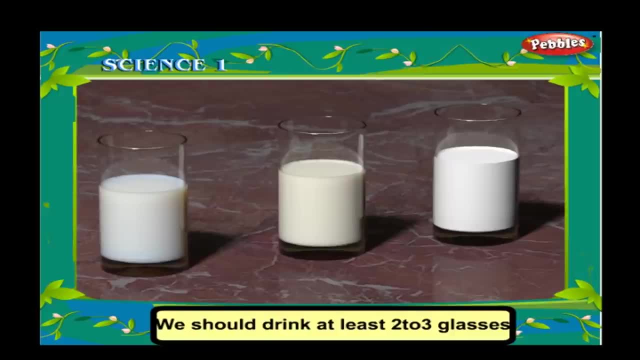 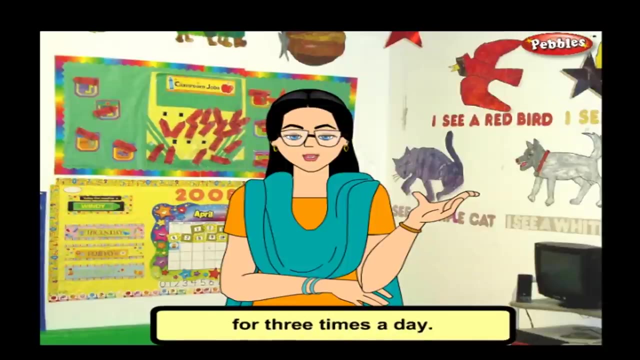 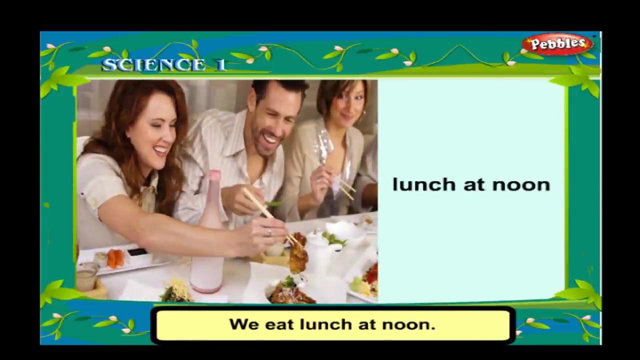 It is called a complete food Food. It makes our bones and teeth strong. We should drink at least two to three glasses of milk every day. Food is eaten by us generally for three times a day. We eat breakfast in the morning. We eat lunch at noon. 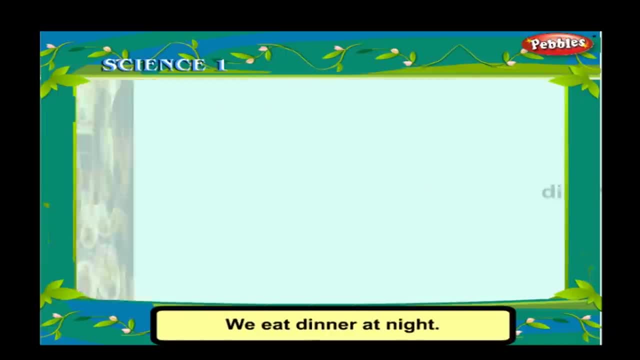 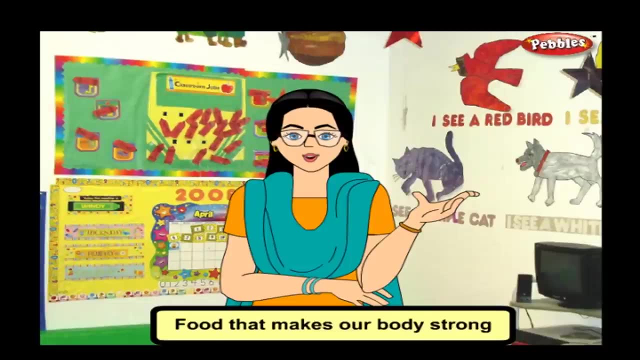 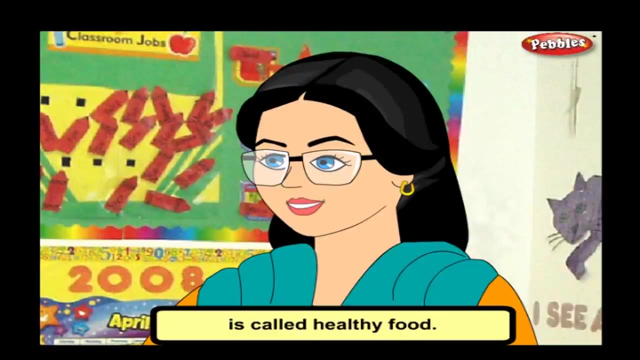 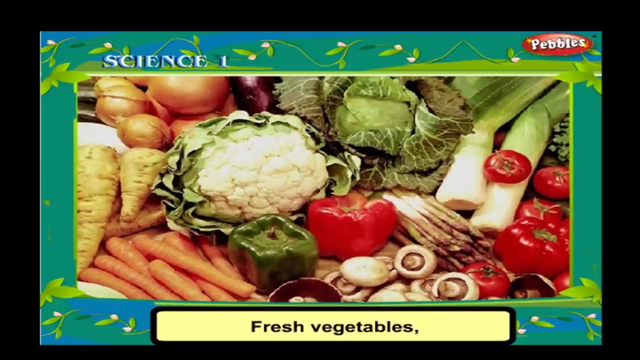 We eat dinner at night. Having seen about food, let us see what is healthy food. Food that makes our body strong and which helps us stay healthy is called healthy food. Let me tell you what are the healthy food: Fresh vegetables, fruits. 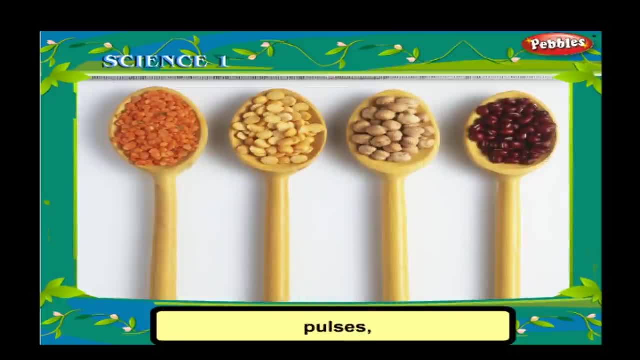 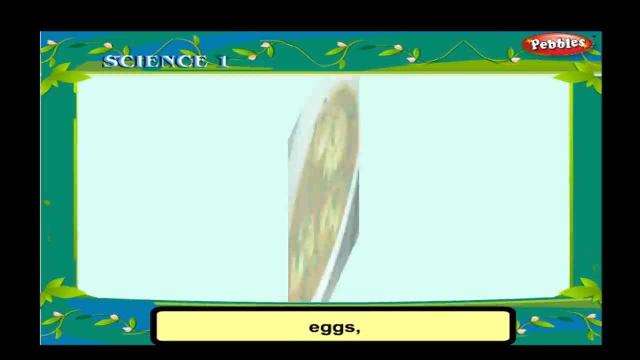 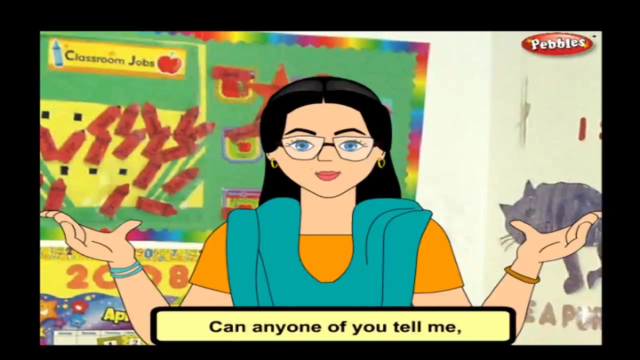 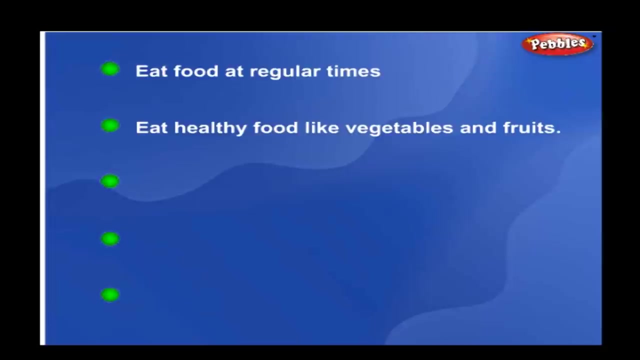 cereals, pulses, milk, eggs, meat are very healthy for our body. Can any one of you tell me about the good eating habits that we should follow? I will tell you now. Eat food at regular times. Eat healthy food like vegetables and fruits. 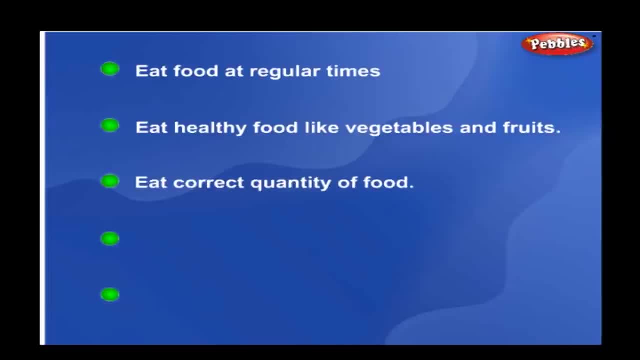 Eat correct quantity of food. Eat healthy food like vegetables and fruits. Eat correct quantity of food. Eat correct intake of the moderate quantity of food. Drink plenty of water. Drink plenty of water- At the least two liters. Drink at least two liters. 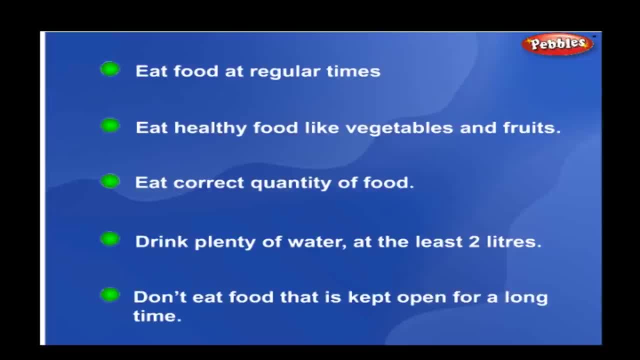 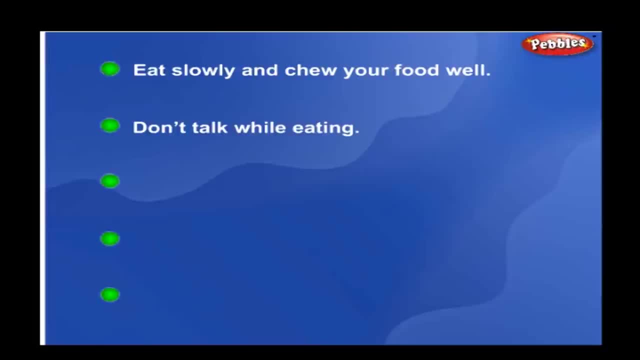 Don't eat food that is kept open for a long time. Don't eat food that is kept open for a long time. Eat slowly and chew your food well. Eat slowly and chew your food well. Don't talk while eating. Don't talk while eating. 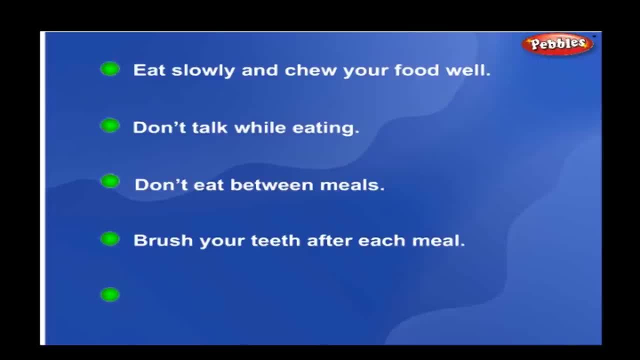 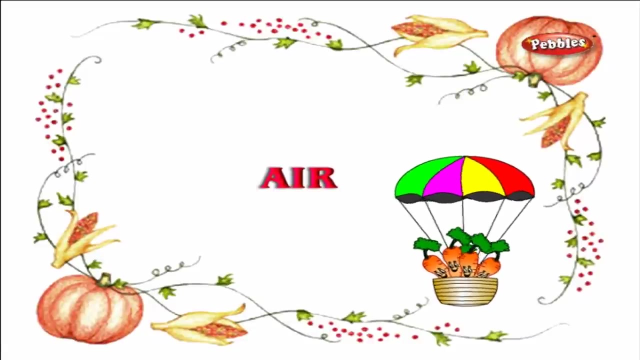 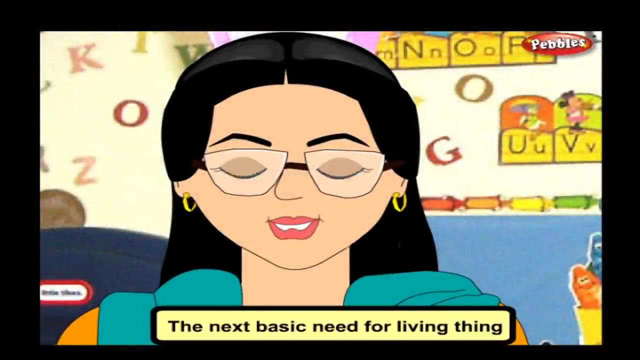 Don't eat between meals. Brush your teeth after each meal. Brush your teeth after each meal. We break our teeth during meals. We spread our mouth widely. eat clean and healthy food. the next basic need for living thing is air. can we see air? no, we cannot see air. 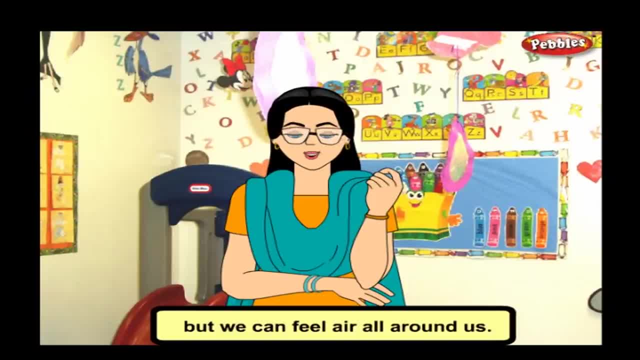 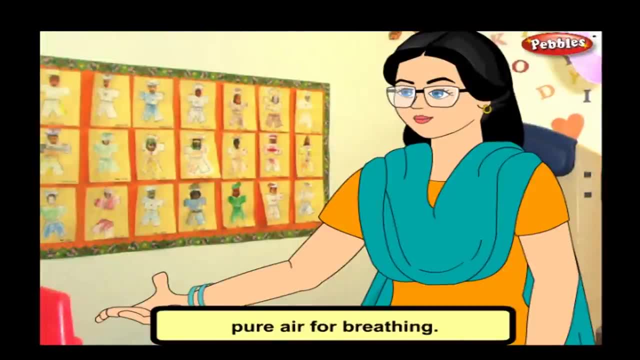 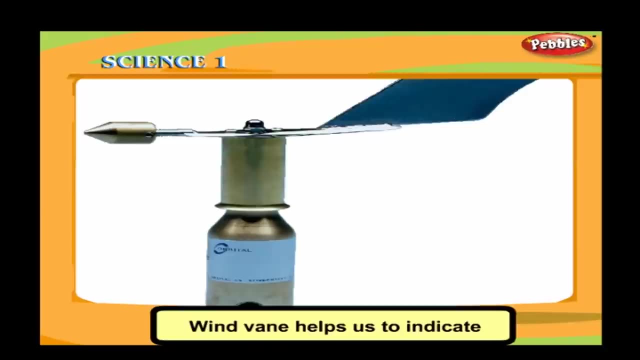 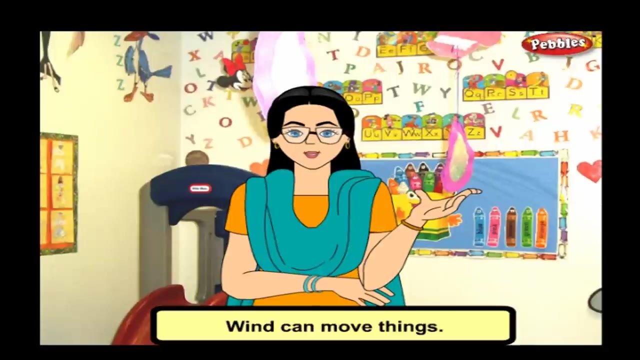 because it has no color, but we can feel air all around us. living things need fresh and pure air for breathing. moving air is called wind. wind vane helps us to indicate the direction of the wind. wind can move things. I will show you some things that move with the help of. 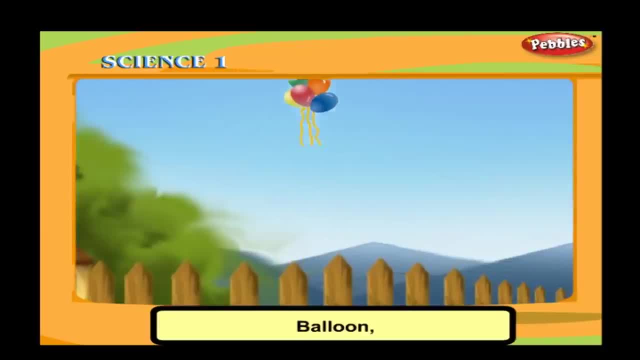 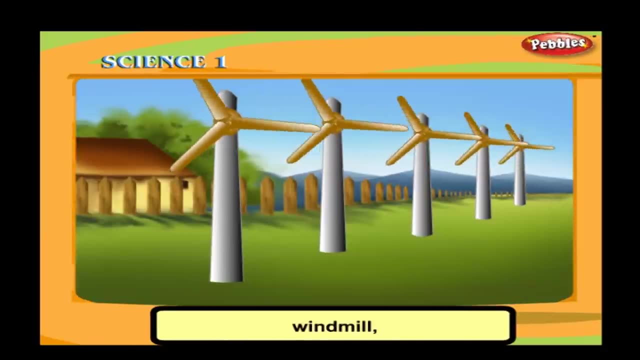 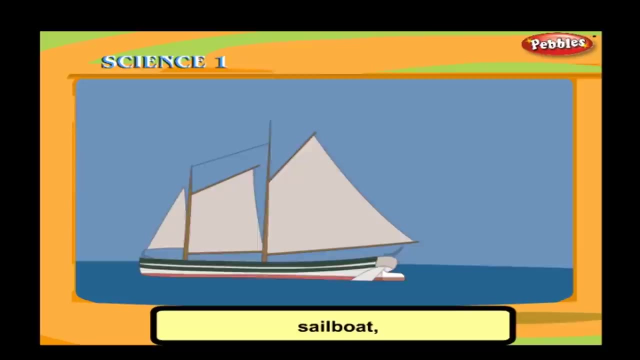 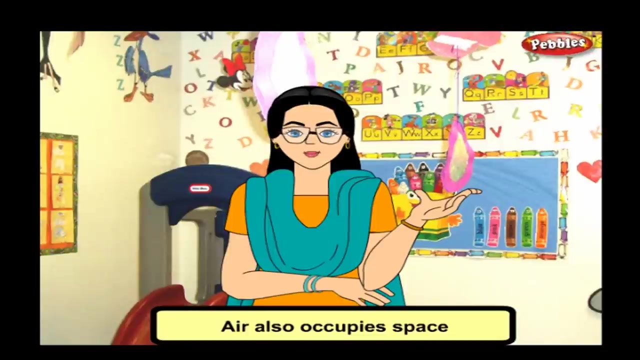 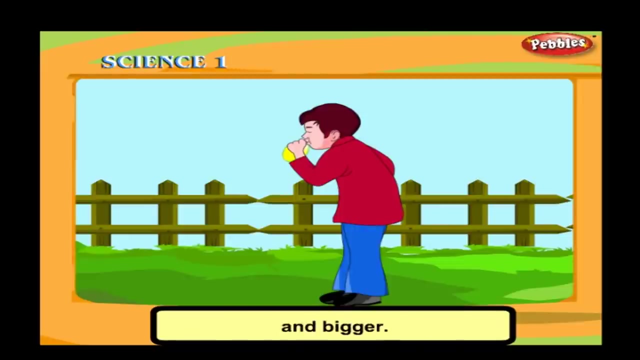 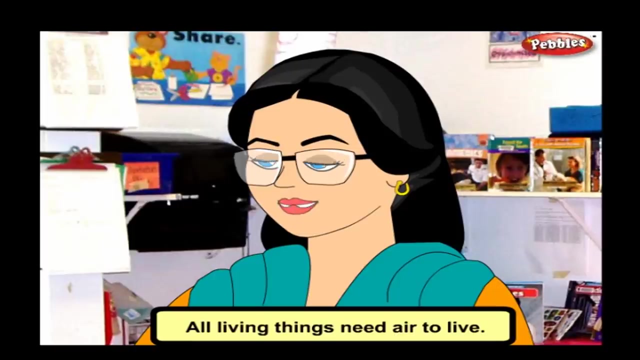 the air balloon, kite, birds, windmill, aeroplane, sailboat, parachute, etc. air also occupies space. blow air into a balloon. see how it becomes. air comes bigger and bigger. the air that you blow in fills up the space inside the balloon. so we can see that air occupies the space. all living things need air to. 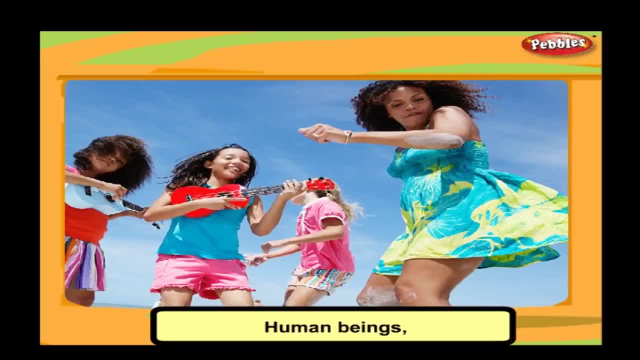 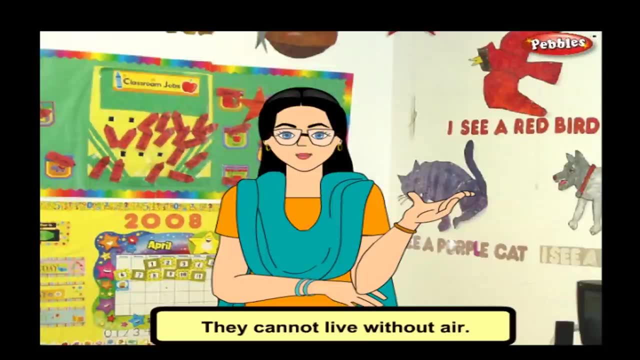 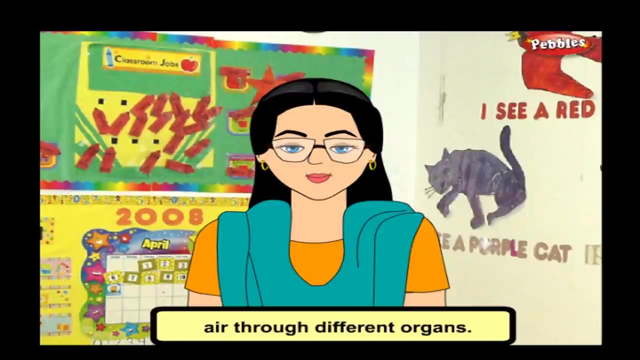 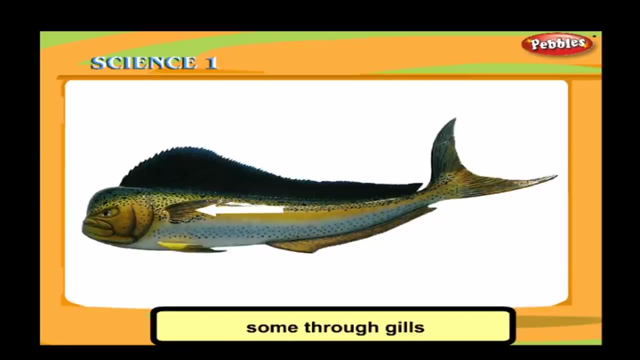 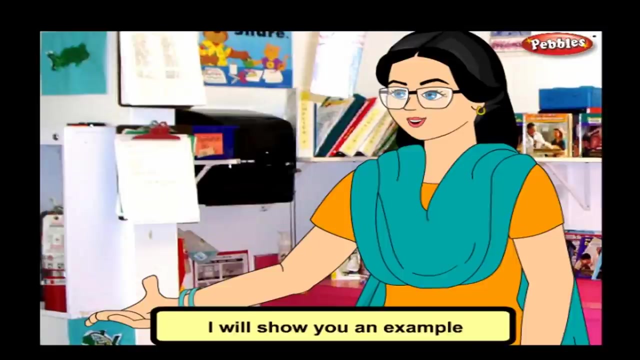 live. human beings, animals and plants breathe in air. they cannot live without air. they will die without air. different living things breathe in air through different organs. some living things breathe through lungs, some through gills and some through air holes. I will show you an example that living things cannot live without air. 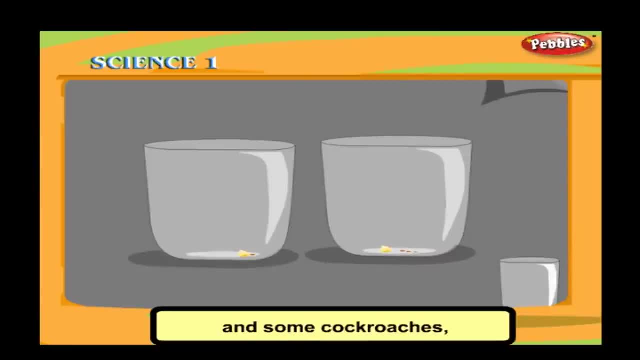 take two glass bottles and some cockroaches. put some cockroach inside both the bottle and close the first bottle with the tight lid and the second bottle with a lid with some holes. keep it aside for one or two days. see what happens to the cockroaches. you can see that the 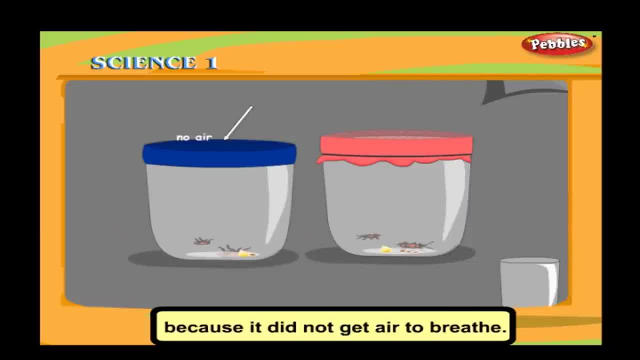 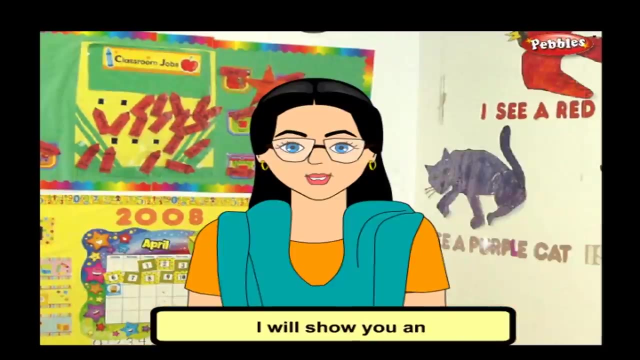 cockroach in the first bottle dies because it did not get air to breathe. the cockroach could not breathe. how to breathe with air in a bottle? in the second bottle lives because it gets air to breathe. we also need air for burning. I will show you an example for this. also light a candle and leave it. 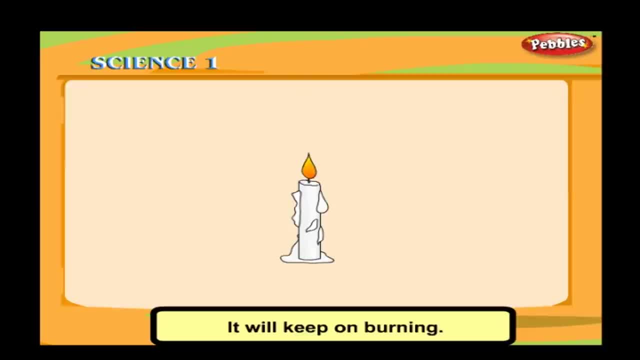 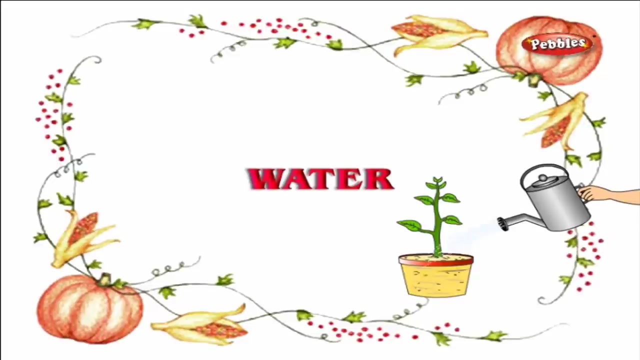 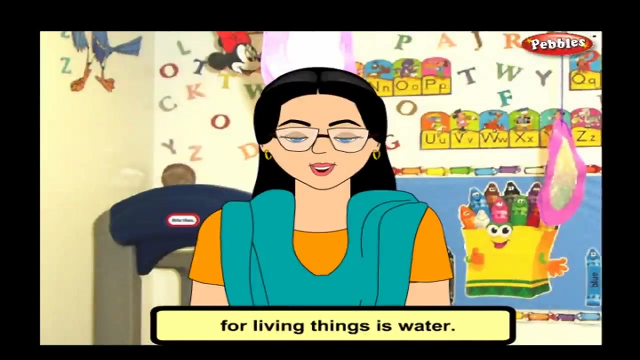 for some time it will keep on burning. now close the burning candle with a glass jar. in a little moment the candle will stop burning. this is because there is no air inside. the next basic need for living things is water. let us see the uses of water we. 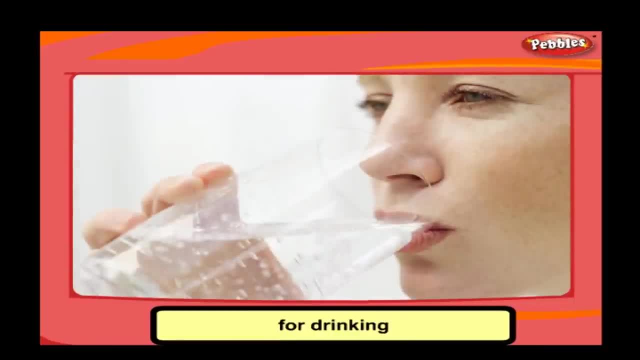 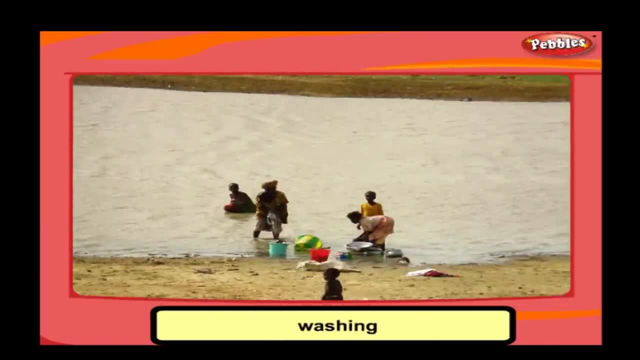 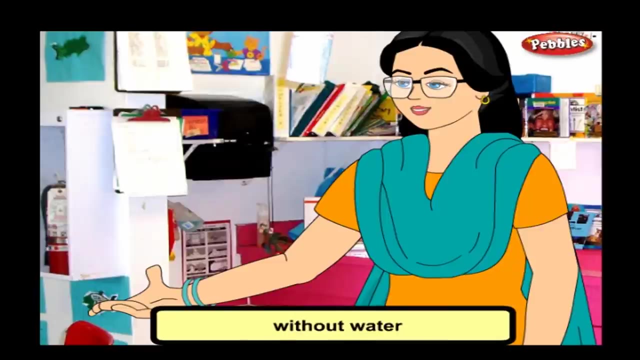 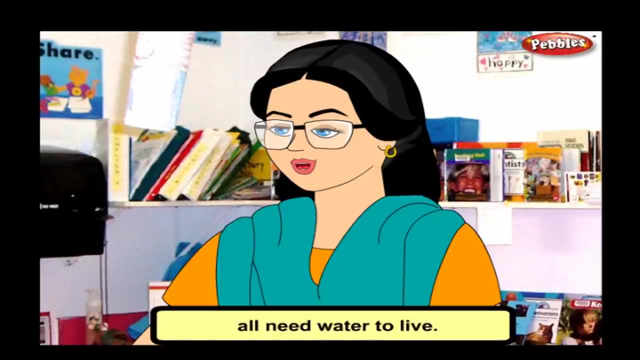 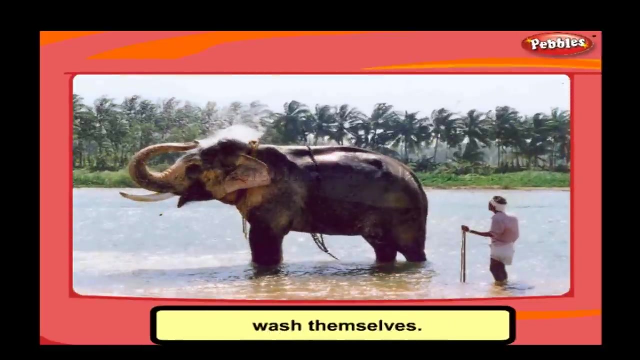 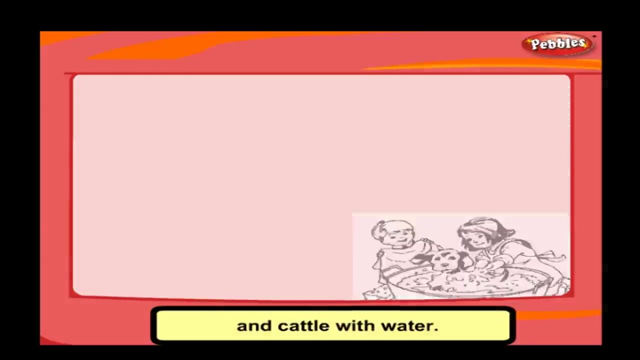 need water for drinking, cooking, bathing, washing and cleaning. Living things cannot live without water. Human beings, animals and plants all need water to live. Animals also drink water. They need water to wash themselves. We wash our pet animals and cattle with water. 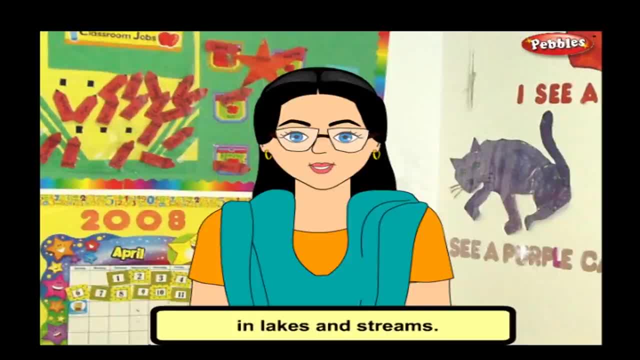 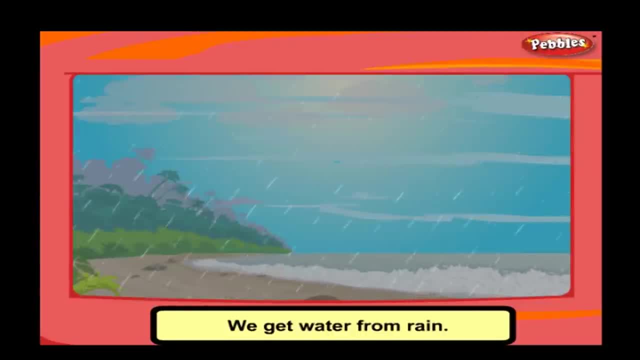 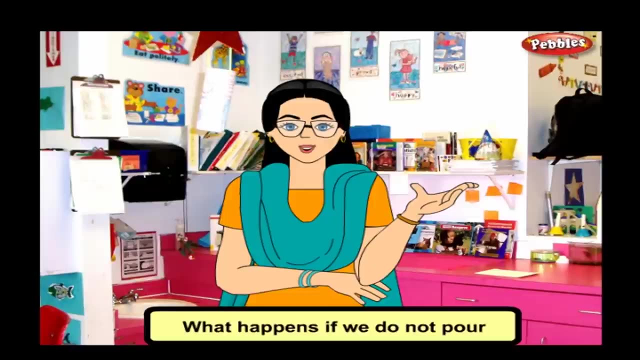 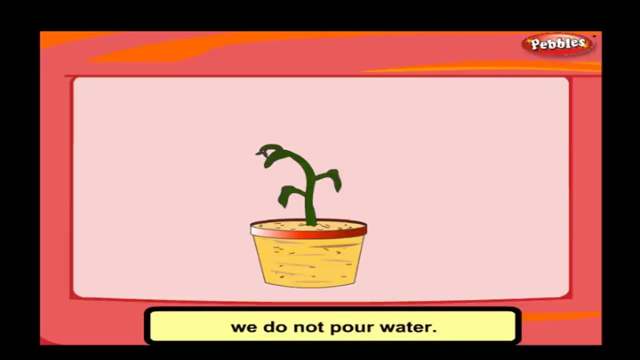 Forest animals take bath in lakes and streams. From where do we get pure water? We get water from rain. Rain falls from the clouds. What happens if we do not pour water to a plant? for a few days? Plants dry up and die if we do not pour water. 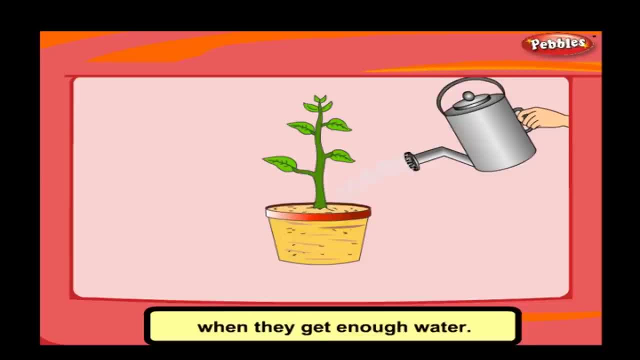 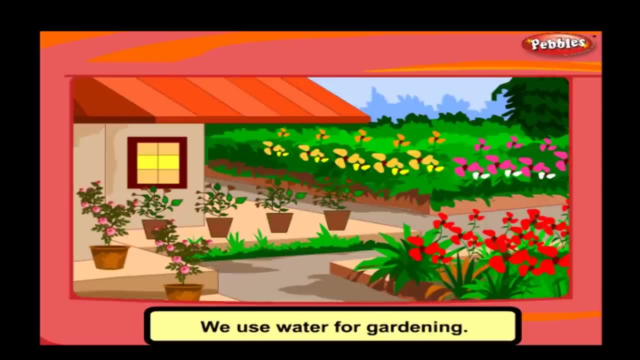 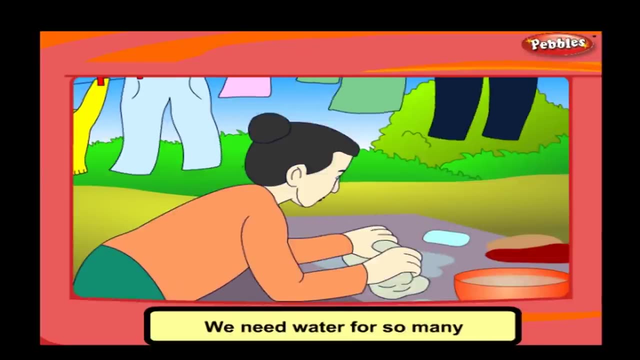 Plants grow well when they get enough water. They use water to make food. We use water for gardening. Farmers use water for growing crops. We need water for so many other purposes. Water is so important to everyone. We need water for everything. 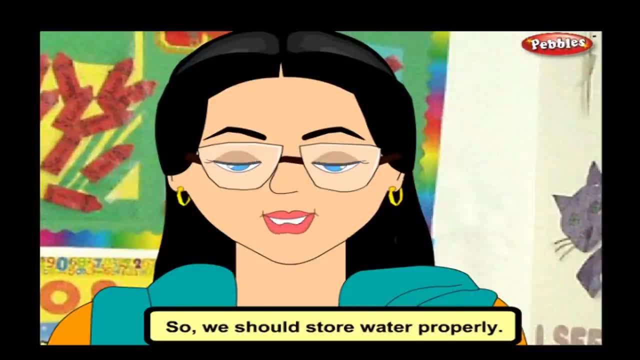 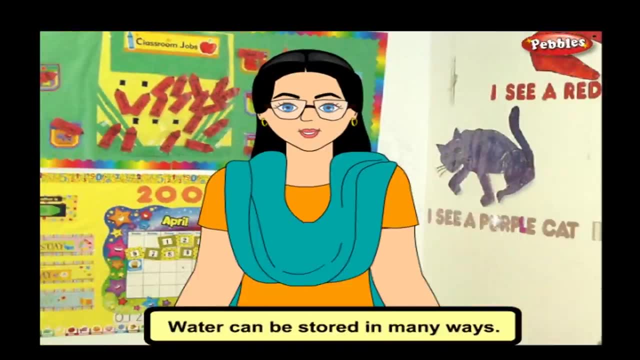 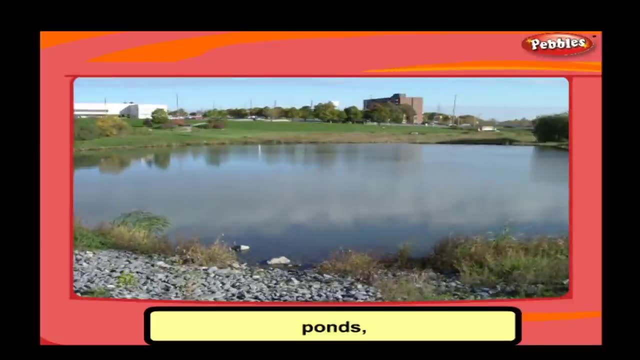 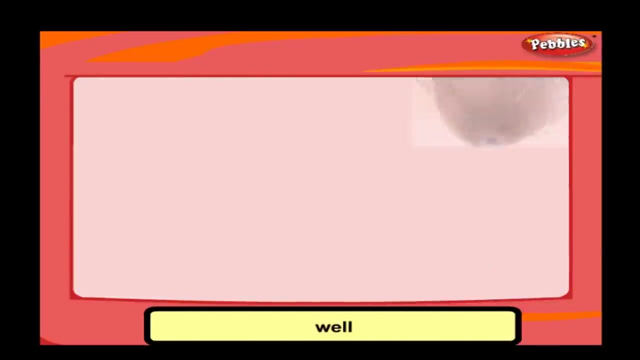 We need water for everything, So we should store water properly. I will tell you the different methods in which we can store water. Water can be stored in many ways: In dams, ponds, lakes, well, and also in buckets. Water is very precious. 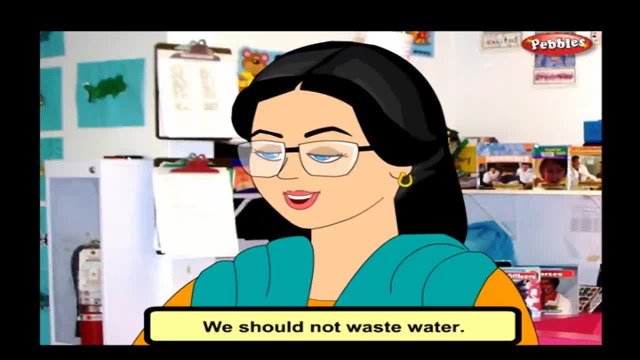 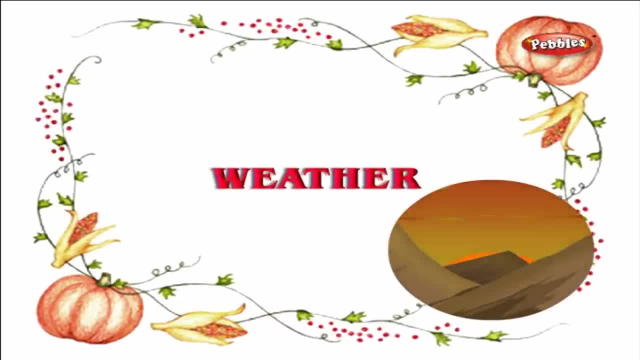 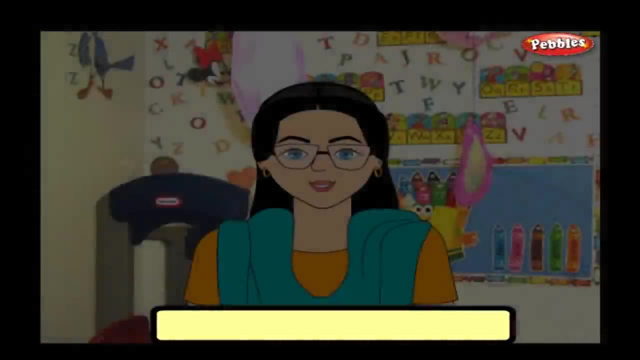 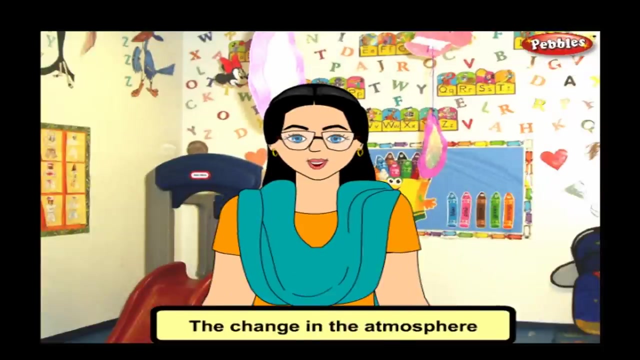 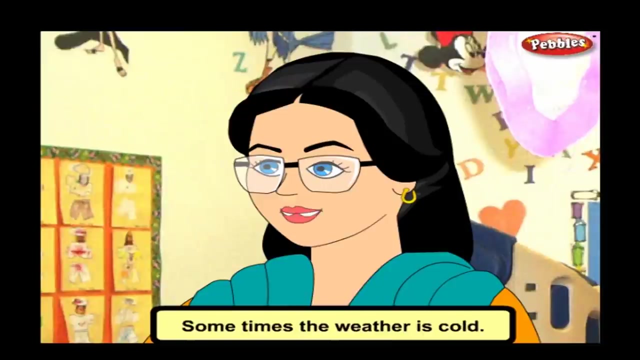 Where does it come from? Great, We should not waste water. We should not throw waste into the water. Do any one of you know what is weather? The change in the atmosphere is called weather. Sometimes the weather is hot, Sometimes the weather is cold. 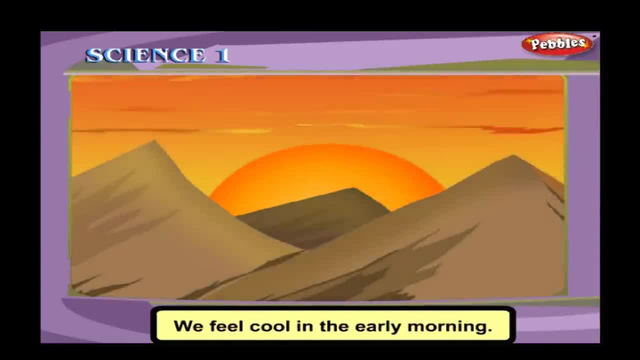 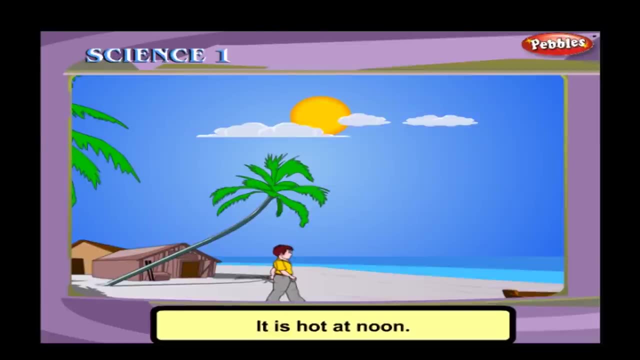 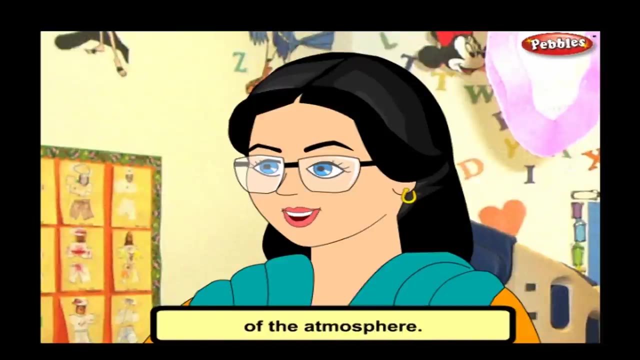 We feel cool in the early morning, So we say the morning weather is cool. It is hot. at noon Now we say the weather is hot. Weather is the condition of the atmosphere. Weather changes from time to time and day to day. 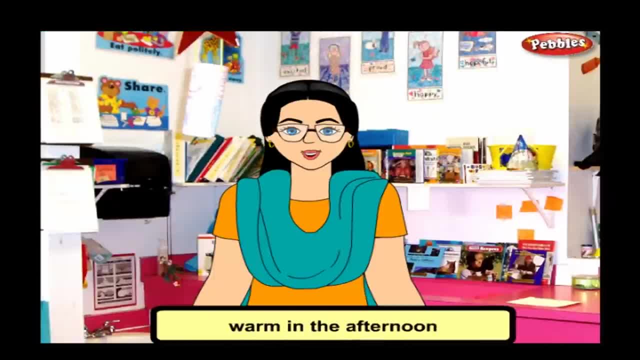 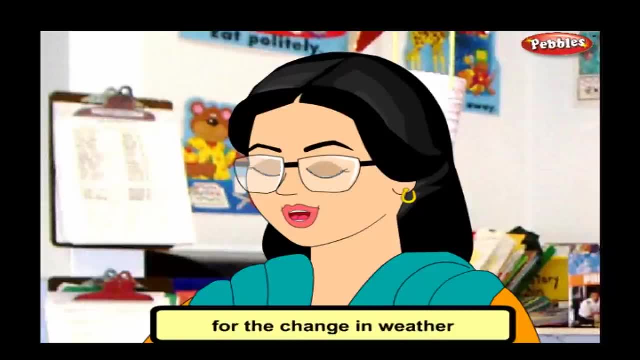 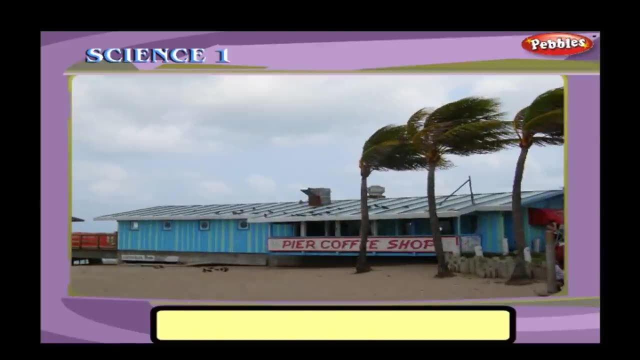 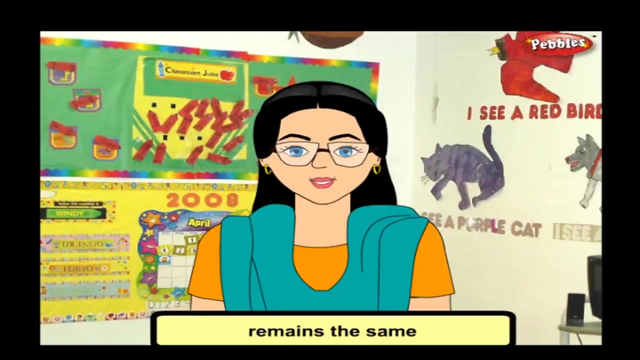 It may be cold in the morning, Warm in the afternoon And cold in the night again. There are many reasons for the change in weather. The sun, The wind And the rain causes changes in the weather When a particular weather remains the same for a period of time. 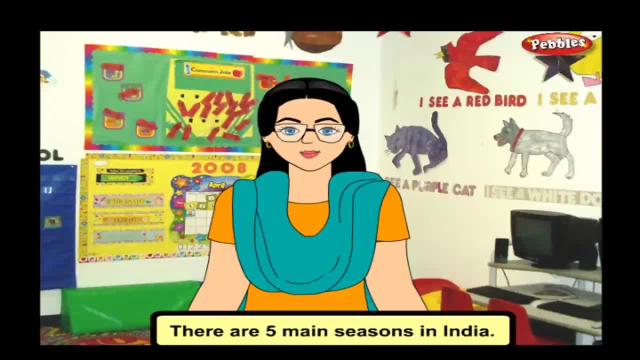 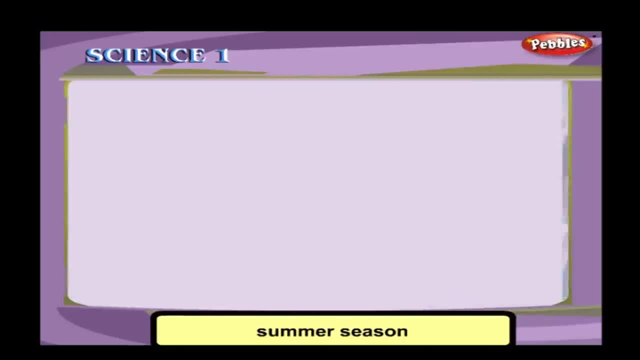 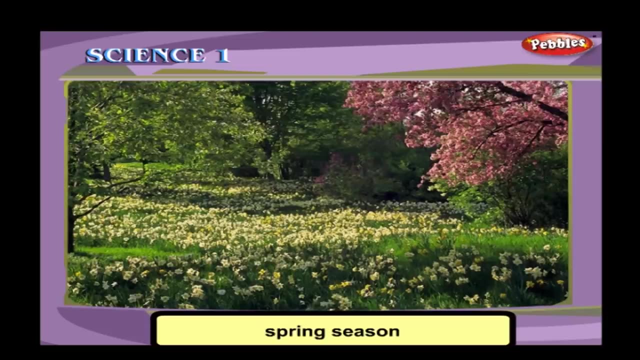 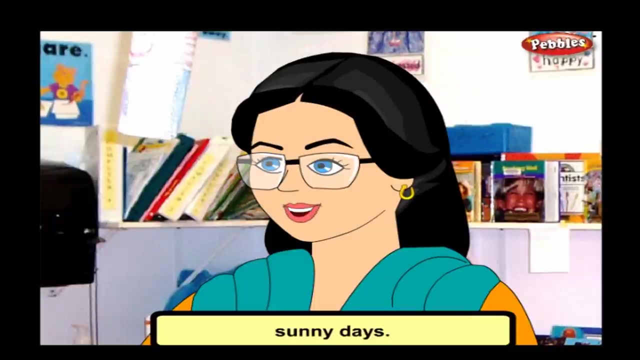 it is said to be a season. There are five main seasons in India. They are the summer season, rainy season, winter season, spring season and autumn season. First, I will tell you about the sunny days. The sun shines brightly on a sunny day. 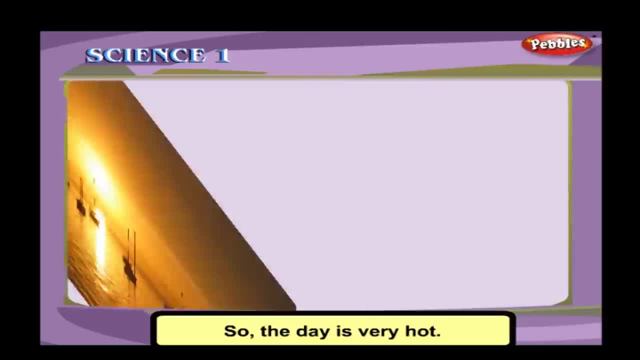 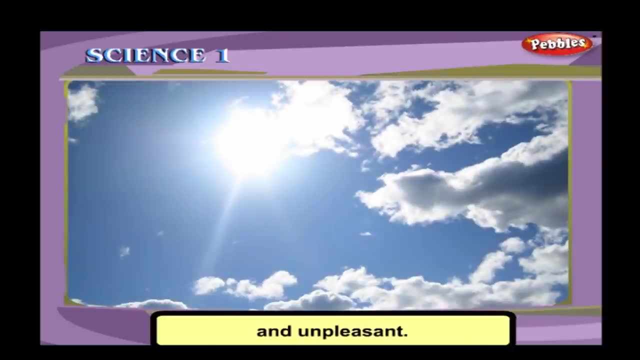 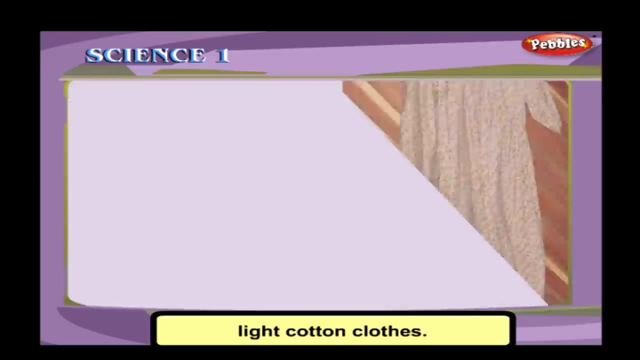 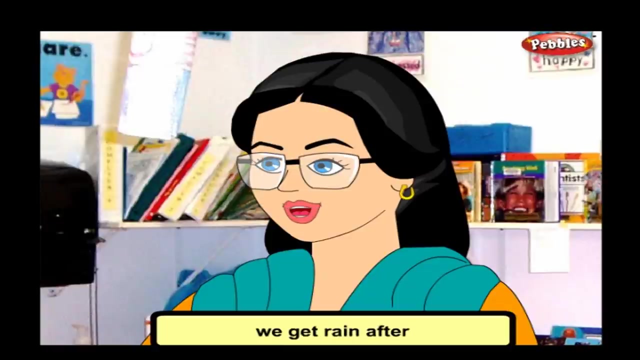 So the day is very hot. In summer the days are mostly sunny. The weather becomes hot and unpleasant. In this time we prefer to wear light cotton clothes. The weather becomes cooler on a rainy day. Sometimes we get rain after the hot summer days. 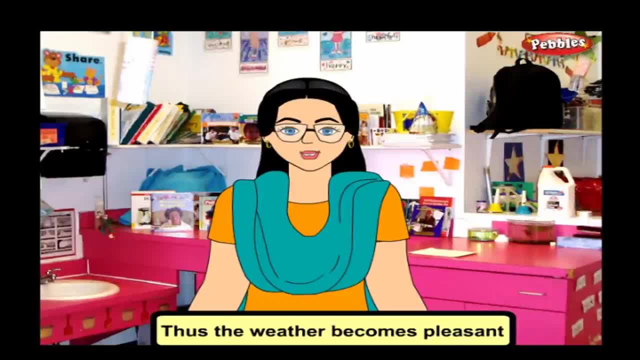 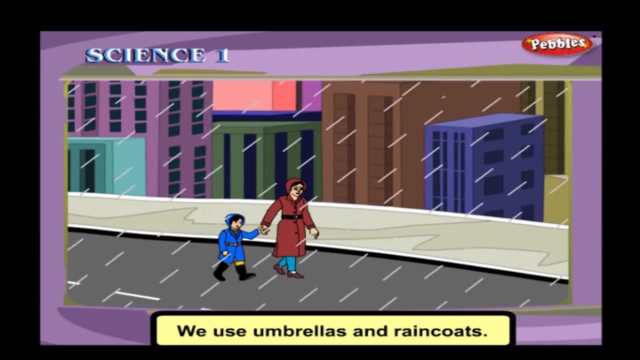 Thus the weather becomes pleasant. The rain in the winter makes the weather very cold and cold. The rain in the winter makes the weather very cold and cold. We use umbrellas and rain coats. They protect us from getting wet. We use umbrellas and rain coats. 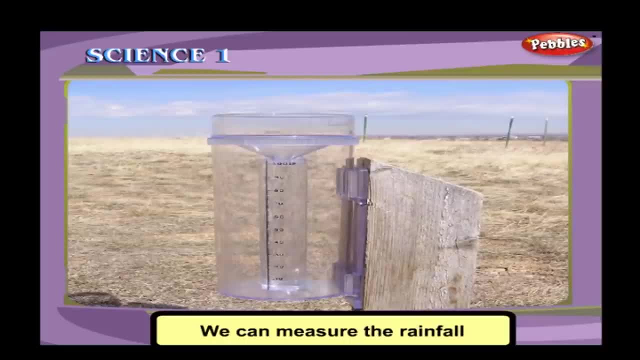 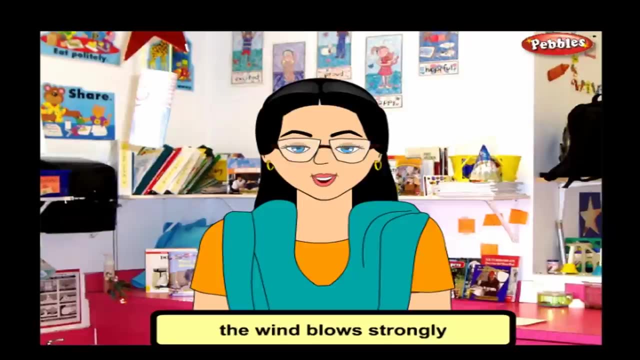 They protect us from getting wet. We can measure the rainfall by using the rain gauge. We can measure the rainfall by using the rain gauge. On some days the wind blows strongly. We call it a windy day. We can see many things flying in the wind. 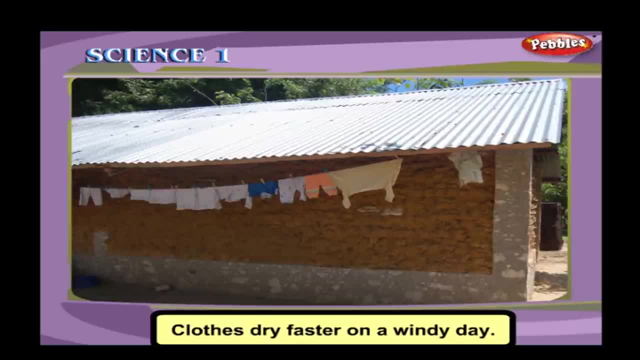 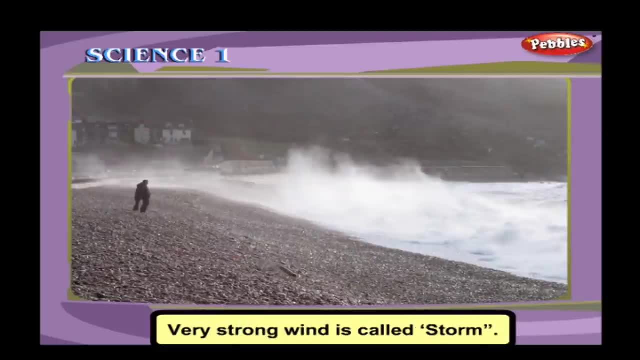 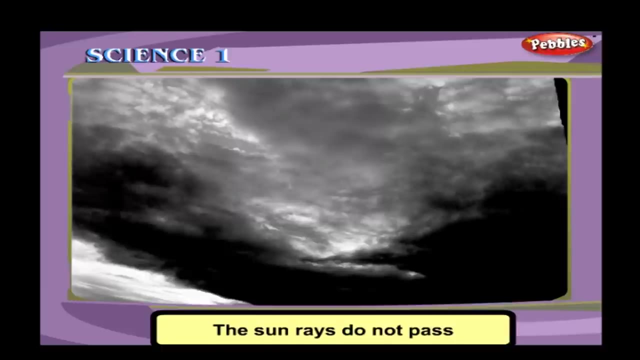 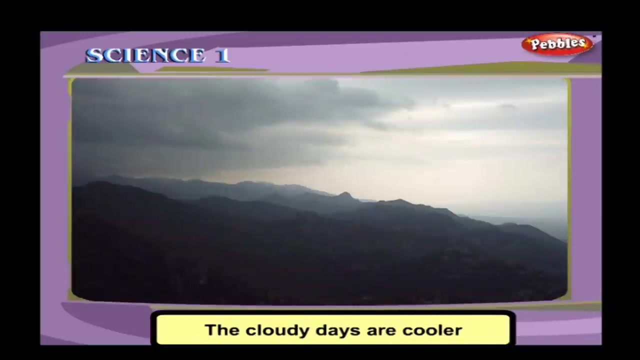 Clothes dry faster. on a windy day, children enjoy flying kites. very strong wind is called storm. we see clouds in the sky on a cloudy day. the sun rays do not pass through the clouds, so the weather becomes cooler. the cloudy days are cooler than the sunny days in winter. 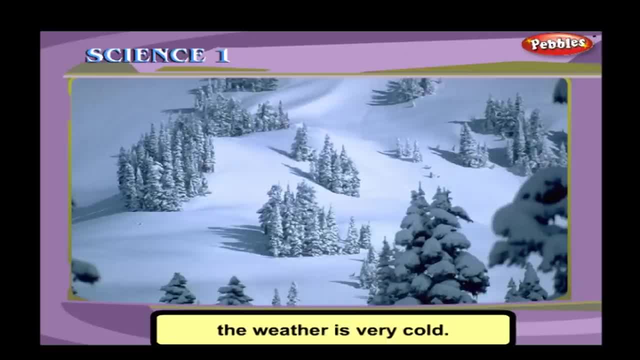 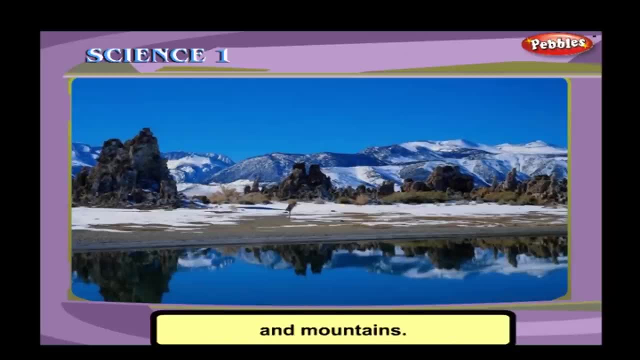 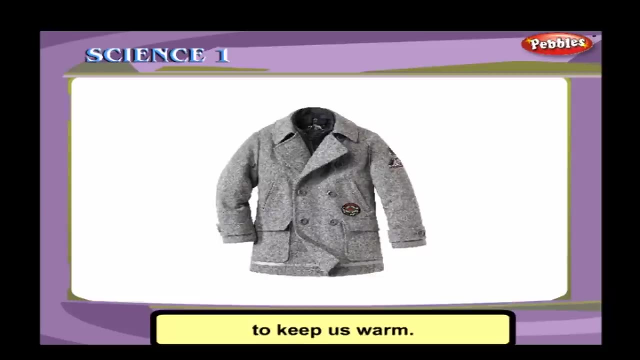 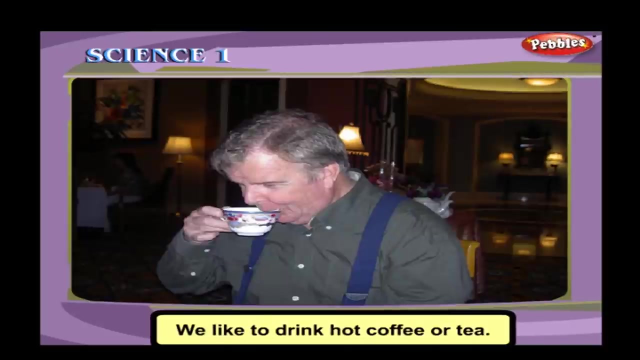 the weather is very cold. when it is very cold, snow falls on the high hills and mountains. on cold days, we wear woolen clothes to keep us warm. we use fire or a heater to protect us from the cold. we like to drink hot coffee or tea in cold countries. the weather is very cold, but the weather is very cold, so we 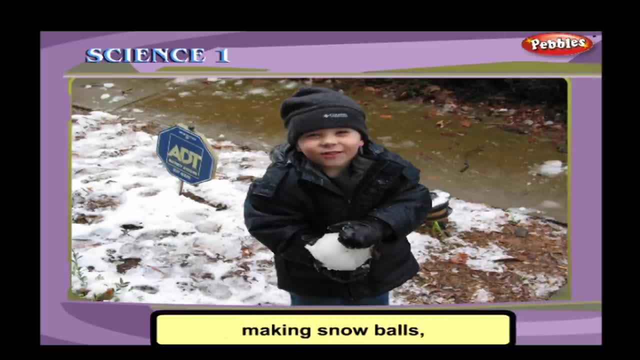 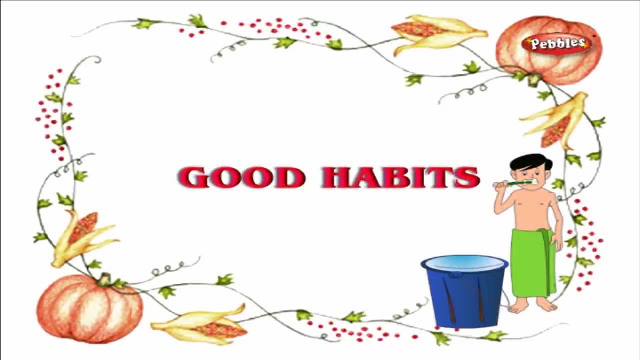 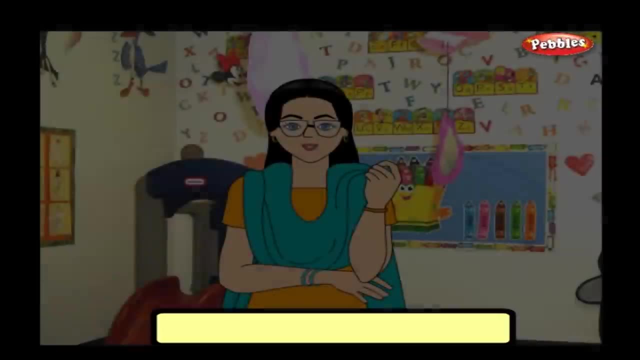 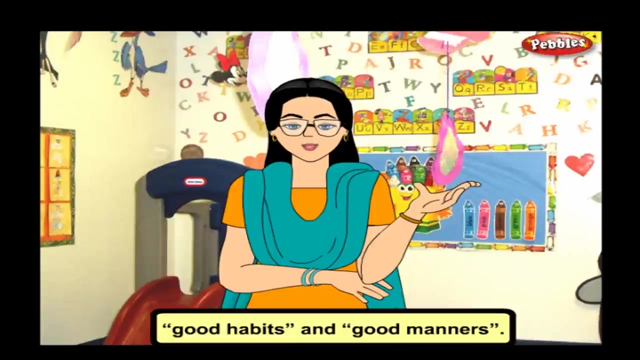 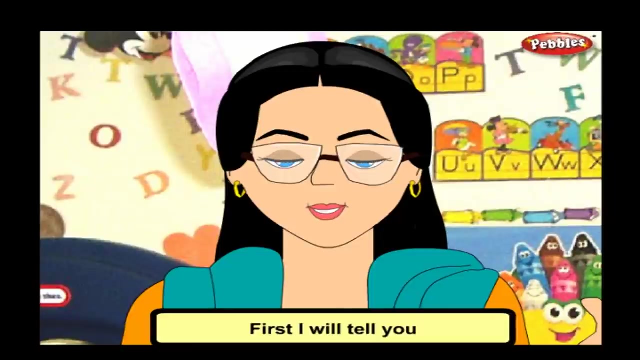 we like to drink hot coffee or tea. in winter, children play with snow, making snowballs. people go for ice skating. let us now discuss about good habits and good manners. good habits makes the person healthy and happy. first, I will tell you what you should do before and after eating: wash your hands. 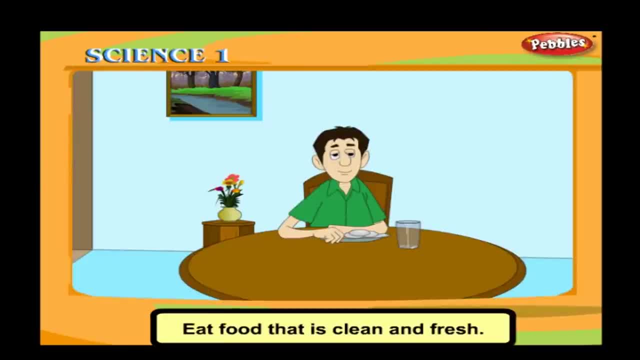 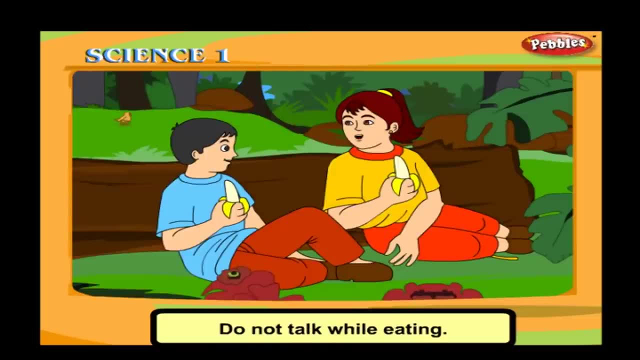 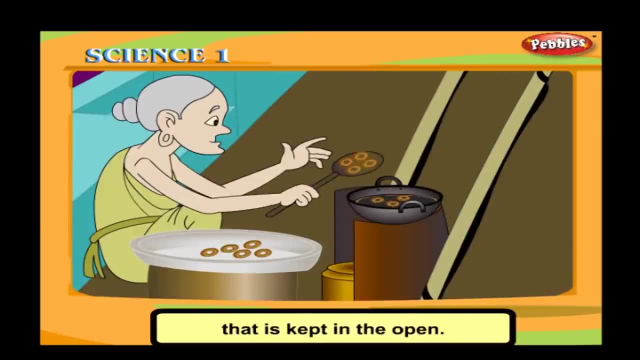 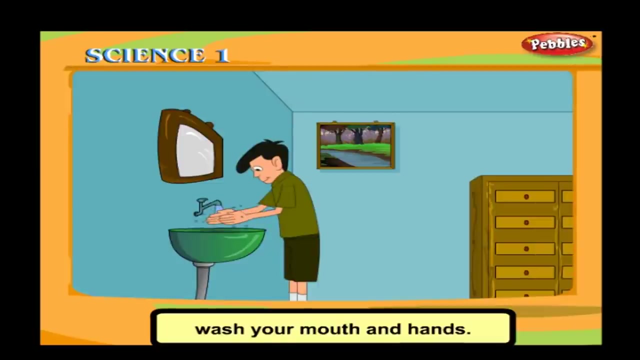 before eating food. eat food that is clean and fresh. do not eat too much food. do not talk while eating. do not eat food that is kept in the open. chew your food well. don't waste your food after the meal. wash your mouth and hands. dry your hand with a clean hand. 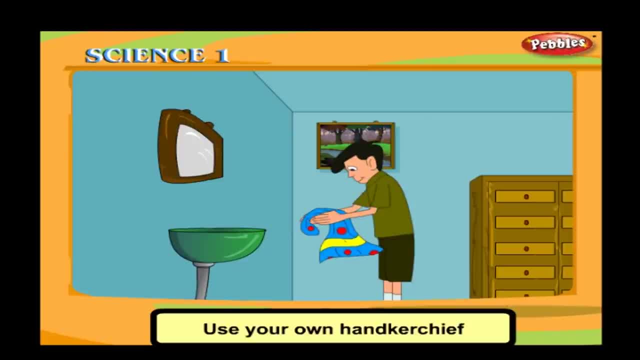 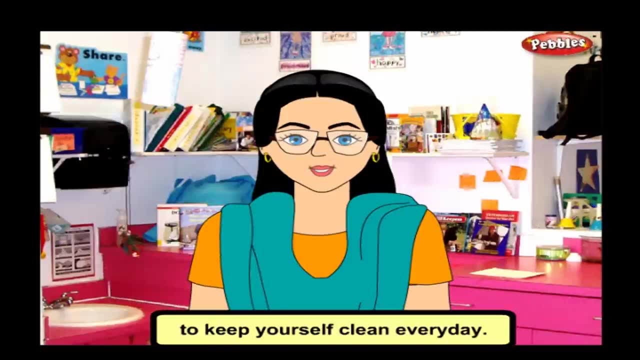 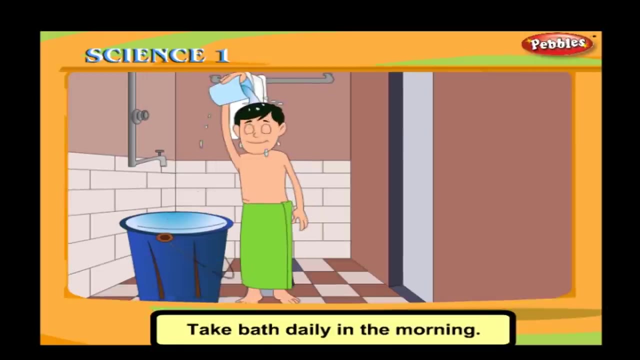 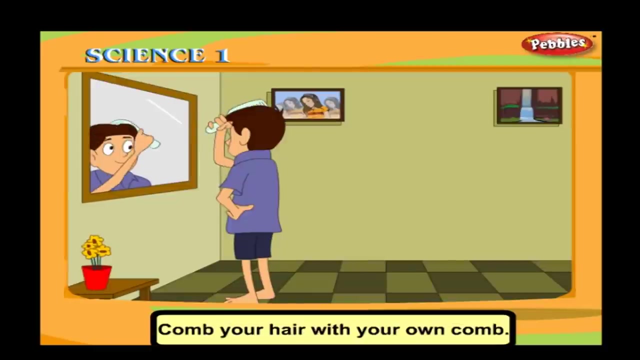 handkerchief or a towel. use your own handkerchief. now I will tell you some tips to keep yourself clean every day. brush your teeth every morning. take bath daily in the morning. wash your legs while coming out of a toilet. comb your hair with your own comb. wear clean and tidy uniforms and clothes. keep. 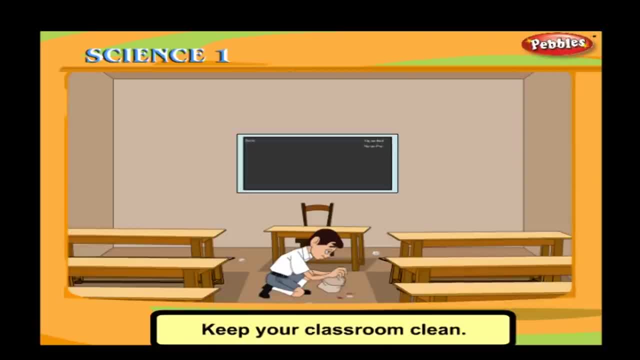 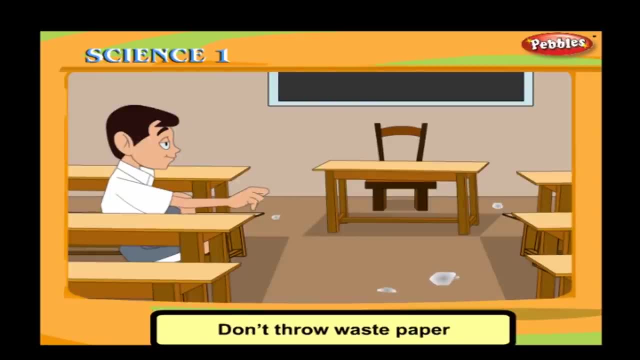 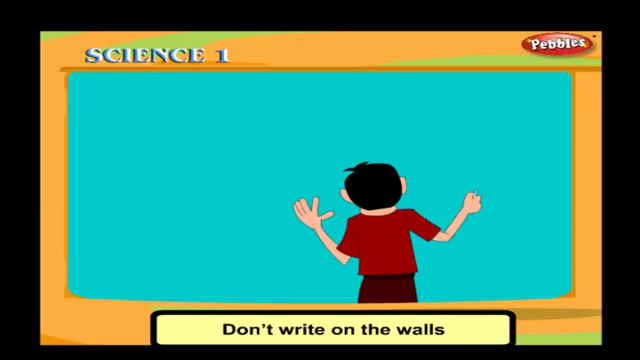 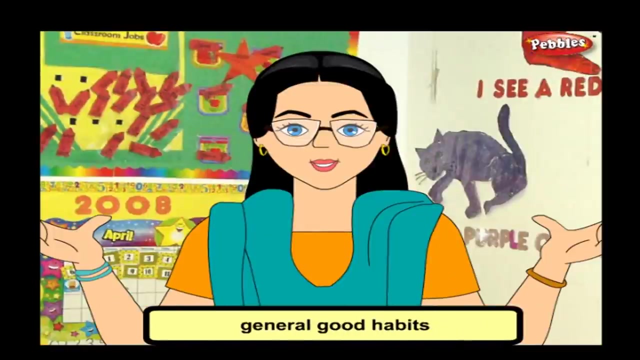 your home clean and tidy. keep your classroom clean. don't bite your nails. don't throw waste paper everywhere. put the waste paper into the dustbin. don't write on the walls or on the floors. don't write on the walls or on the floors. next I will tell you about some general good habits that children should follow. 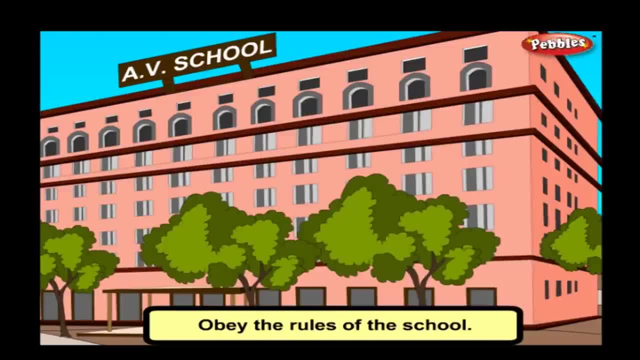 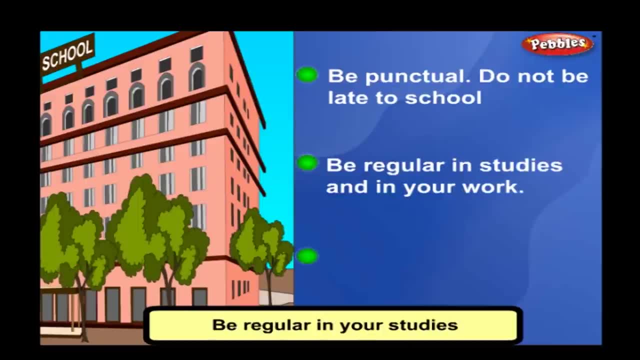 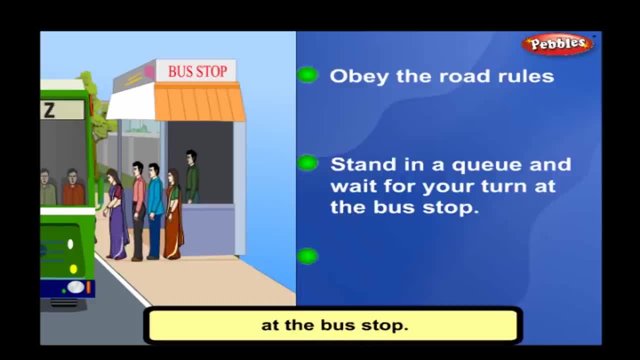 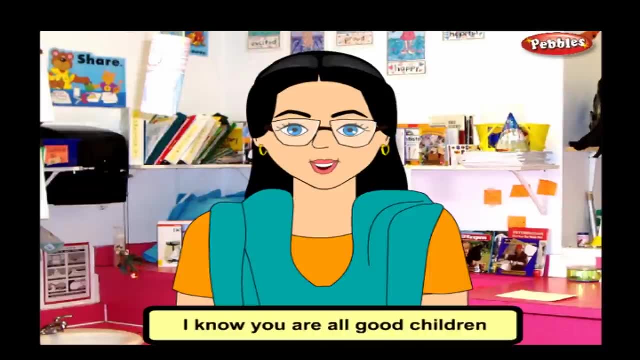 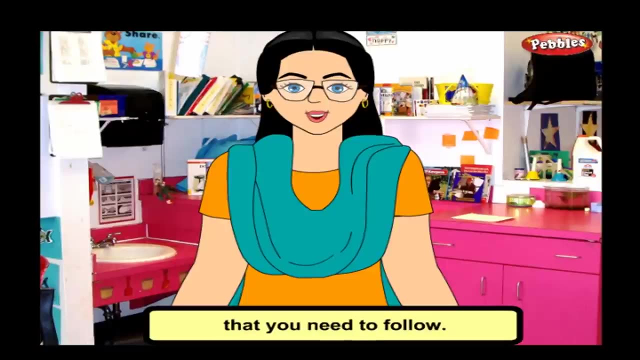 homework, do your homework, stand in a queue and wait for your tilt at the bus stop? children with good manners will be loved by all. I know you are all good children, but yet let me tell you some good manners that you need to follow. obey your parents, teachers and elders. respect. 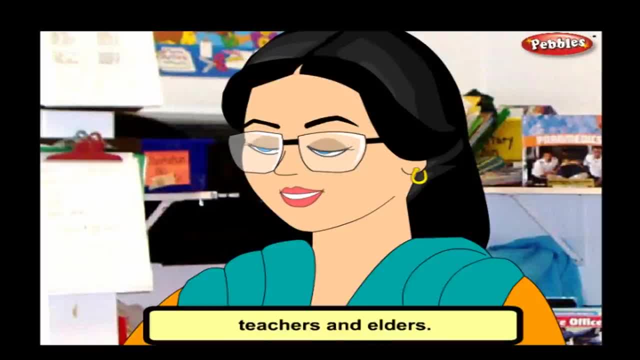 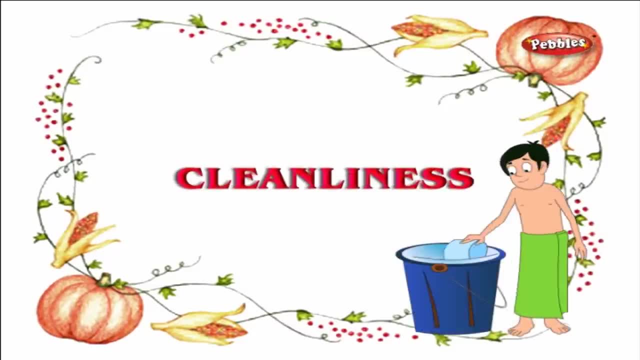 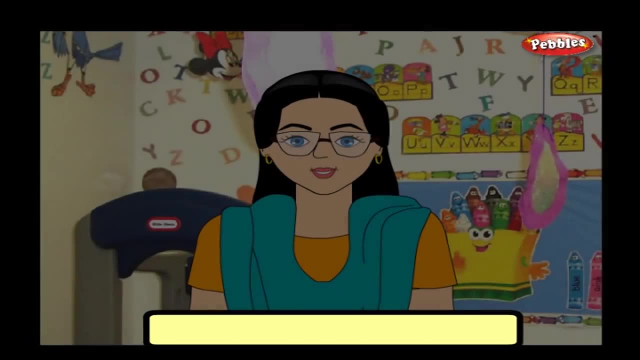 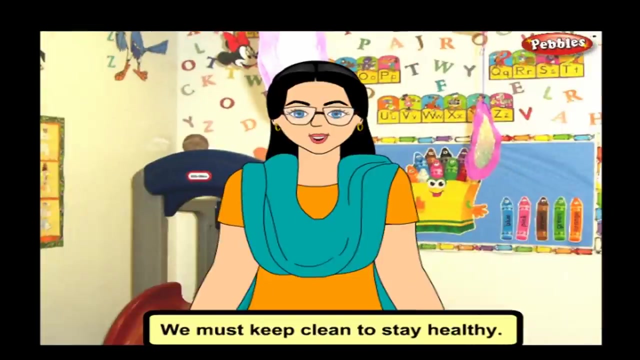 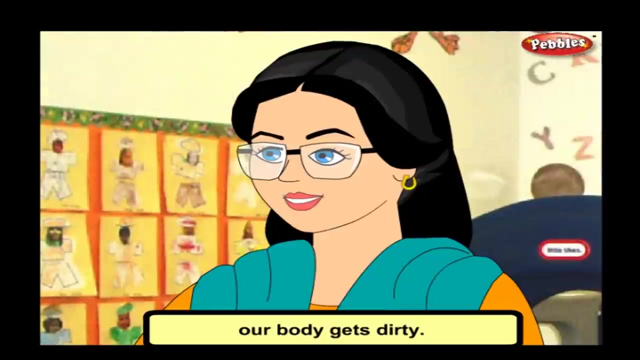 your parents, teachers and elders say sorry when you are rude. your teacher and family, your teachers and elders respect your parents, teachers and elders say sorry when you are, you hurt somebody by mistake. now I am going to tell you about cleanliness. we must keep clean to stay healthy. when we play or work, our body gets dirty. dust makes our body dirty. 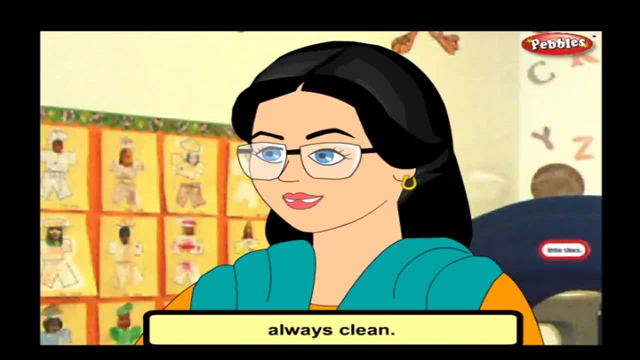 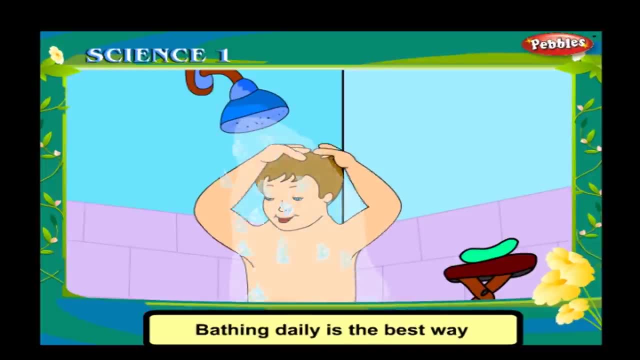 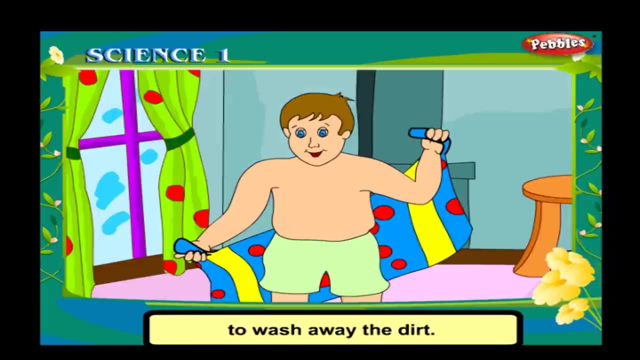 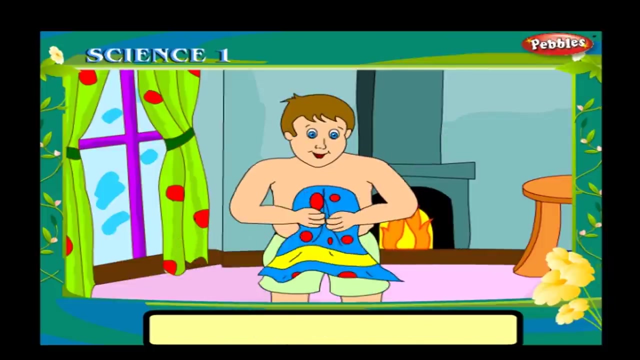 so we must keep our body always clean. how can we keep our body clean? bathing daily is the best way to keep our body clean. use soap and water to wash away the dirt. dry your body using a clean towel. wear clean clothes every day after the bath. cut your nails regularly and keep them. 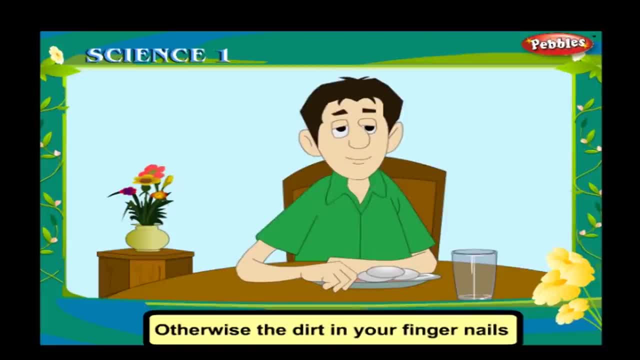 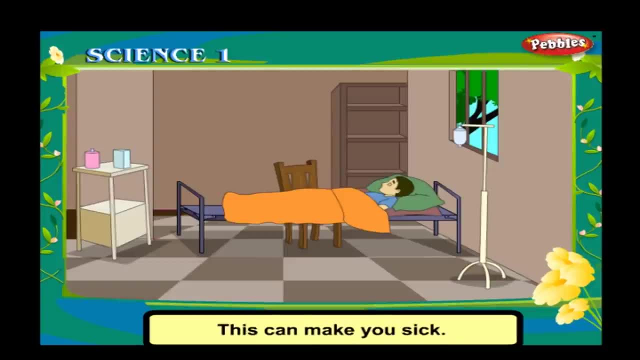 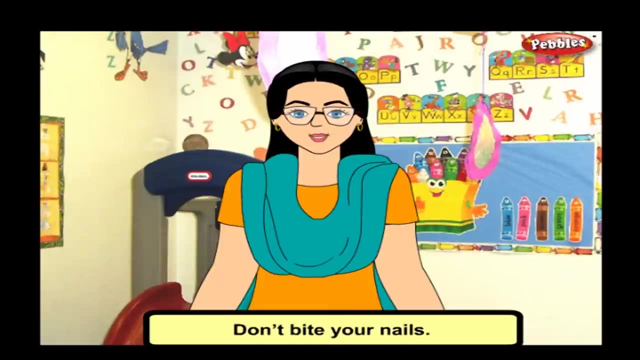 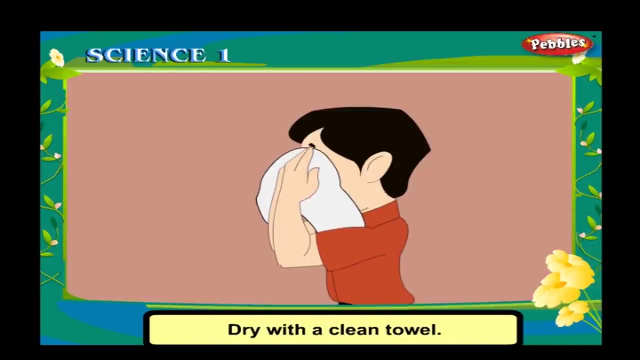 clean, otherwise the dirt in your fingernails will enter your body along with the food you eat. this can make you sick, so your nails must be trimmed and kept clean. don't bite your nails. wash your face with soap and water, dry with a clean towel. try to keep your face bright and clean so that your face looks nice. 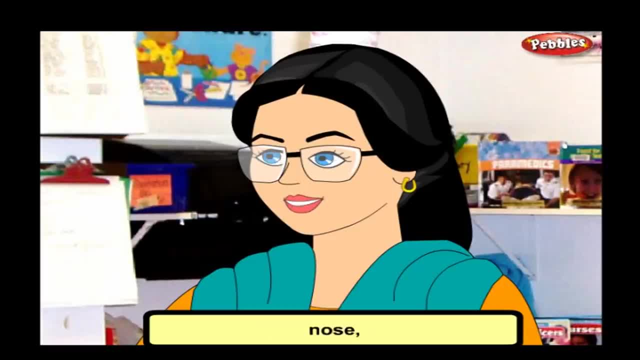 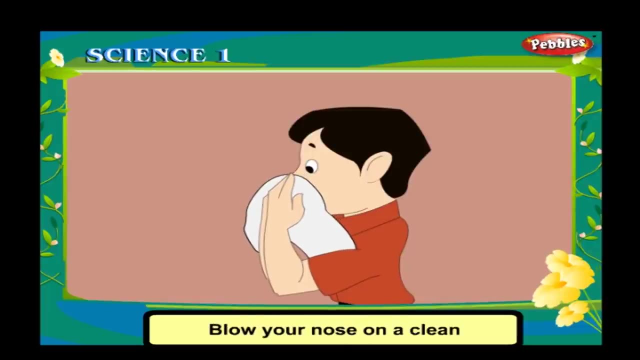 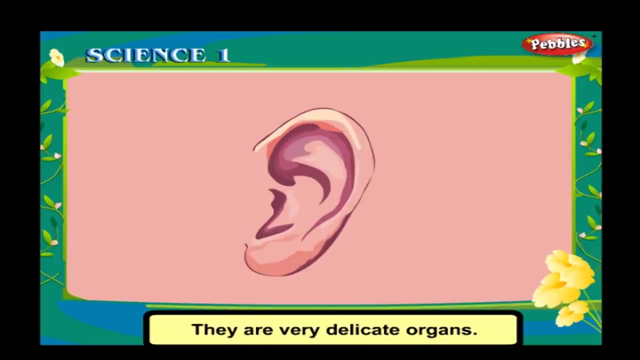 clean your eyes, nose- yes, teeth- and hair regularly. how to keep your nose clean? we breathe and smell with our nose. blow your nose on a clean handkerchief. do not clean your nose with your fingers. it is a bad habit. next comes years. we hear with our ears. they are very delicate organs. we must take care of them. use a clean. 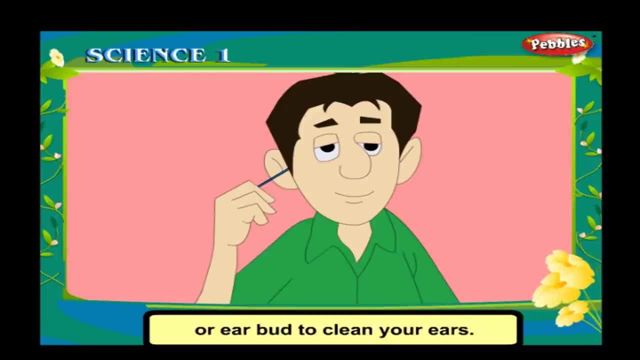 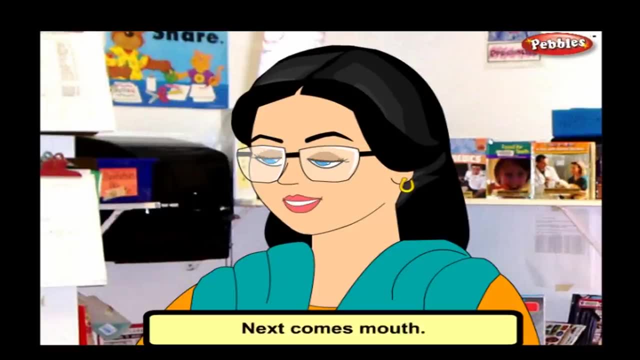 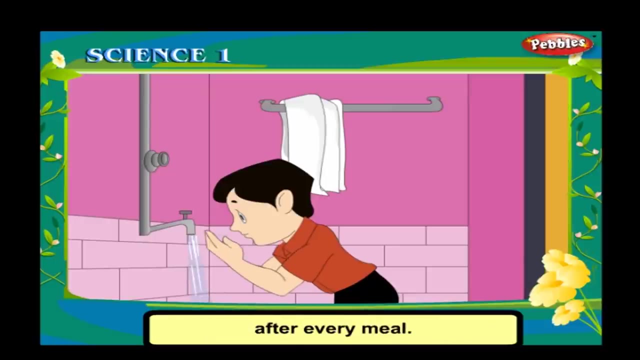 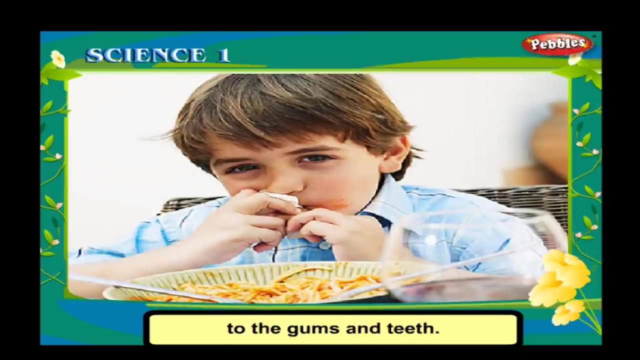 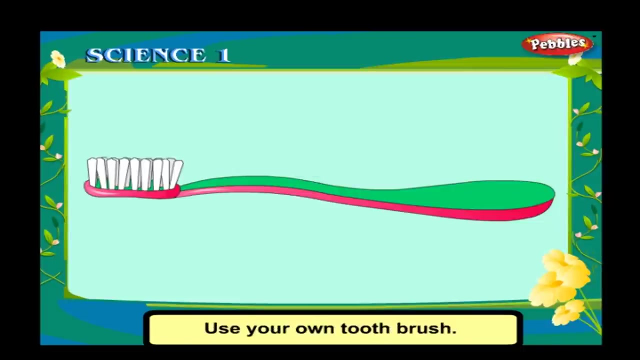 wet towel or ear bud to clean your ears. you should not put anything into your ear. next comes mouth. we speak and eat with our mouth. rinse your mouth with water after every meal. then comes teeth: when we eat, the food particles stick to the gums and teeth. it causes tooth decay and diseases. use your own toothbrush. 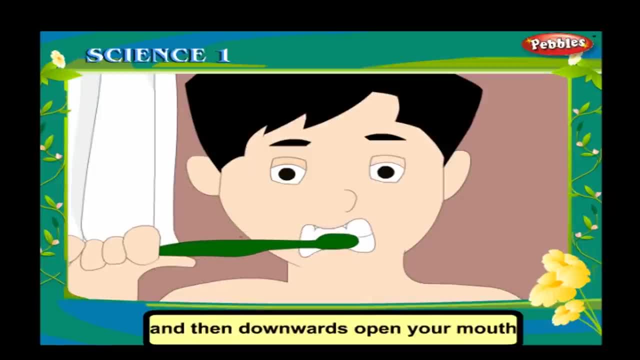 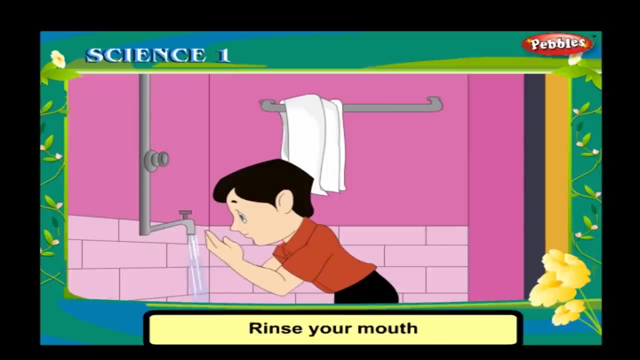 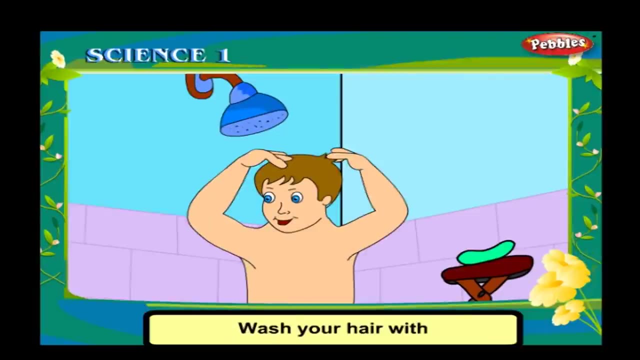 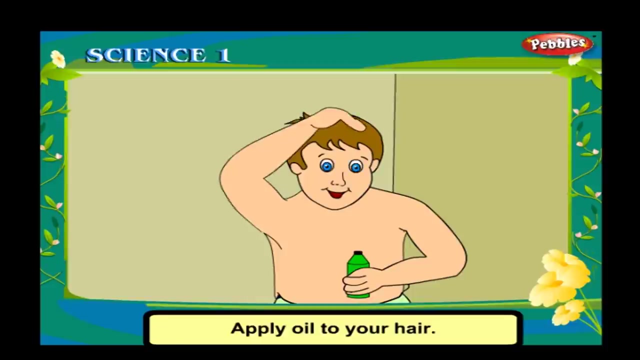 brush your teeth upwards and then downwards. open your mouth and brush from inside. rinse your mouth several times with water, water. finally, we will see about your hair. wash your hair with shikakai or shampoo. dry with a clean towel, apply oil to your hair. comb your hair. 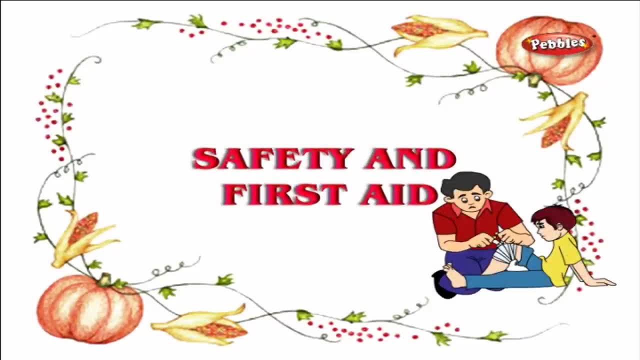 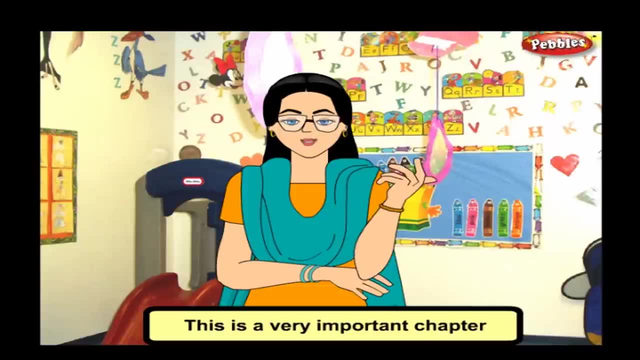 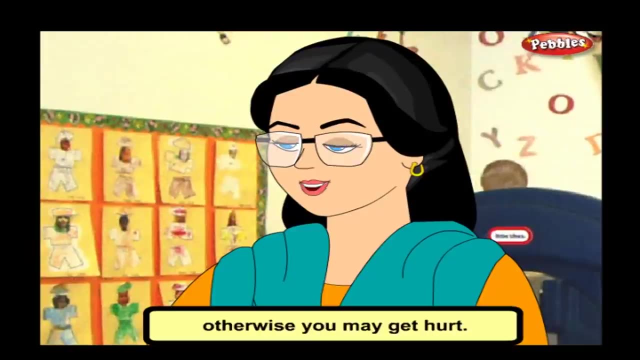 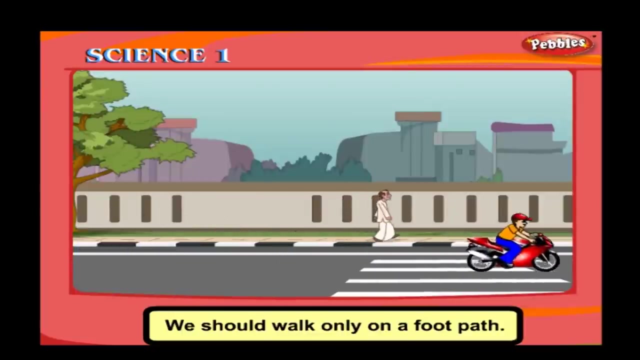 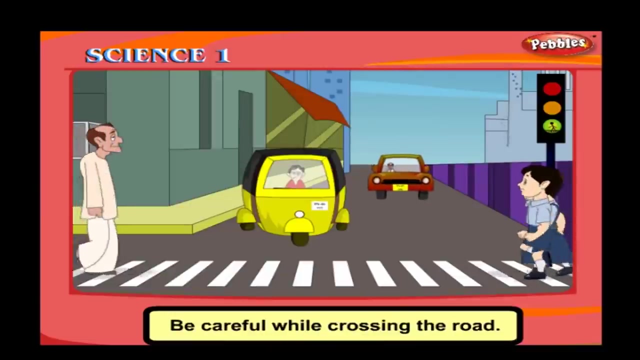 this is a very important chapter for small children. you have to be very careful all the time, otherwise you may get hurt. first comes road safety. we should walk only on a footpath. if there is no footpath, walk on the safe side side of the road. do not run on the road. you may slip and get hurt. be careful. 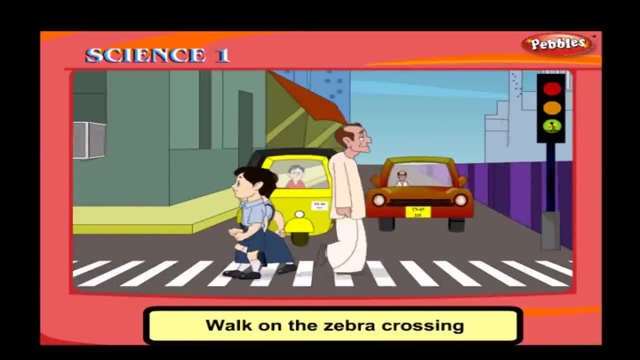 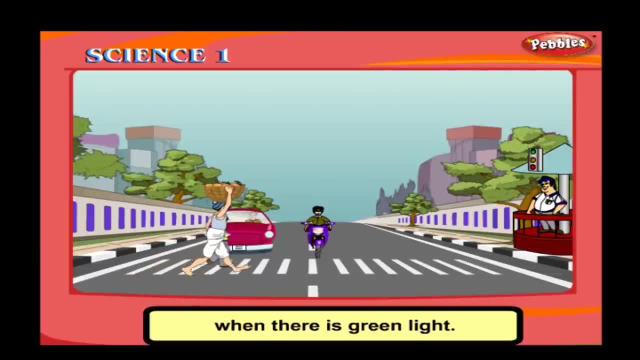 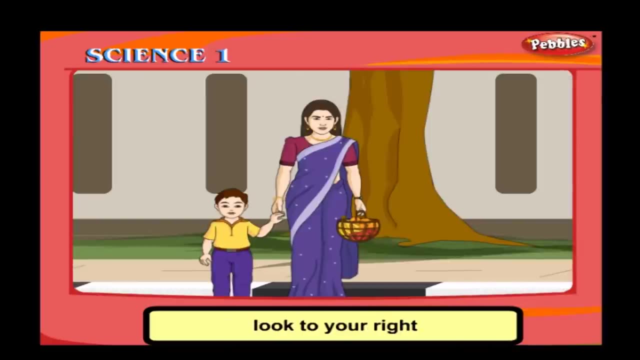 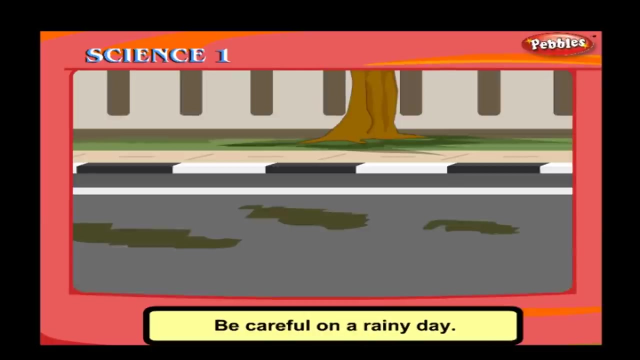 while crossing the road. walk on the zebra crossing. look at the traffic lights. cross the road only when there is green light. stop when there is red if there is no zebra crossing. look to your right now. look to your left. look to your right again. cross the road only when it is clear. be careful on a rainy day. the 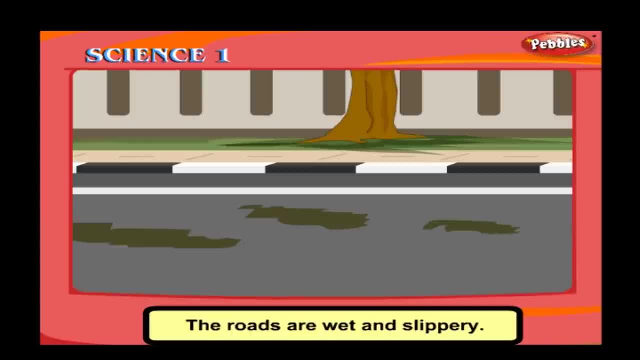 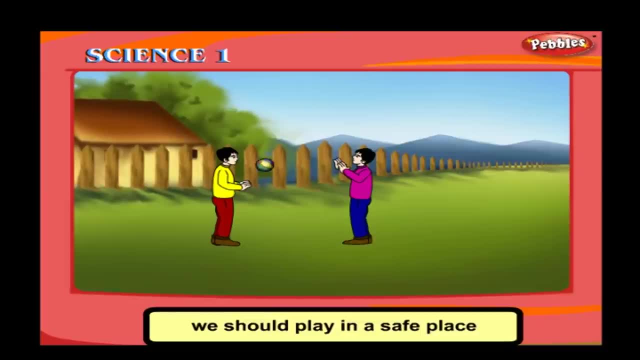 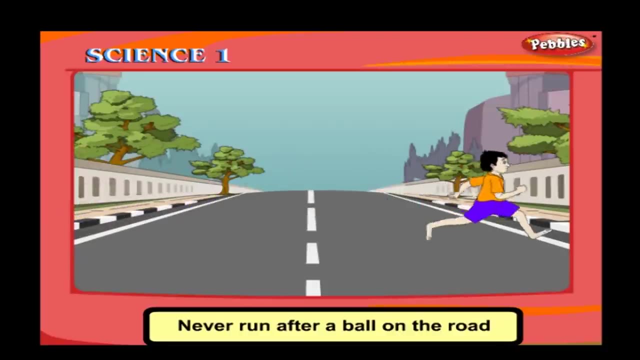 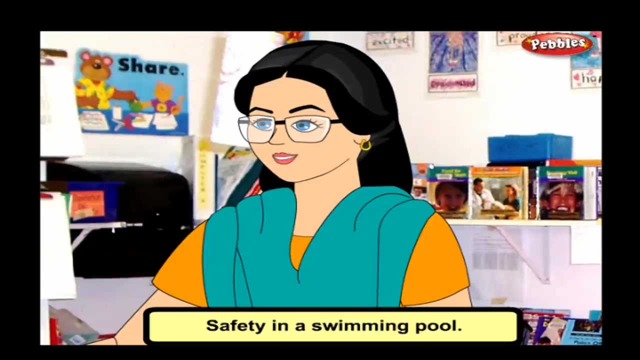 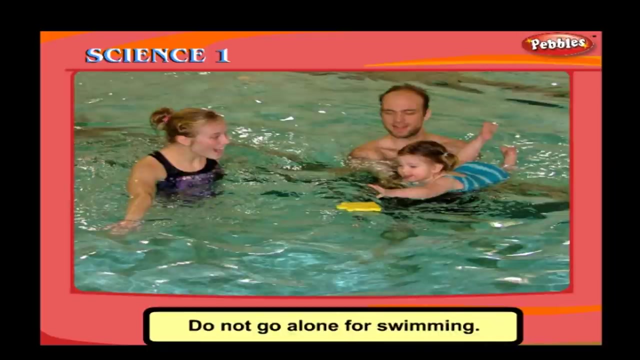 roads are wet and slippery. safety while playing. when we play, we should play in a safe place. it is not safe to play on the road. never run after a ball on the road. playing kites on rooftops or roadside is dangerous. safety in a swimming pool: swimming is a very good exercise. do not go alone for swimming if you cannot swim. 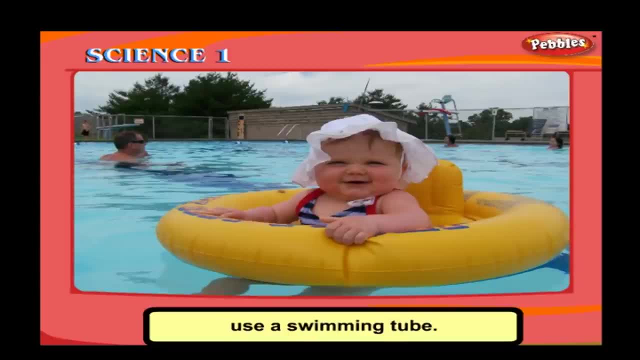 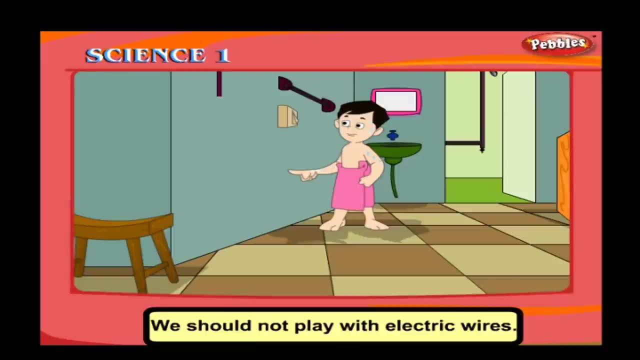 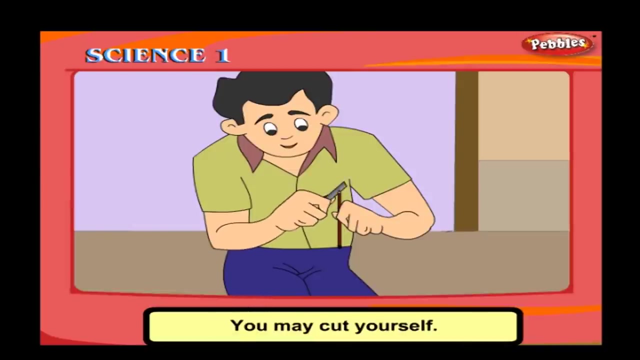 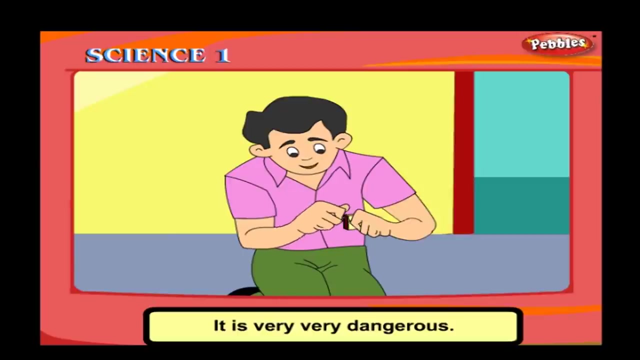 well. use a swimming tube. do not go into deep water. never play in water. we should not play with electric wires. you may get an electric shock. be careful and be safe. be careful when you handle sharp things. you may cut yourself. don't play with fire. it is very, very dangerous, even though we 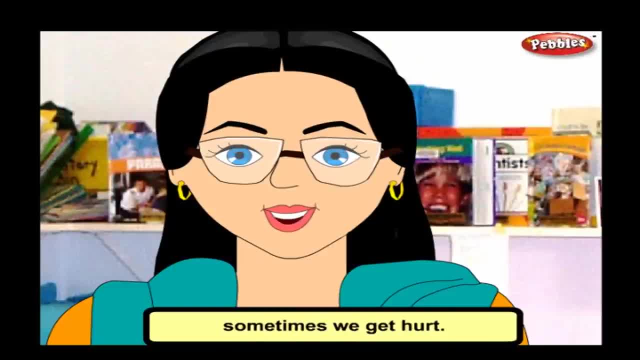 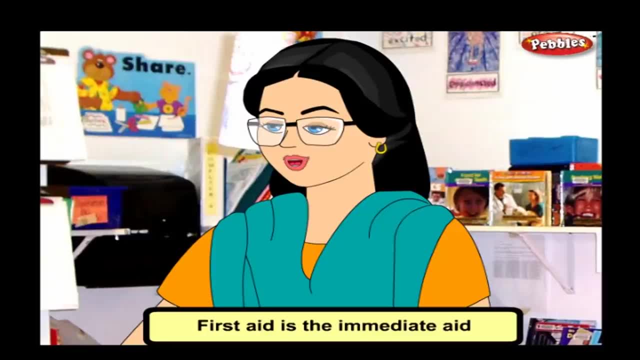 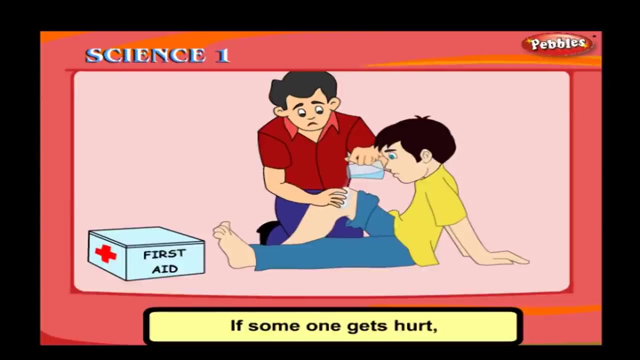 follow all the safety measures. Sometimes we get hurt. Now it is time for first aid. First aid is the immediate aid which we do when we get hurt. The first aid box will contain band-aid medicines, etc. If someone gets hurt, do not run away. 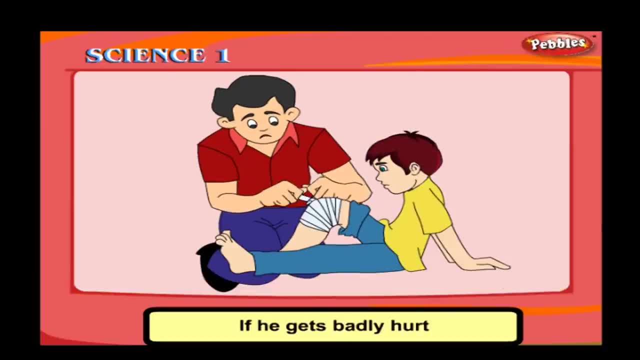 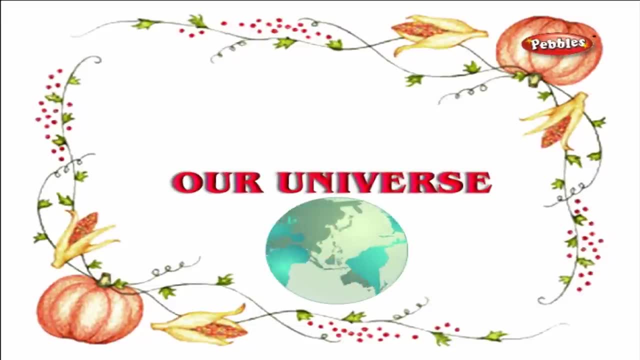 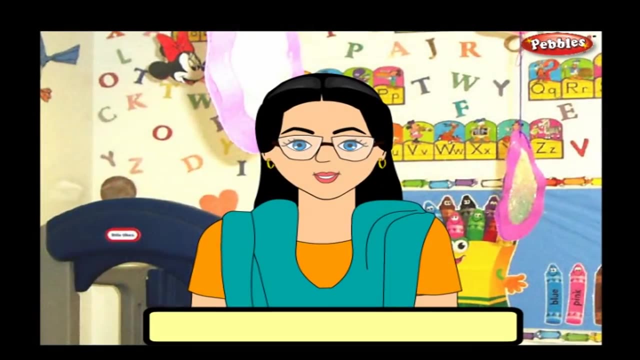 Help him, Give him first aid. If he gets badly hurt, then send for a doctor. Children, now tell me what are the things that you see on the sky, both in the day and night. We can see sun in the day time. 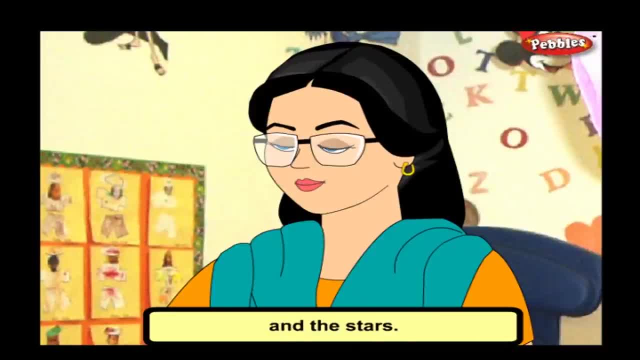 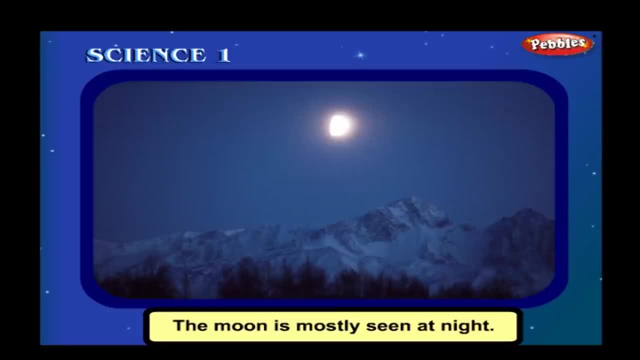 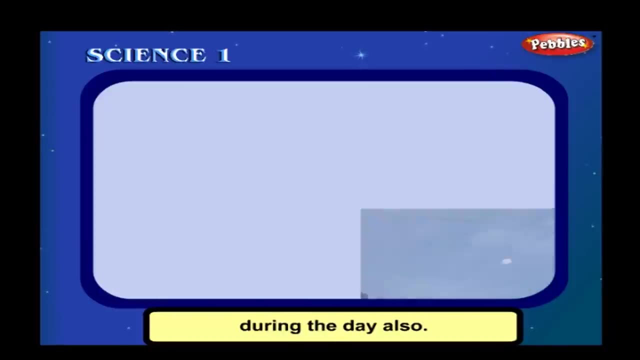 And at night you can see the moon and the sun. The sun shines in the sky during the day. The moon is mostly seen at night. At times we can see the moon during the day also. The stars twinkle in the sky only at night. 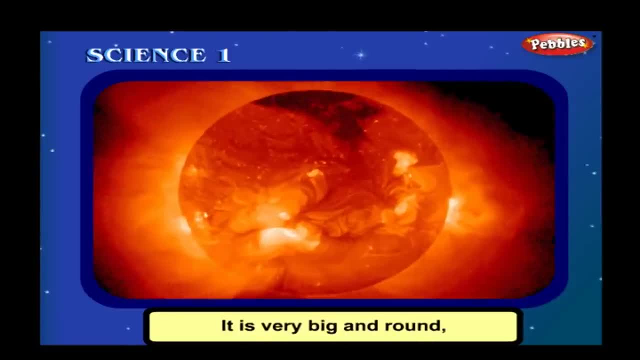 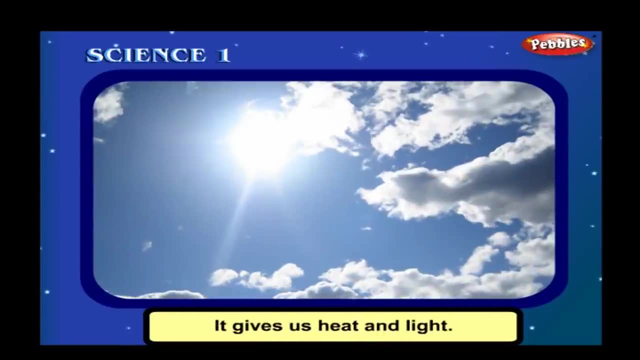 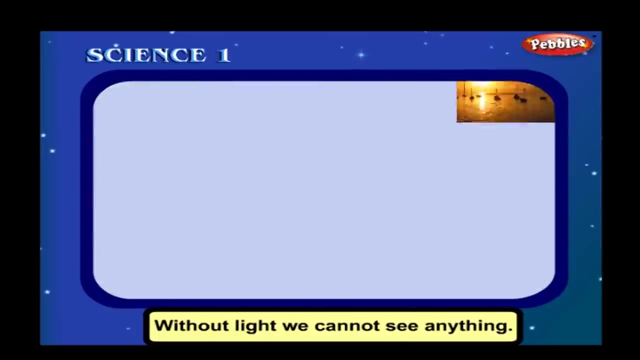 The sun is a hot ball of fire. It is very big and round And it is far away from us. It gives us heat and light. Without light we cannot see anything. The sun rises in the east, It rises in the morning. 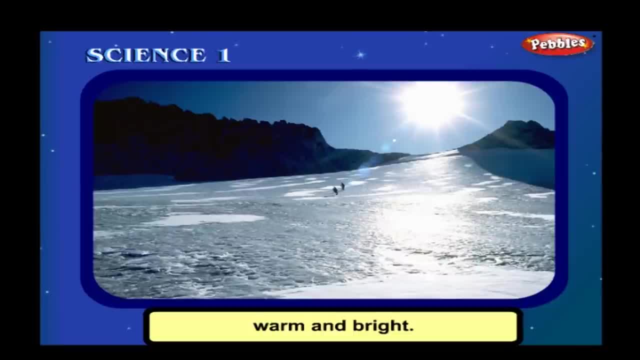 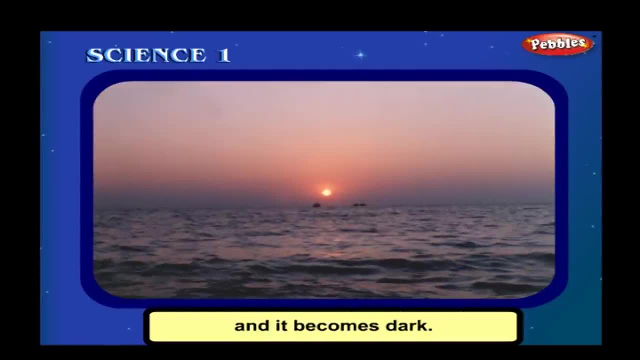 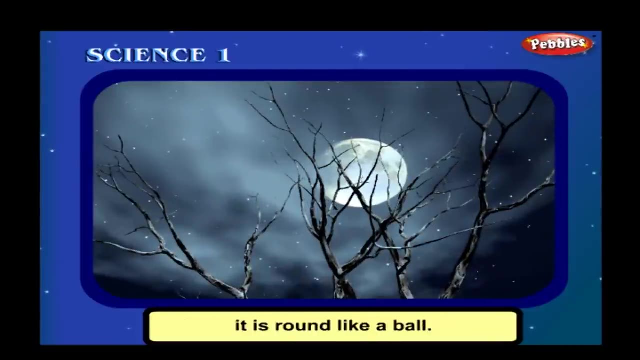 The light from the sun makes our days warm and bright. The sun sets in the west, It sets in the evening And it becomes dark. We see the moon at night. It is round like a ball. It is smaller than the sun.